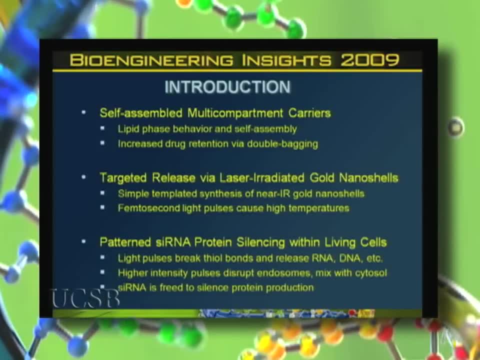 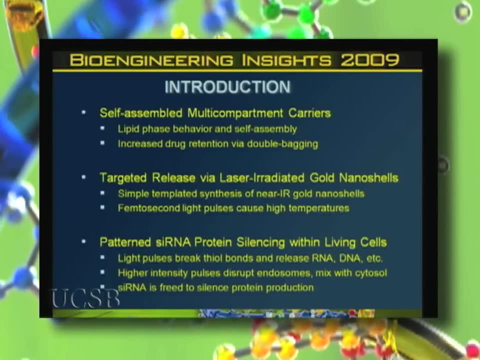 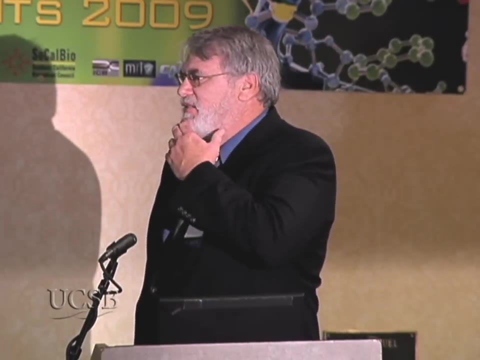 that we have created with a multiple nesting compartment. Basically, the technical idea is the same one you have at the grocery store. If one bag is good, double-bagging must be better, And so we'll tell you how to double-bag things at the nanoscale. 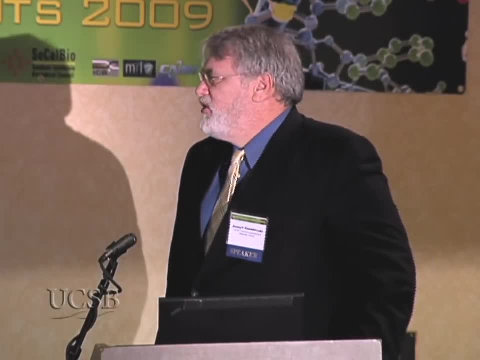 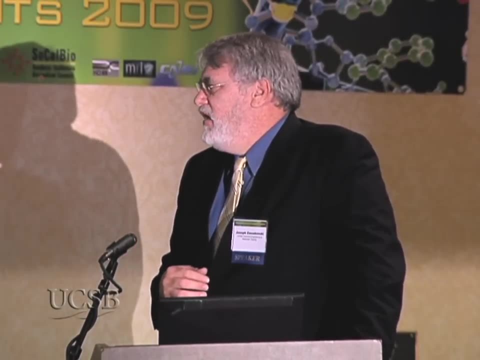 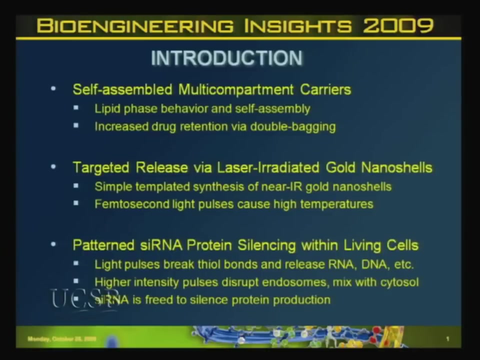 The second thing is a little bit more generic method of targeting and releasing contents, either from cells or from artificial cells, like the lipid carriers that I'm going to talk to you about, And we're going to do this by focusing laser light onto gold nanoshells. 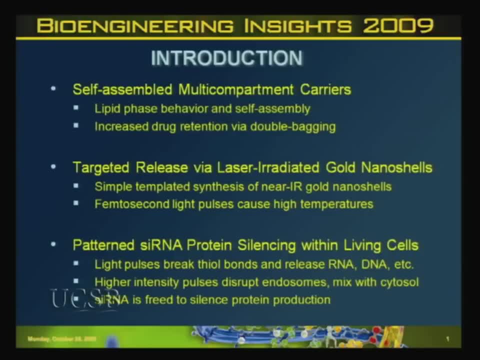 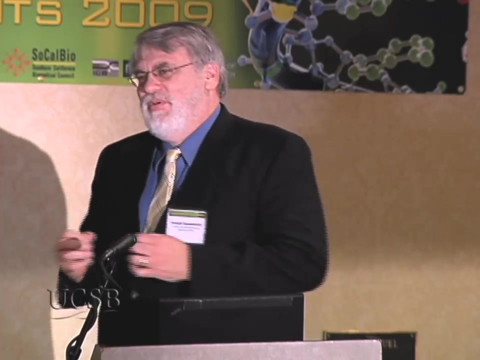 And the particular light we're going to use is in the near-infrared, which is where we all happen to be relatively transparent, so that we can get into our tissue without damaging. So we will talk about that. And then that's actually using this laser as kind of a bomb so that we can explode things. 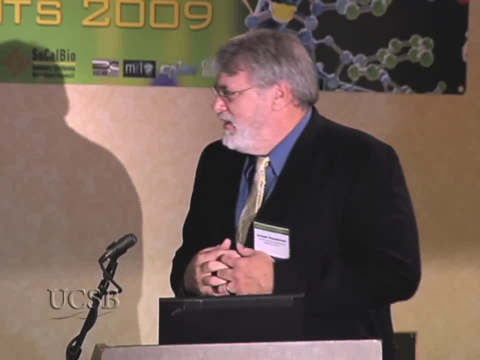 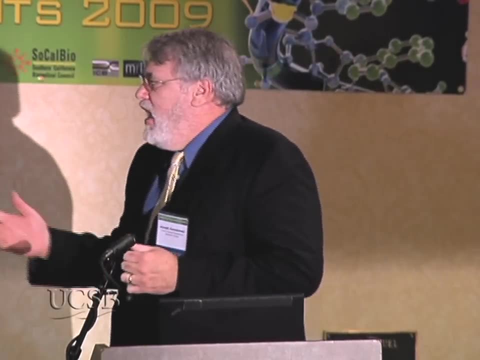 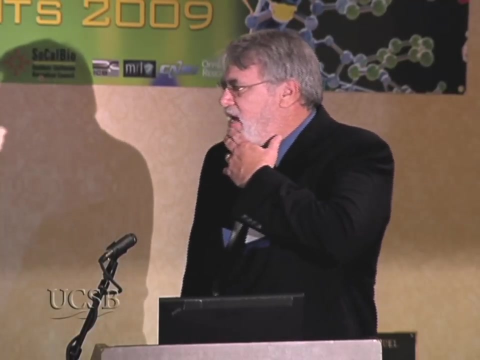 And of course that appealed to my 13-year-old boy inside, because everybody wants to blow stuff up when they're 13.. And then we're going to turn this light into a little bit more of a scalpel and actually show how this light can be used to pattern the delivery. 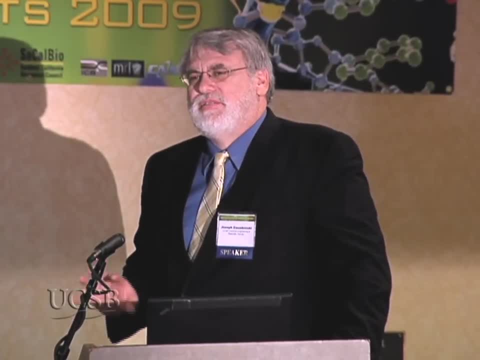 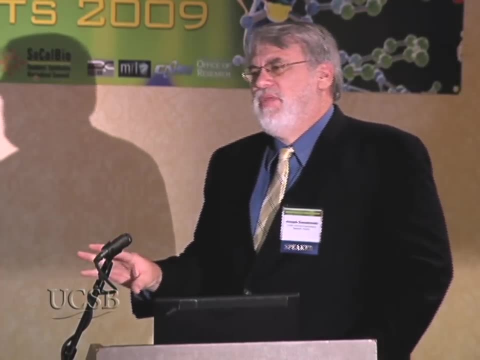 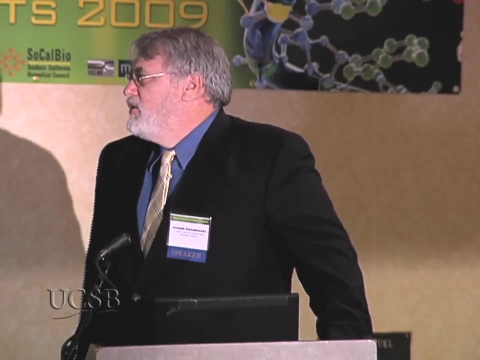 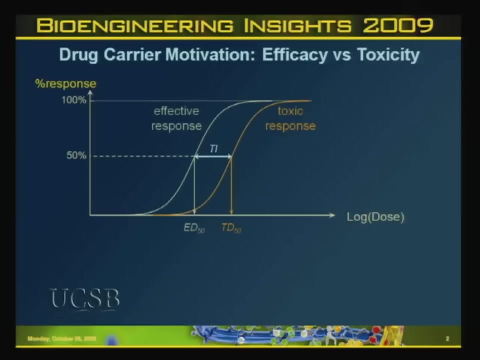 of genetic material into a cell And turn particular protein processes on and off in living cells- And not only living cells, but turn something on in this cell while leaving an adjacent cell unaffected. So our motivation is pretty simple. We're looking at the general problem of efficacy versus toxicity. 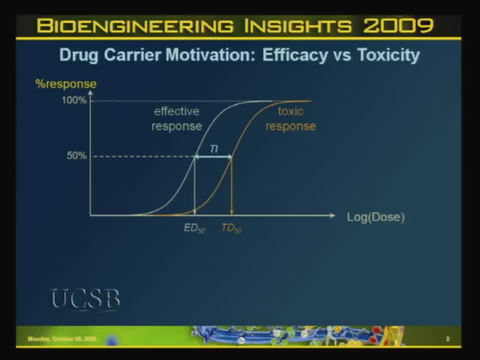 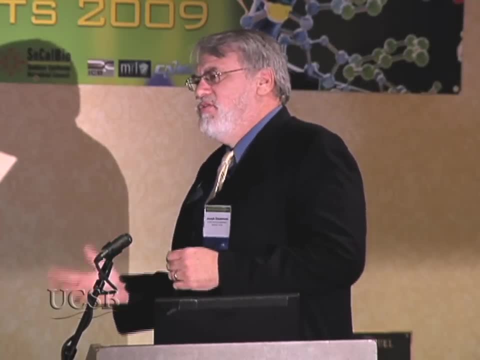 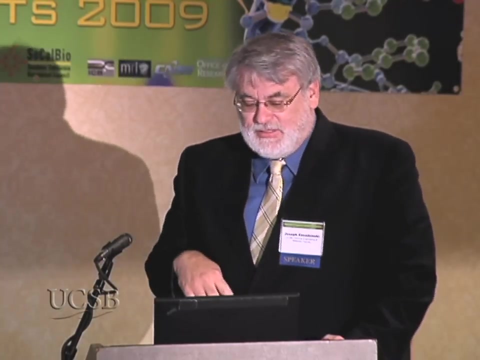 And basically any type of drug has needs a certain concentration to be effective, And almost all drugs, if you put too much in, have some sort of a toxic response. So what you'd like to do with a drug delivery system is to lower the effective dose that you need. 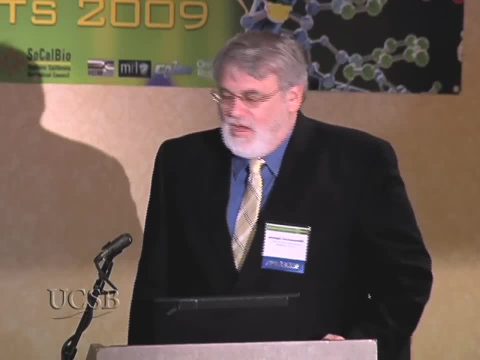 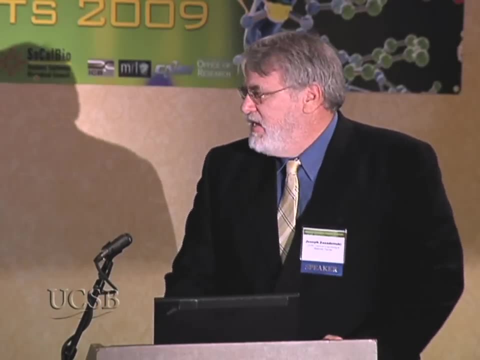 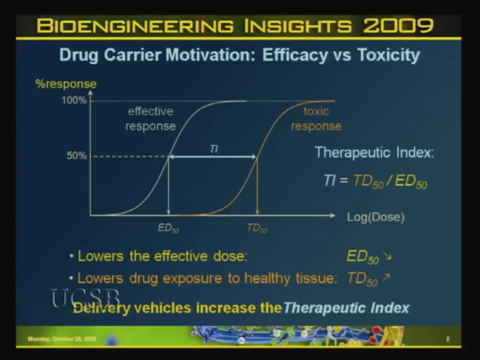 to introduce into the system while increasing the level of drug that gives you this toxicity, And that combination of things is what's called the therapeutic index. It's this ratio of the toxic dose to the effective dose, And so what a good delivery vehicle is going to do is going to deliver more drug to the side. 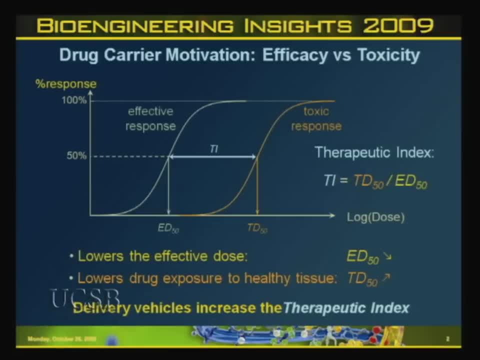 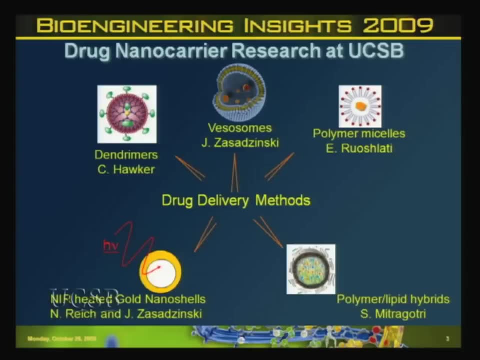 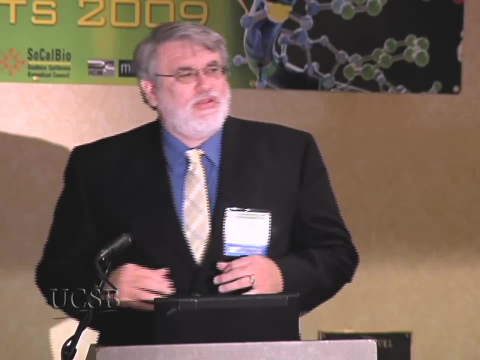 of interest so that you can do both things at the same time, And there's not going to be any one particular magic bullet that is going to be able to deliver any drug or any genetic material to any particular thing, And there's a number of different routes that are going on at UCSB. 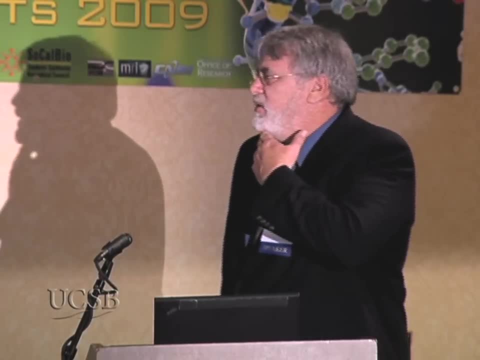 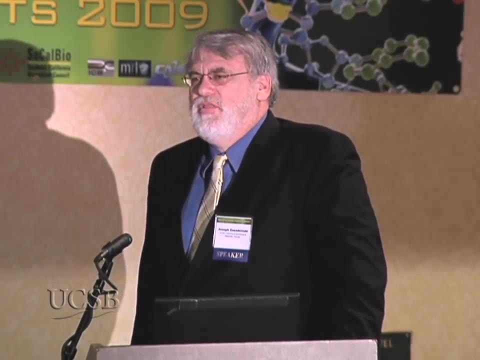 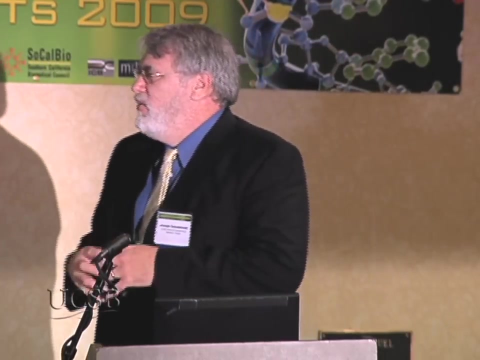 I'm going to talk to you first about a nested vesicle structure called the vesazome- And it's called the vesazome because all the good names were taken- And we are working on this as a way to extend the encapsulation program. 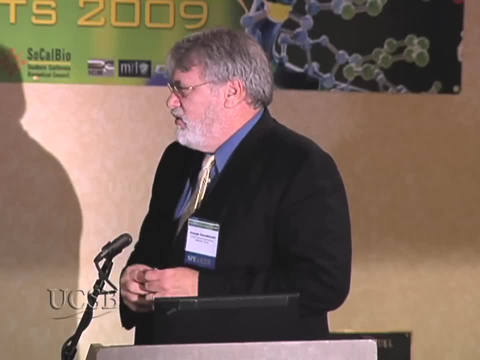 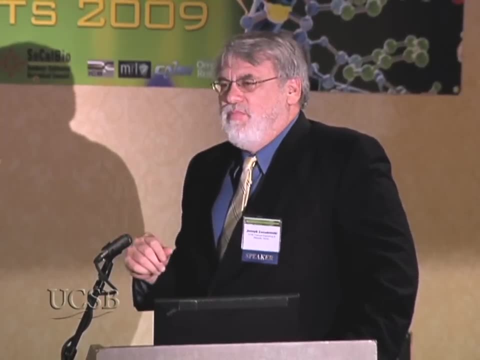 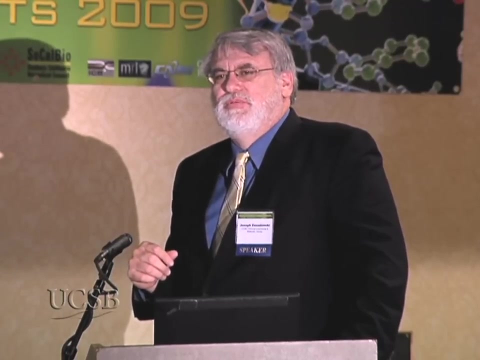 of drugs in the circulation. Dr Ruslati, whose name I spelled wrong- I put the H in the wrong spot- is working on polymeric micelles with a carrier and targeting agents to try to deliver material to specific cells. Craig Hawker of our Materials Research Lab. 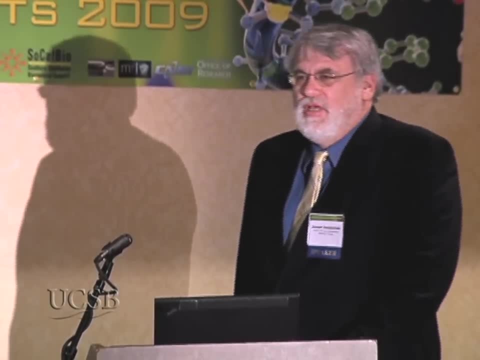 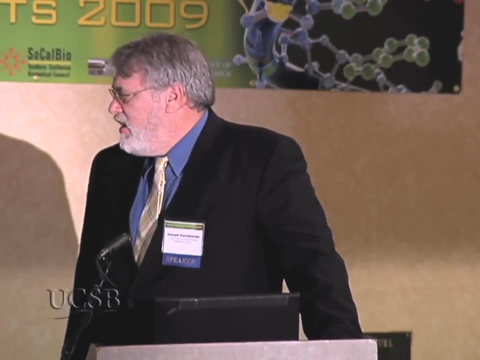 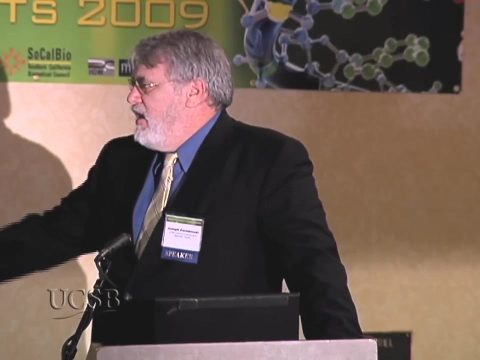 is creating polymer structures, dendromers and other types of polymers to deliver drugs. Samir Mitrogotri, our chair, has been developing polymer-lipid hybrids to try to mimic red blood cells, And I'll also tell you about gold nanoshells. 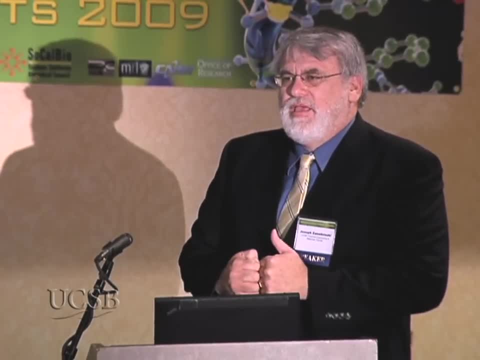 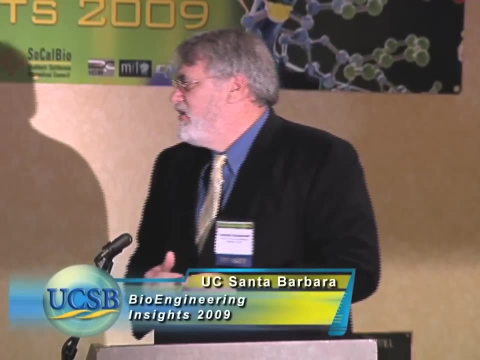 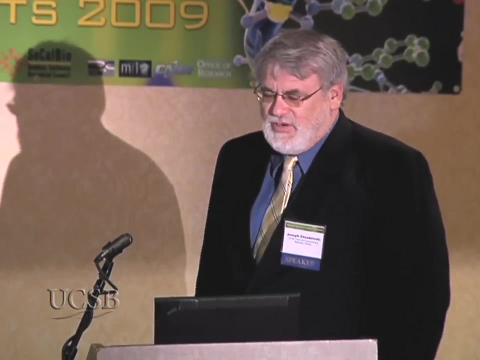 that are heated work I'm doing in collaboration with Norbert Reich of our chemistry department. So we can go anyway, and the main unifying characteristic of these things is that we are, at at least in some aspect of these structures at the nanoscale And we have to. 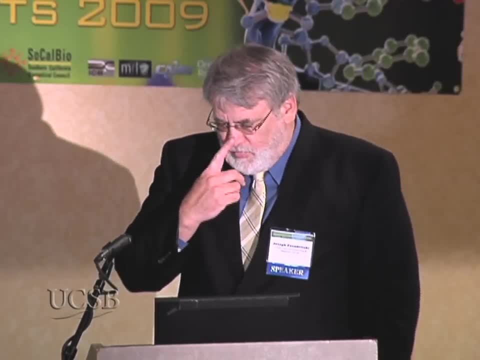 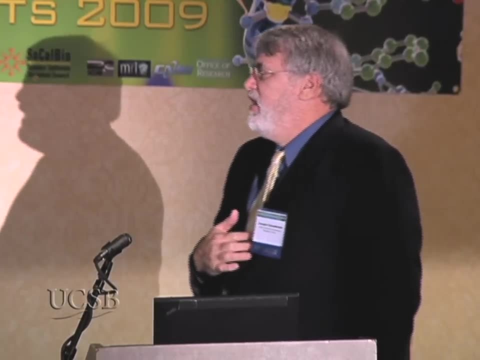 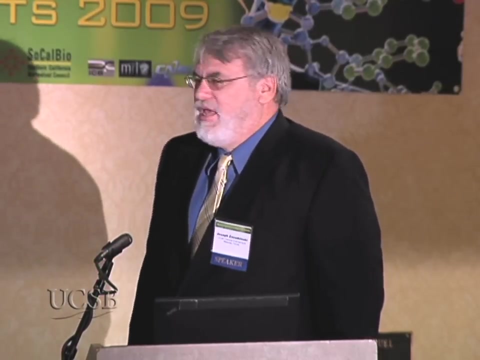 understand that in order to get any further. So our vesisome came out of- if you'd like to be fancy about it- a mimic of the eukaryotic cell. So a multi-compartment structure can do more things than a single compartment. 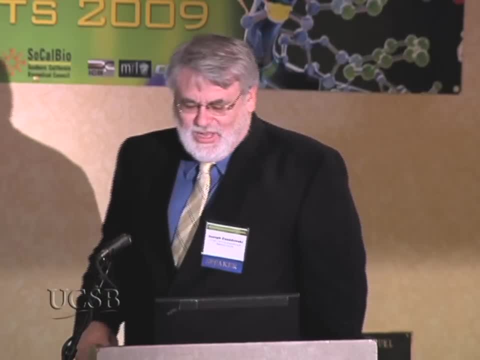 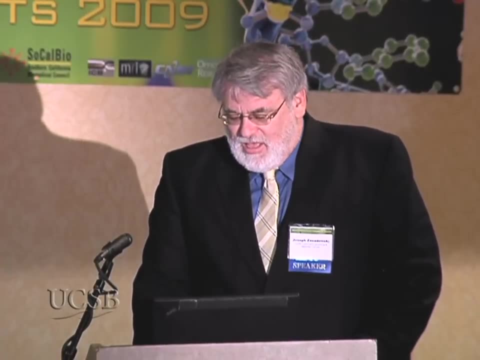 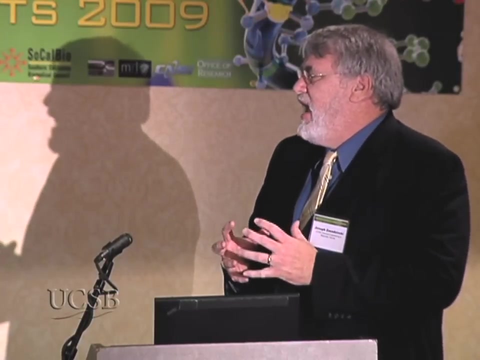 structure And really what it came from is my experience as a bag boy at Stater Brothers Market when I was a student in 2018.. It takes a little bit more work, but basically all we're doing is putting one lipid bag that could be of a different composition. 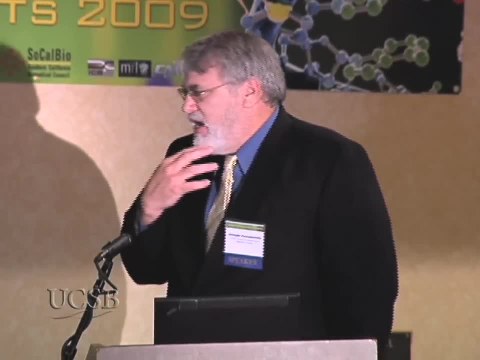 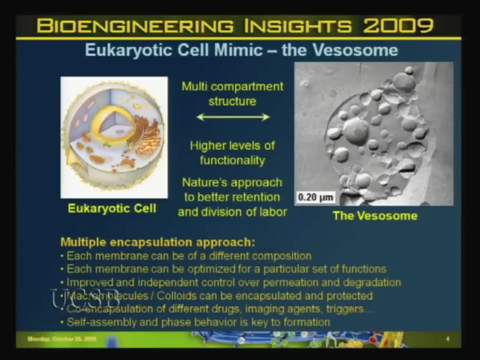 inside of the bigger lipid bag. We do this to try to optimize the function of each of the bags to get a better retention and control over drug release in the circulation. The other thing is we can also try to optimize the function of each of the bags to get a better retention and control over drug release in the circulation. The other thing is that we can change one or two kinds of lipid bags from which the different types of lipid bags are stored, and then they get improved. 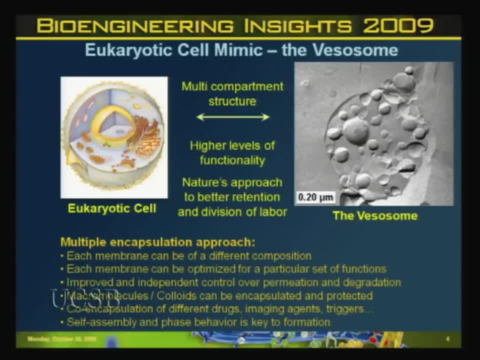 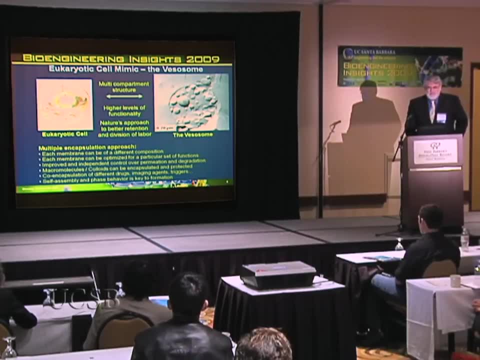 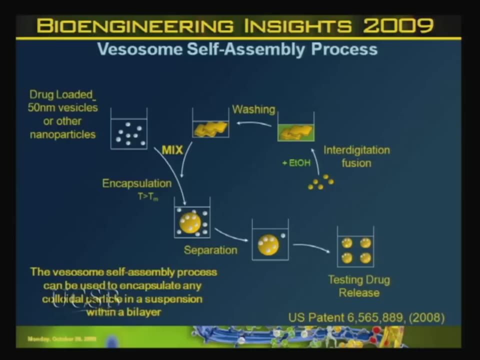 The other thing is that we can put almost anything we want of colloidal dimension inside of a lamellar bag using some pretty simple phase behavior. So this is what we have to do, And one of the sort of guiding principles of engineering is trying to keep things simple. 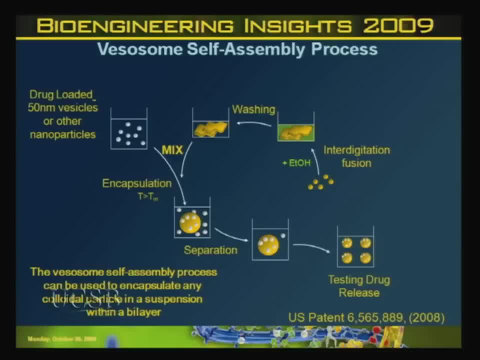 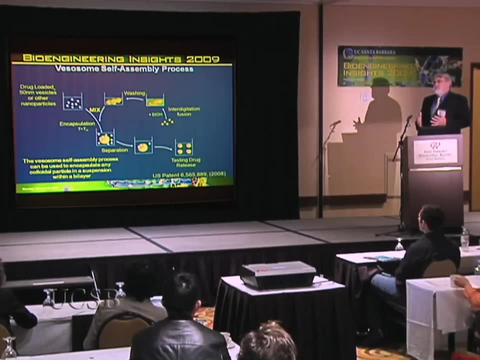 I don't know if that's a guiding principle of medicine in general. It doesn't seem to be, But we'd like to do everything so it's scalable and that the only steps that we have to do are heating things up and cooling things down and mixing. 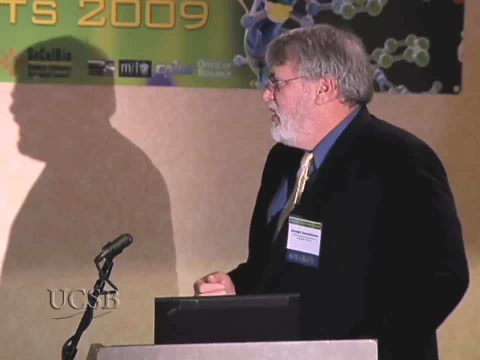 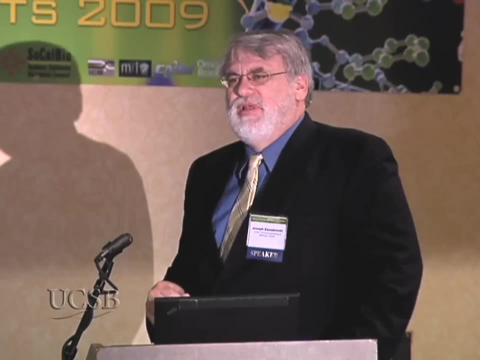 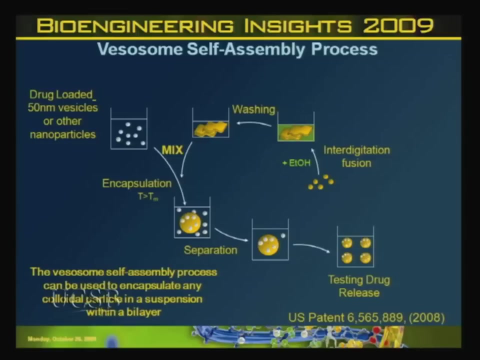 Those things we can do pretty efficiently. So what we do is we take lipid vesicles made out of certain saturated lipids and we mix them with a little bit of ethanol and water. This causes a change in the bilayer structure that normally is structure. 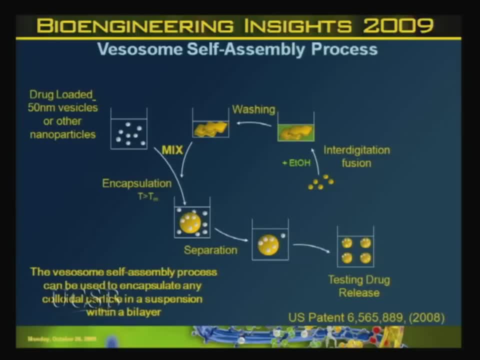 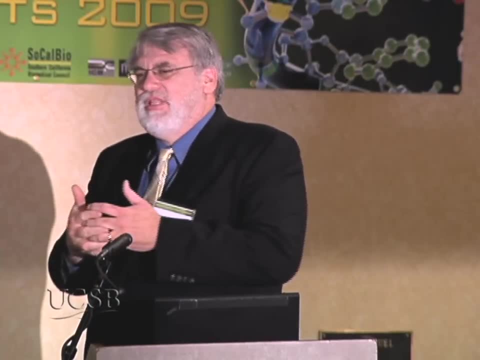 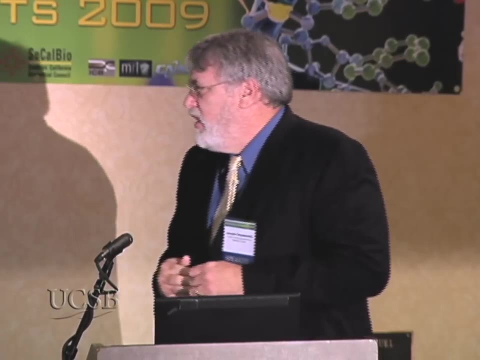 That normally happens. Instead of the normal bilayer, the ethanol causes the layers to interdigitate, And as you interdigitate those layers, the membrane gets stiffer. It can't bend as well, And so it makes flat sheets. So now we have open sheets of lipid in our solution. 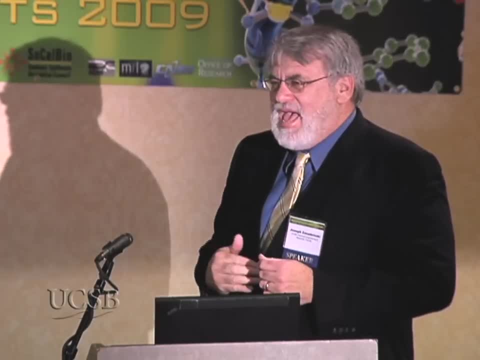 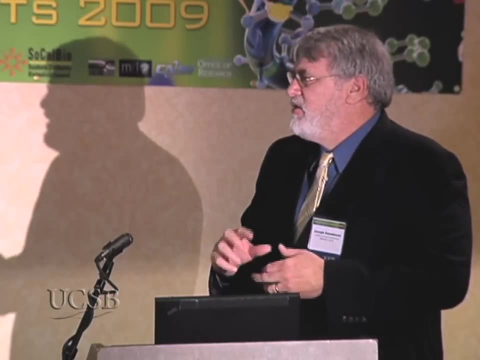 We can remove the excess ethanol And we can add whatever we'd like to that that we want to encapsulate. It could be vesicles, It could be other nanomarins, It could be other nanoparticles, It could be drug particles, et cetera. 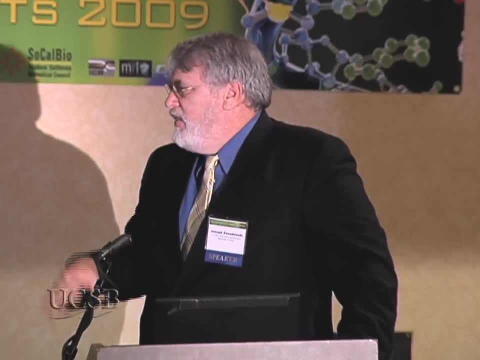 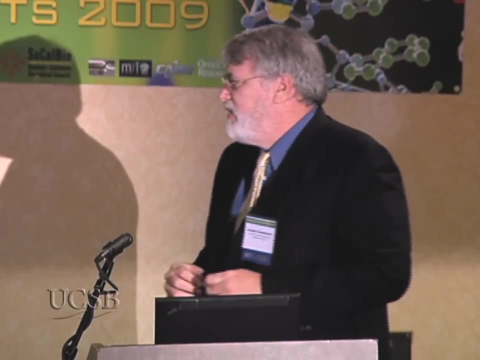 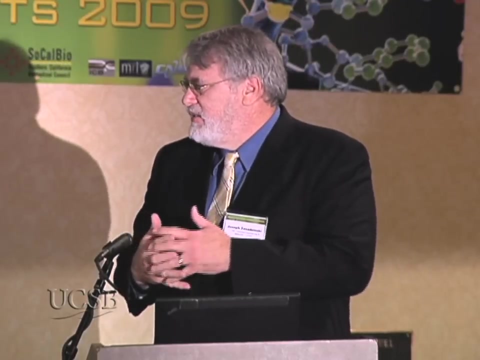 We mix it together and we heat it up. This heating process makes the membranes more fluid again. They close like thousands of little butterfly nets around whatever happens to be in solution And we encapsulate. In this process of encapsulate we don't catch everything. 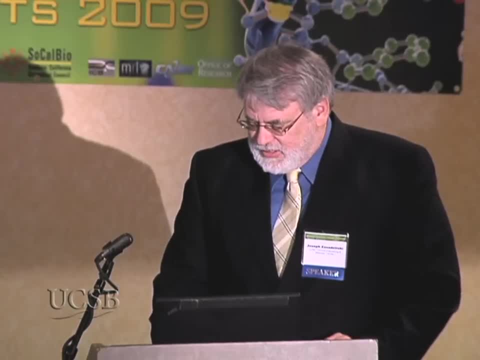 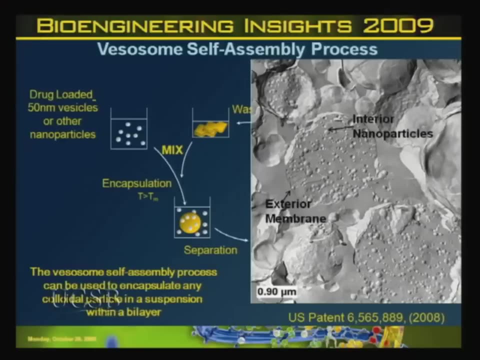 You never catch all the butterflies, And so we do some separations and then we can go test this, And this is what it looks like at the microscopy level. We have particles on the 50 nanometer leg scale. These are small vesicles trapped inside of a bigger membrane. 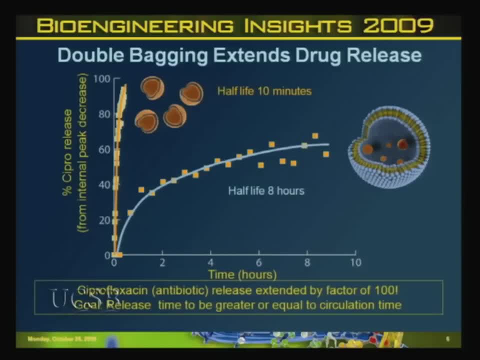 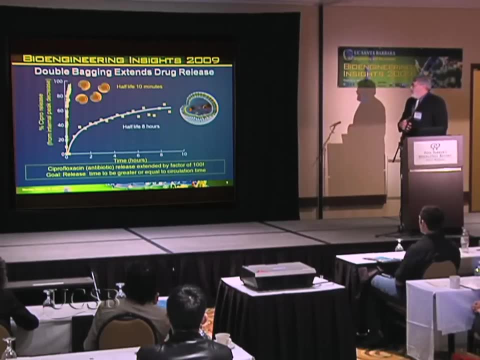 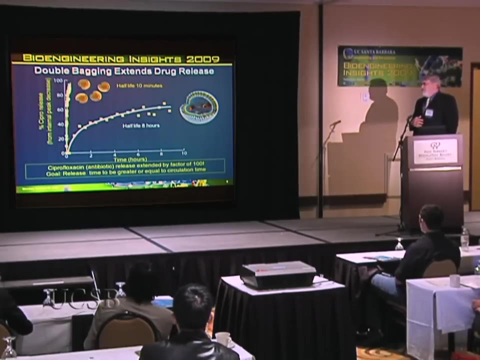 And why do we do this? It turns out that we get an incredible extension of drug release in serum. This is a little graph of what happens when we put Cipro, Which is a nice amphiphilic antibiotic that happens to be fairly difficult to deliver. 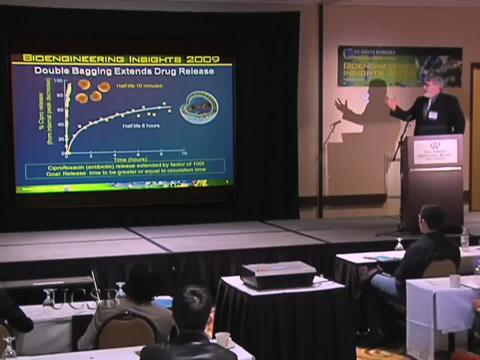 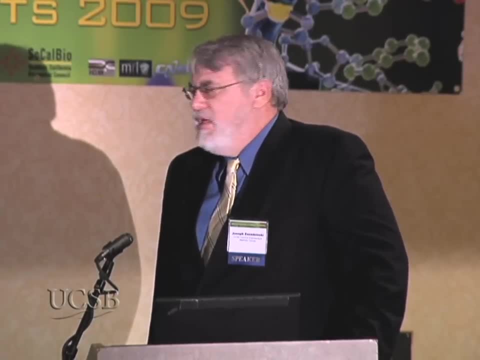 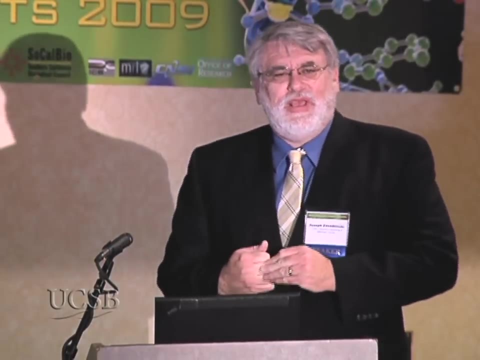 Into one of these carriers. If we just have a single membrane in serum, the half-life of the Cipro is about 10 minutes, And this is because there are thousands of things, And perhaps Dr Hood can tell us all what they are eventually. 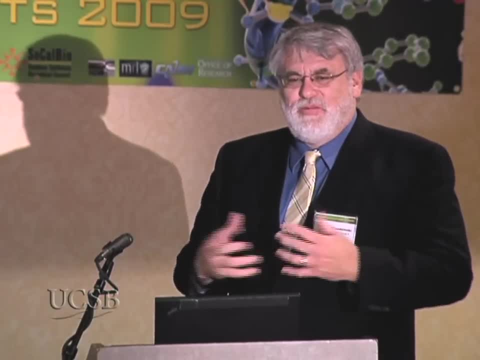 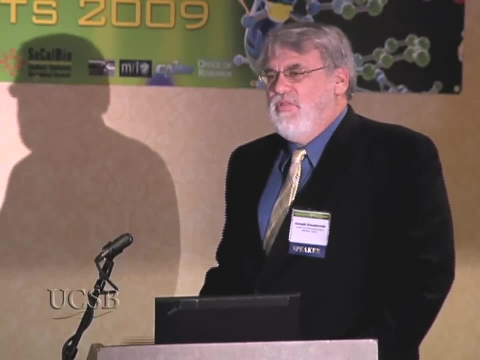 That like to eat lipid in your bloodstream And like to be able to eat lipid in your bloodstream And like to break down membranes Because that's their job. They don't know that this is a good bag as opposed to a bad bag. 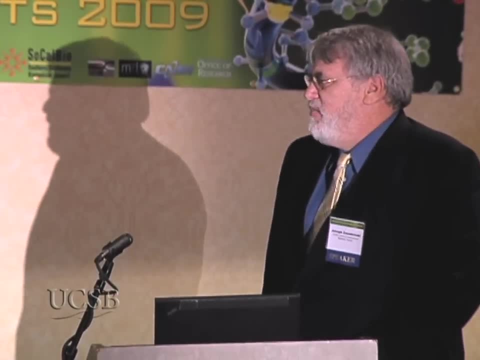 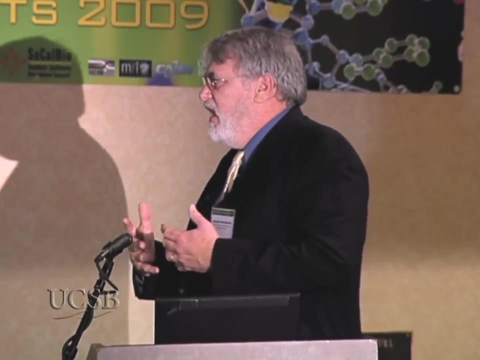 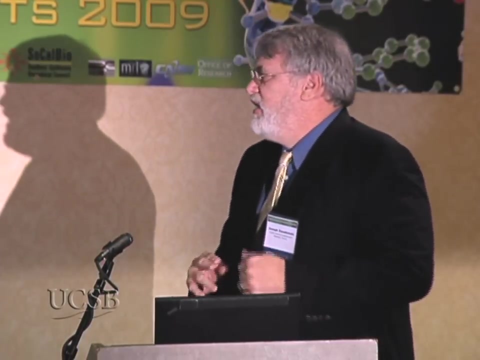 So putting in a bag inside of a bag. A lot of these things require transport into the membrane And even transport to the surface of the membrane in order to work. Lipases, enzymes And cholesterol agents. High density lipoproteins. If you have two layers, You have to go through one to get to the interior structures, And this just takes some time, And so we see an increase in half-life of the drug from about 10 minutes to more than 8 hours, Which gives us the opportunity now to have the release time be greater than or equal to 10 minutes. 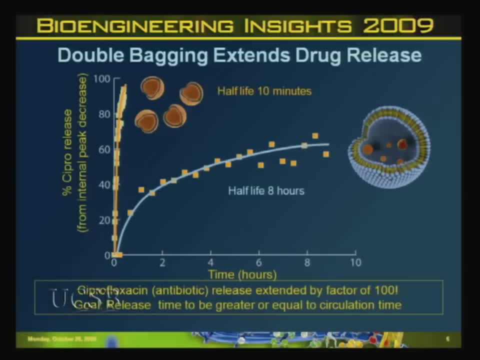 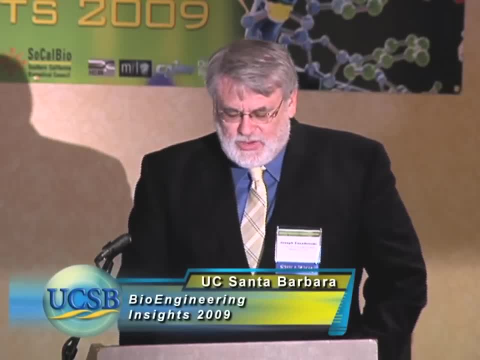 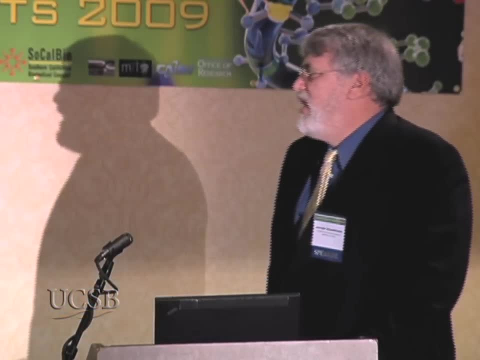 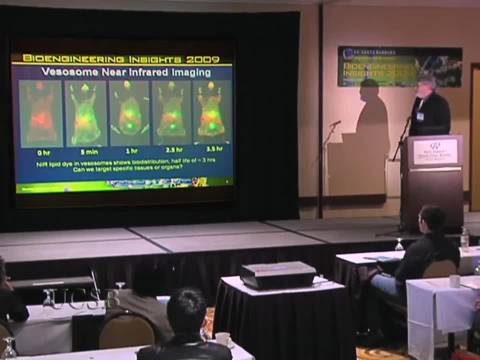 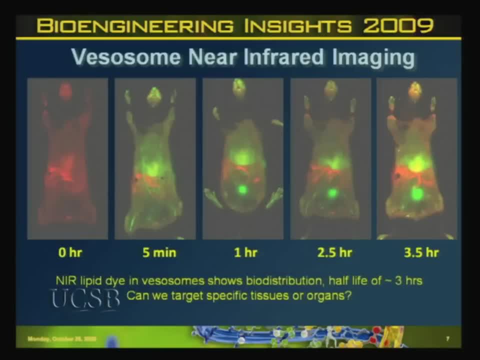 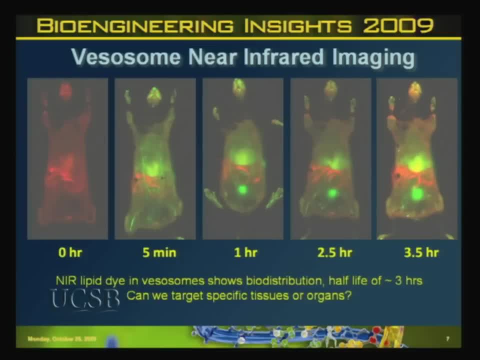 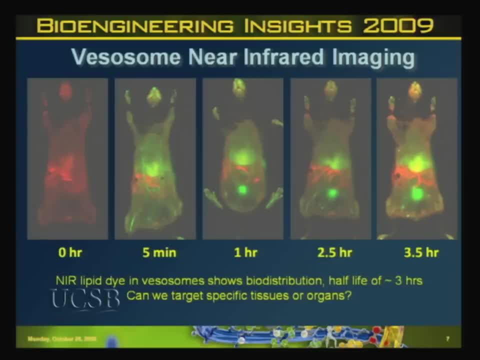 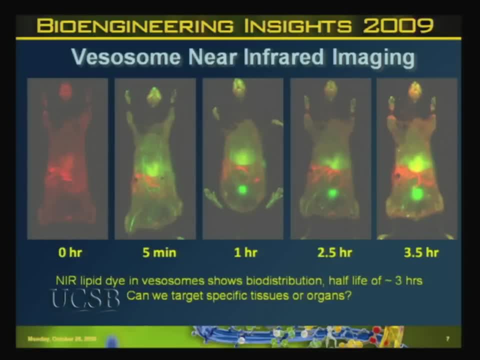 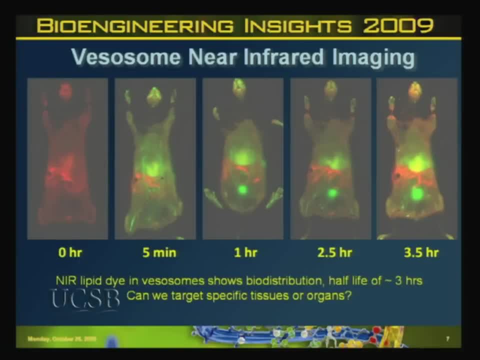 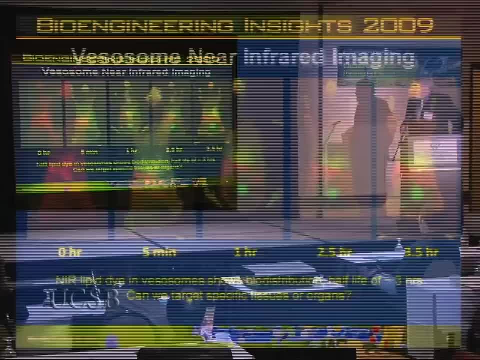 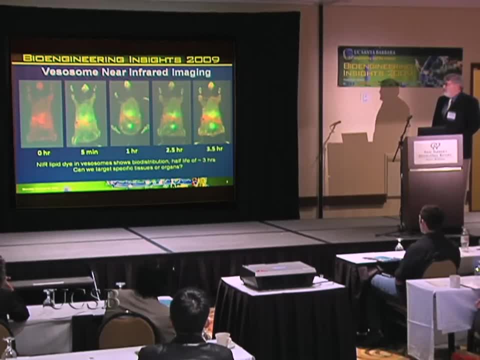 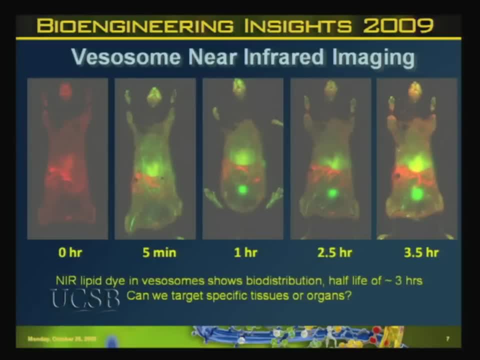 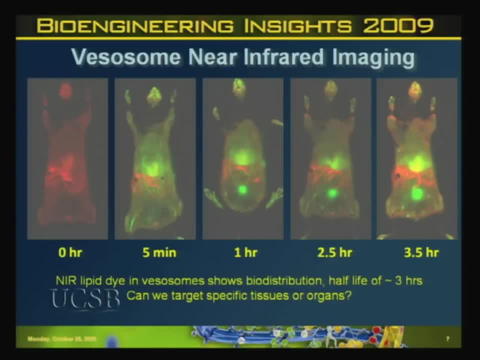 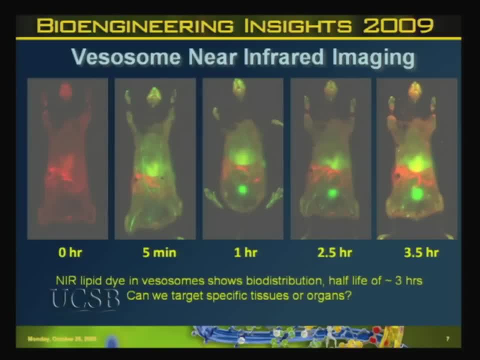 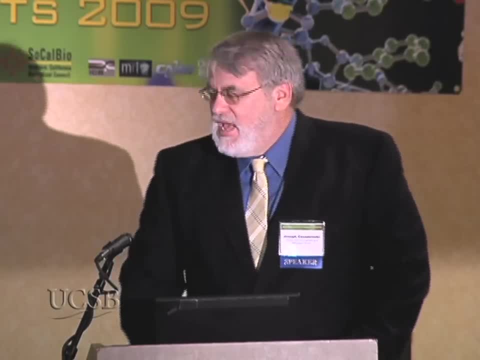 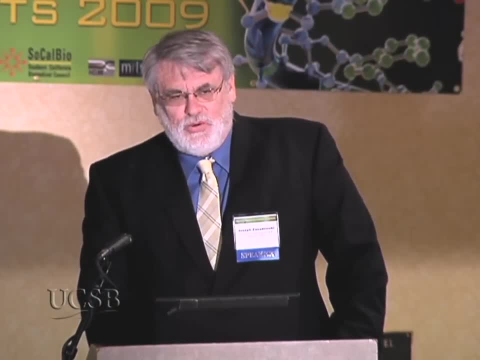 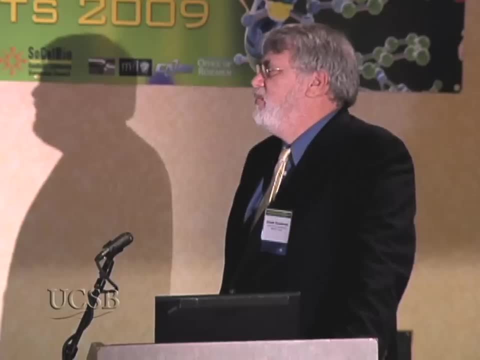 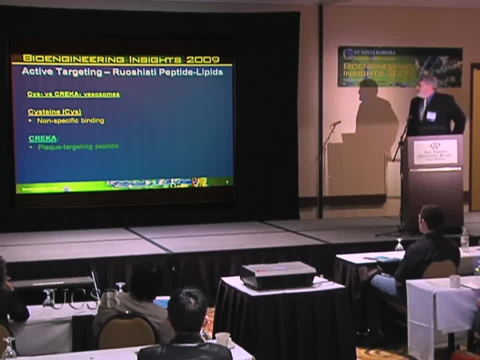 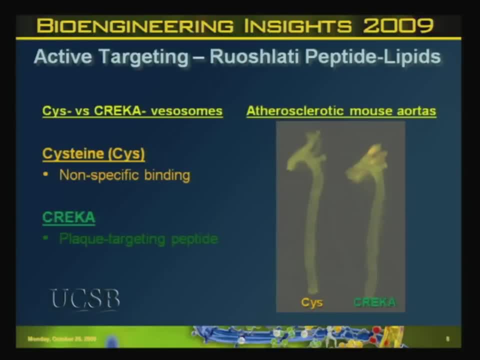 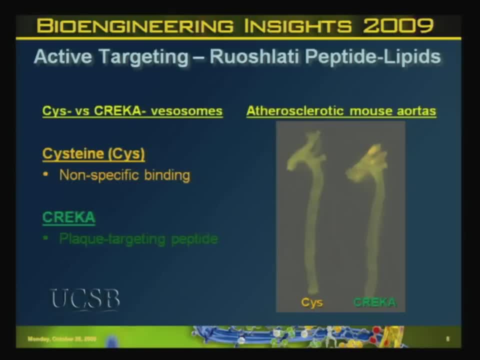 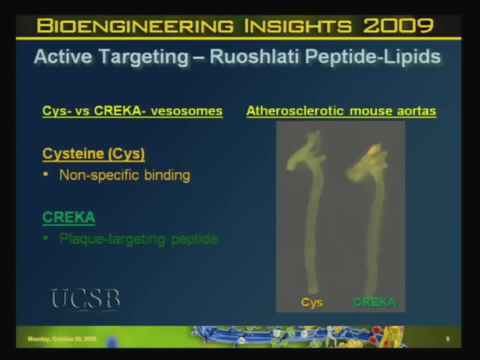 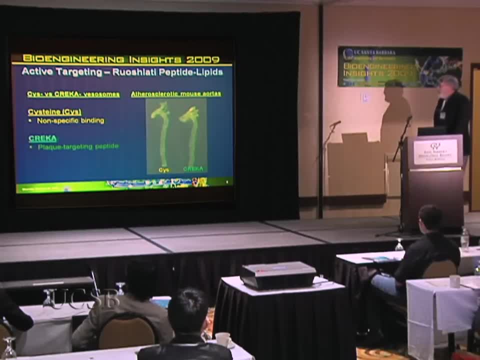 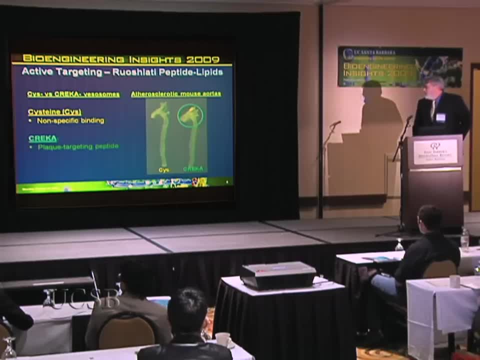 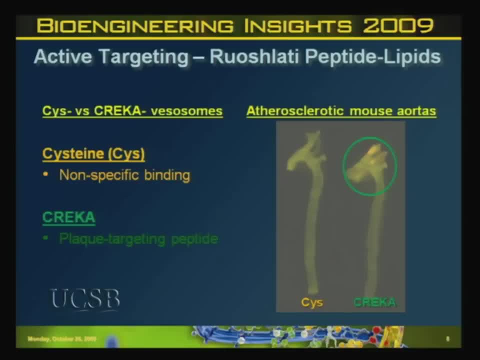 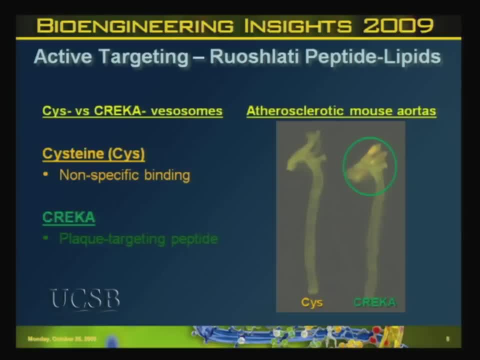 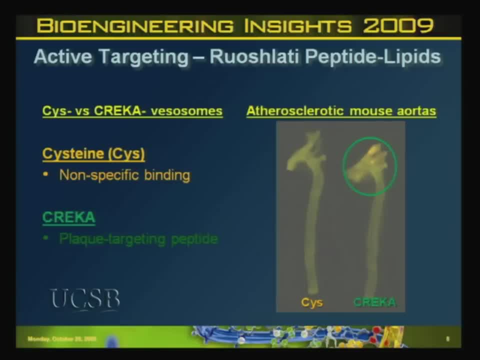 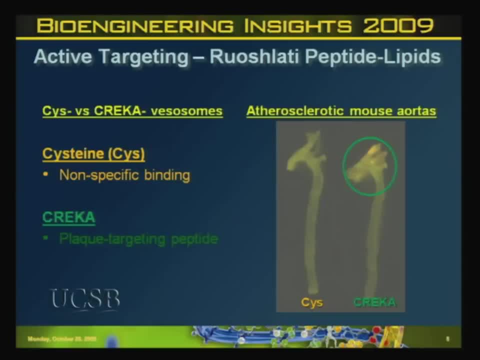 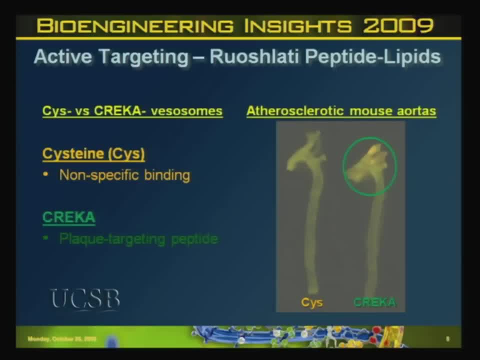 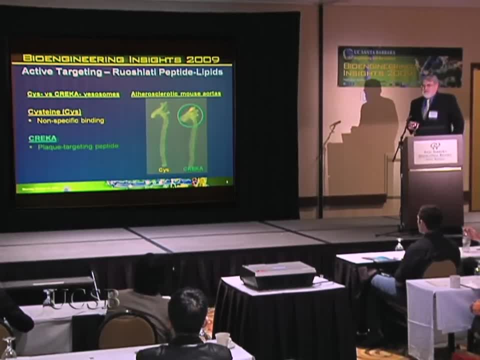 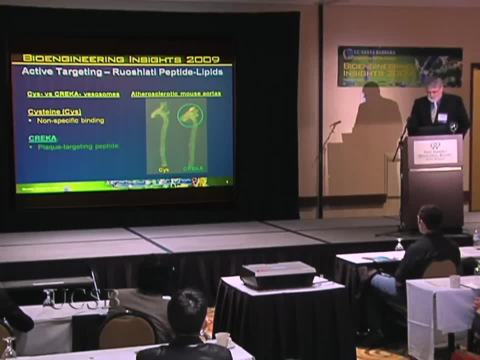 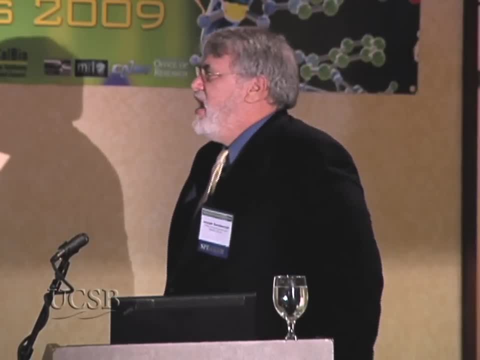 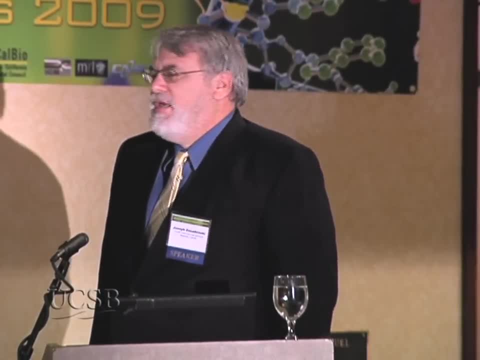 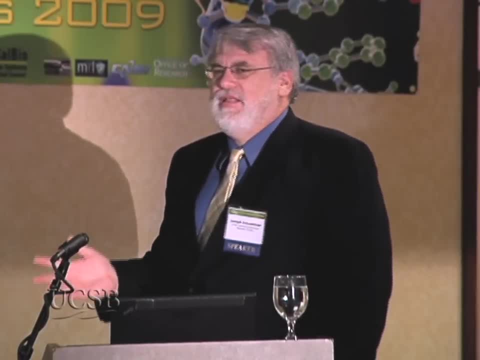 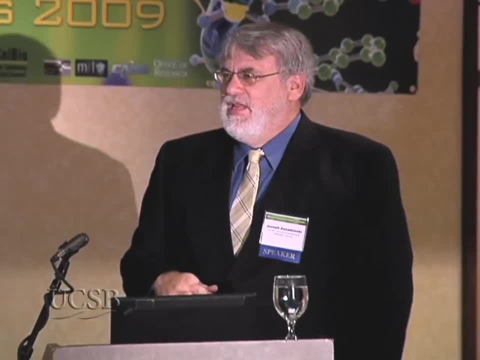 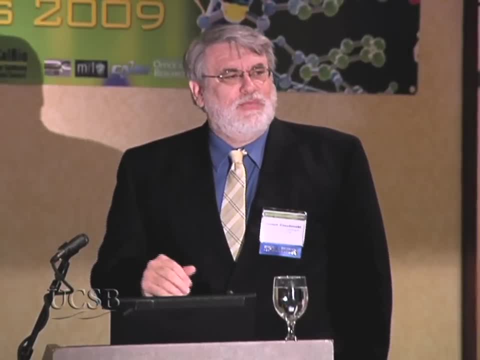 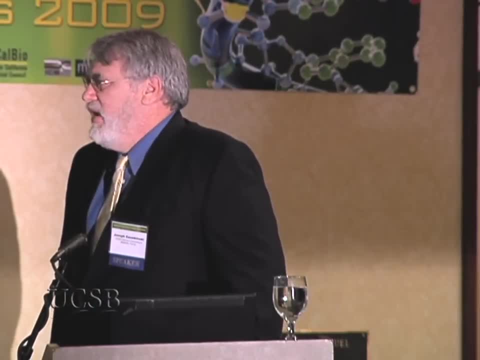 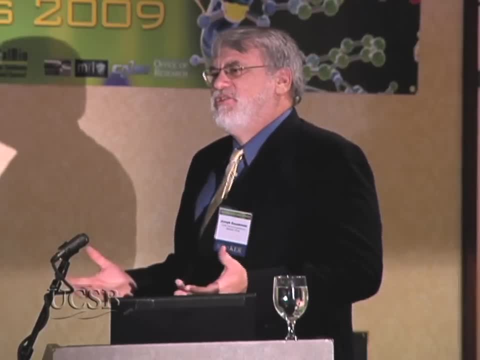 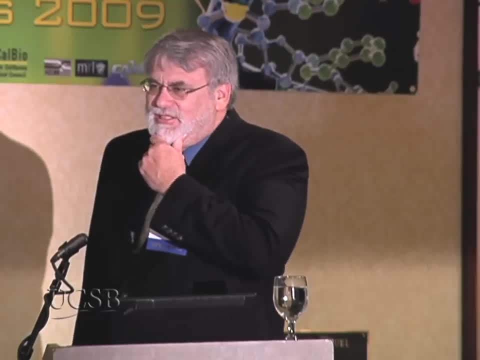 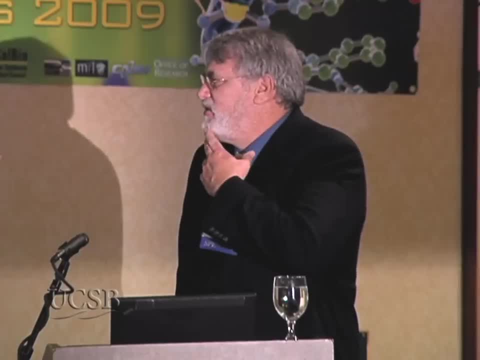 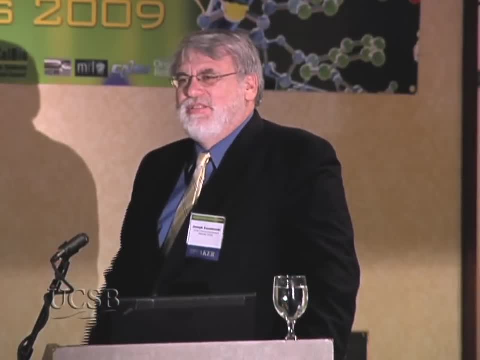 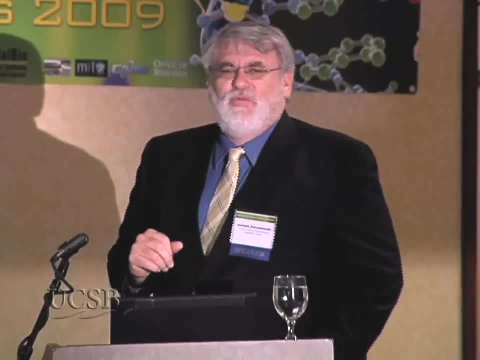 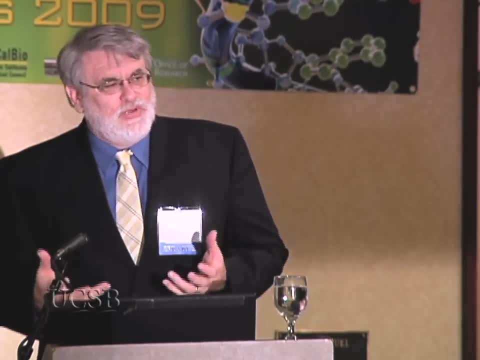 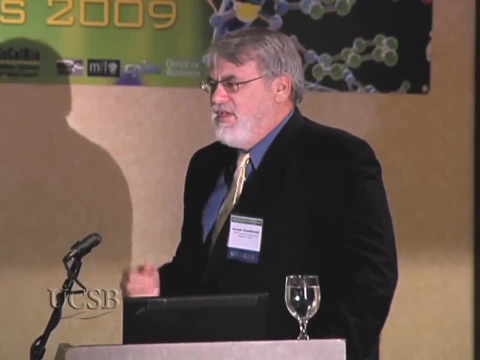 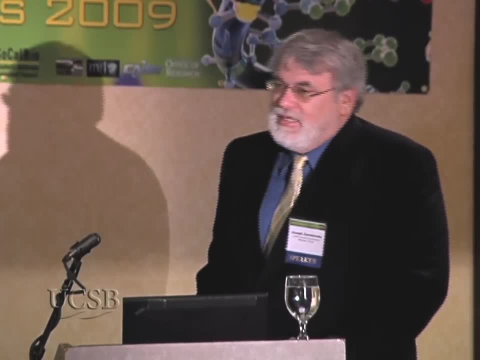 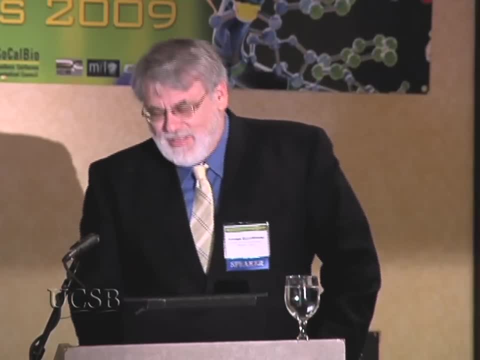 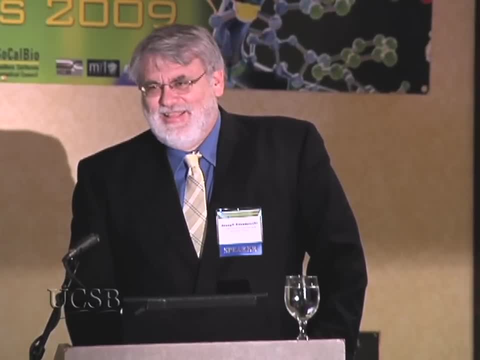 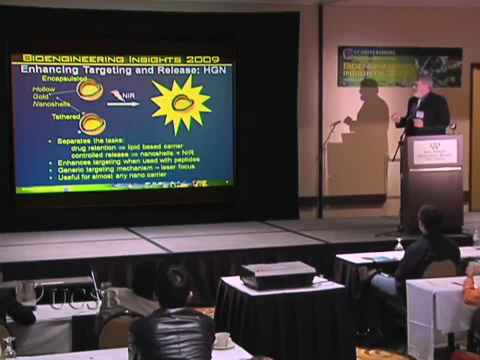 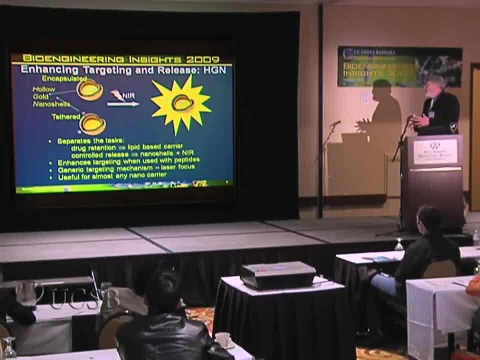 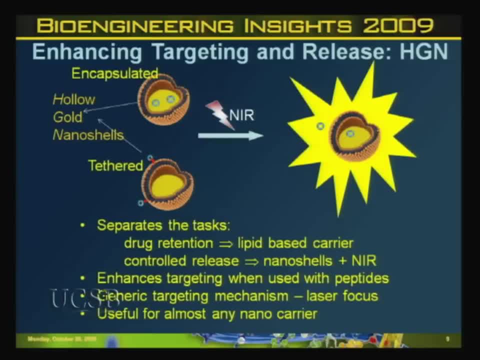 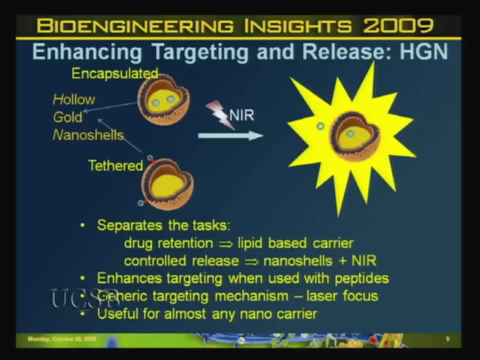 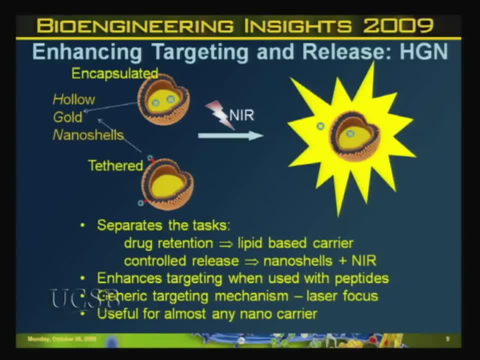 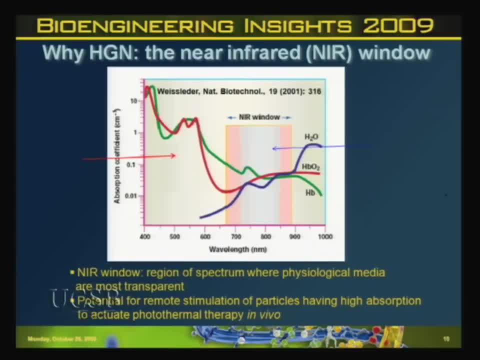 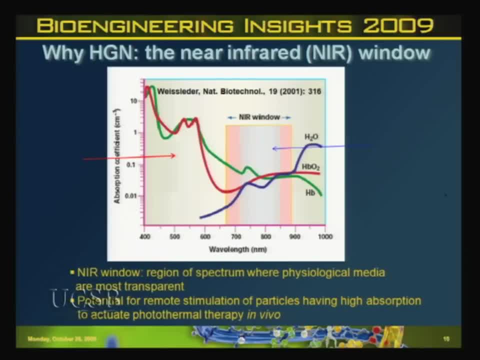 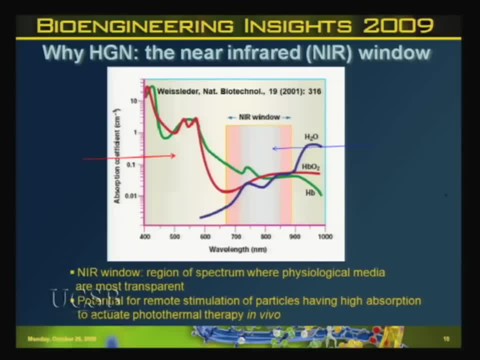 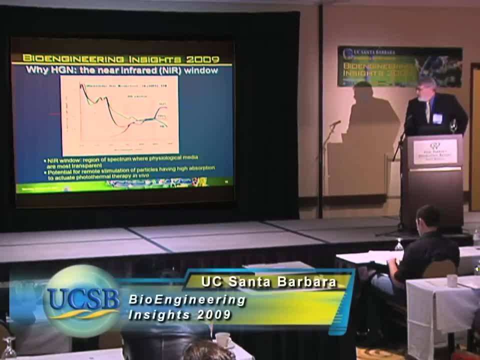 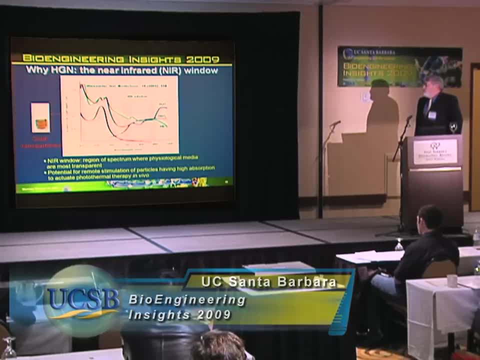 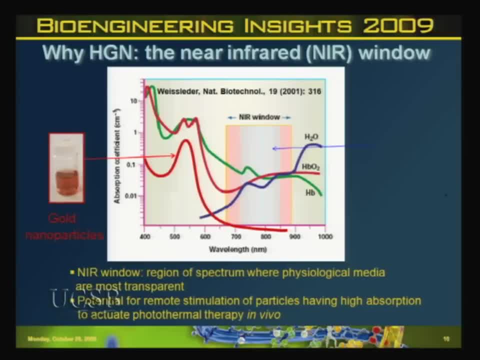 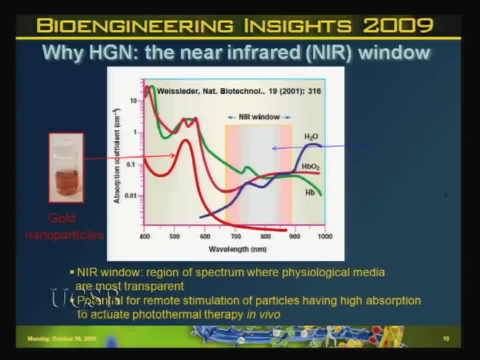 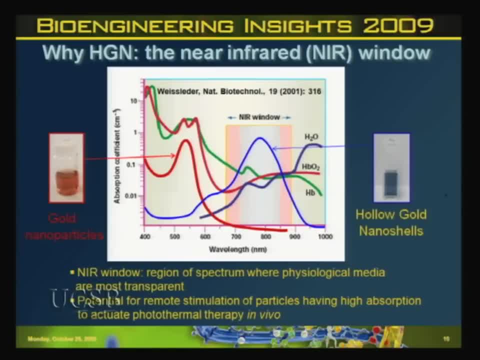 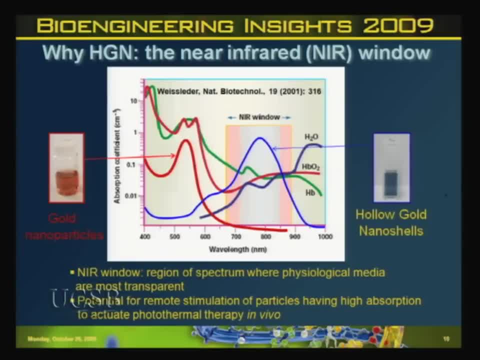 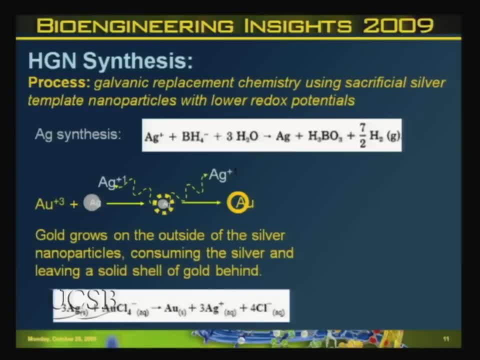 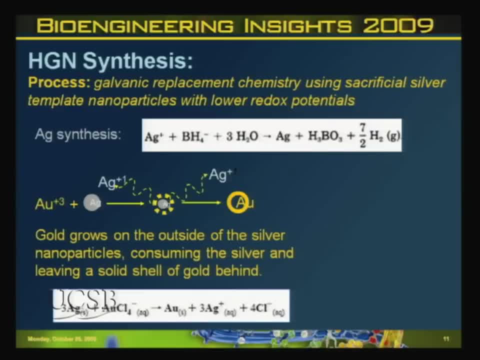 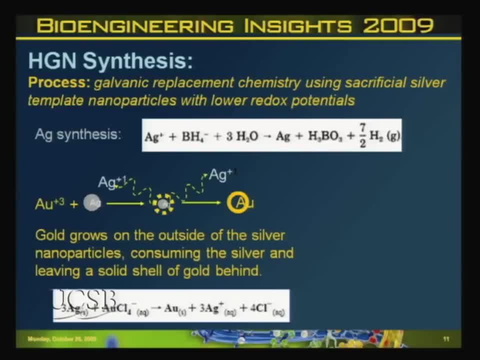 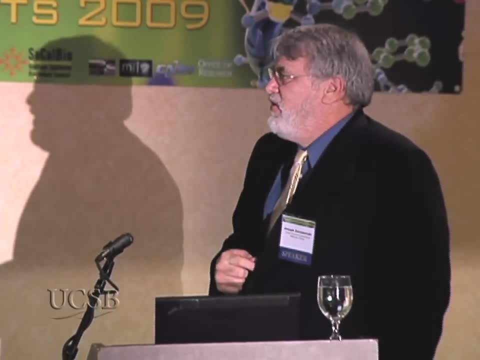 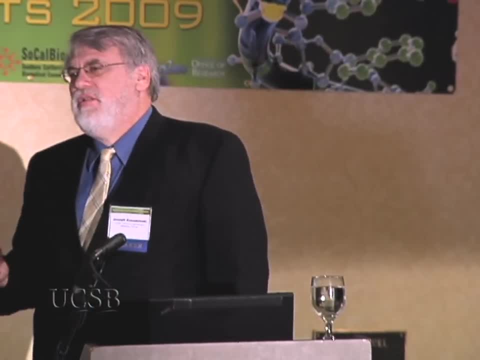 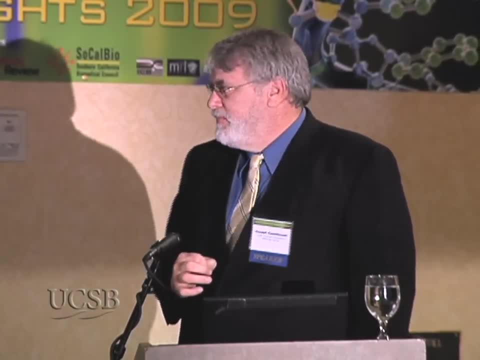 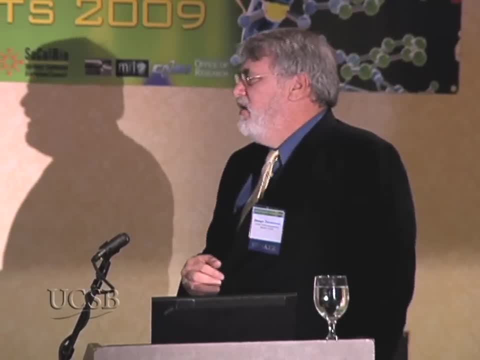 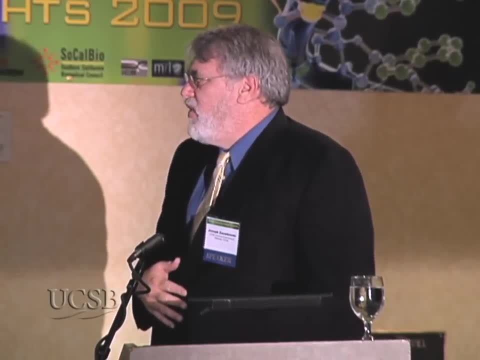 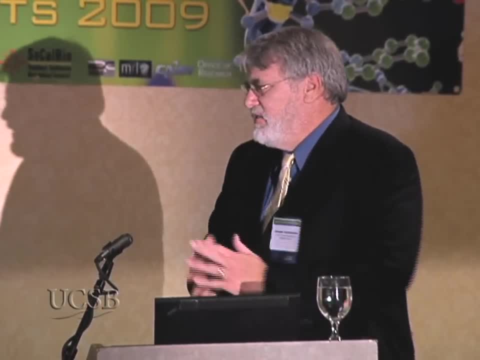 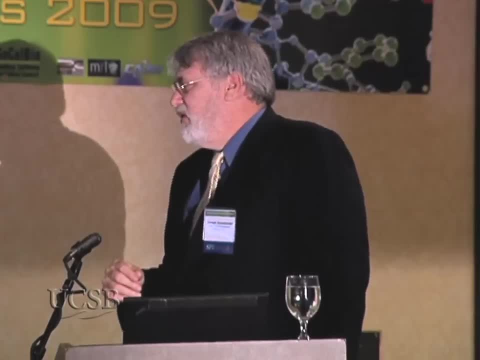 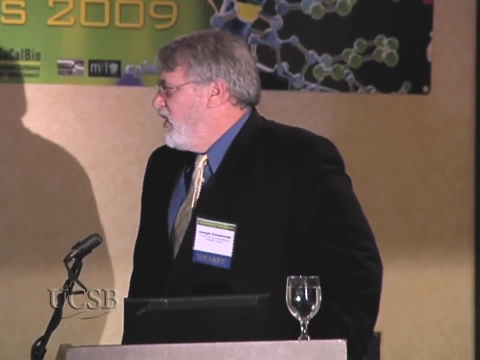 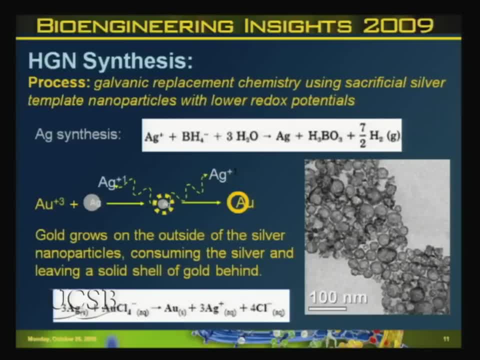 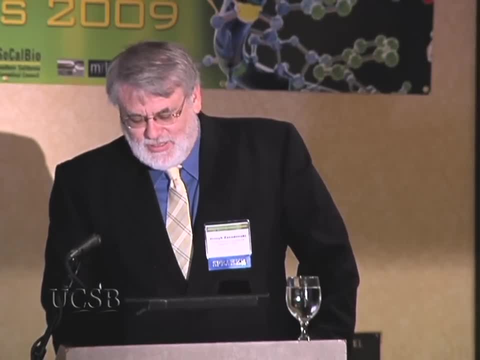 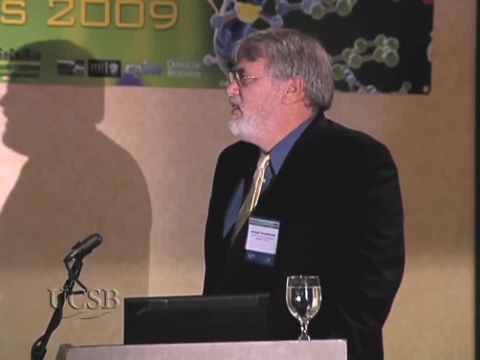 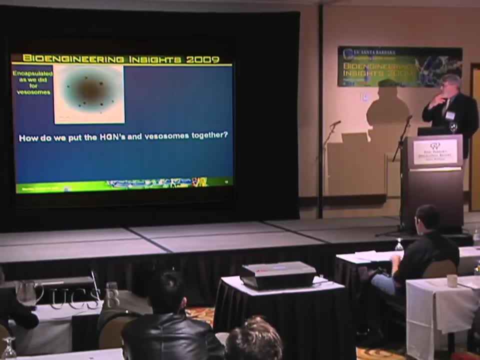 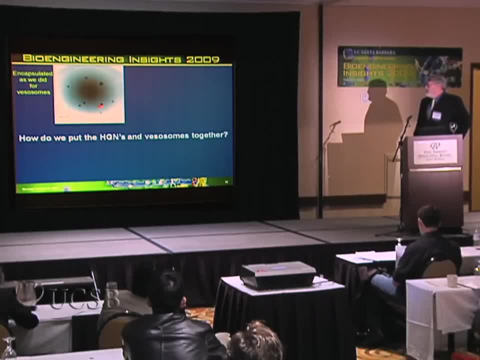 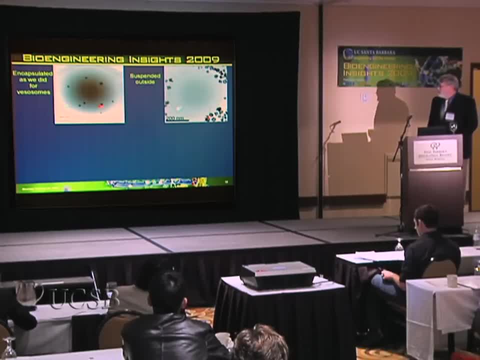 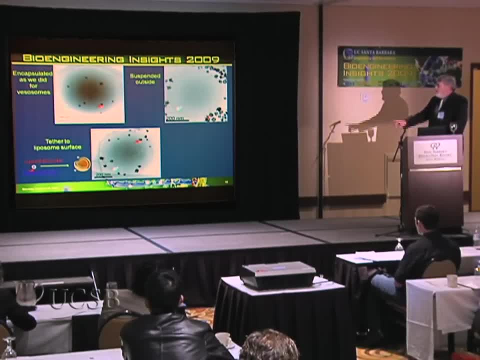 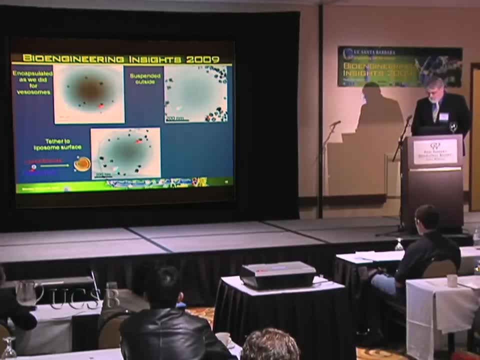 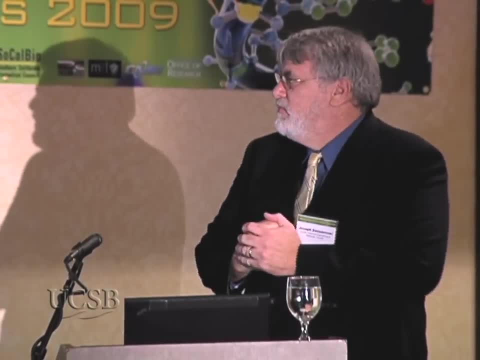 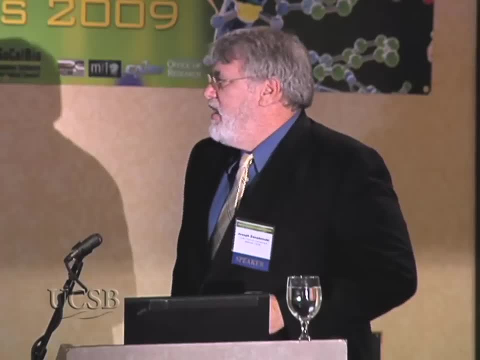 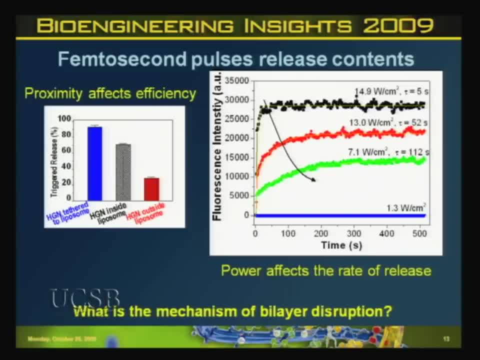 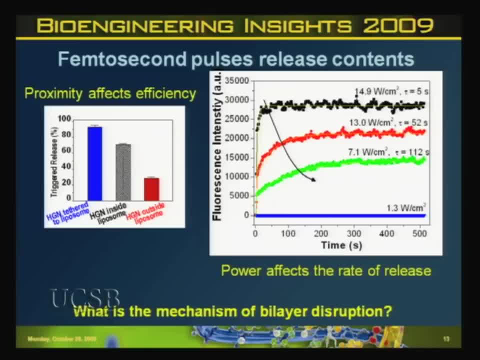 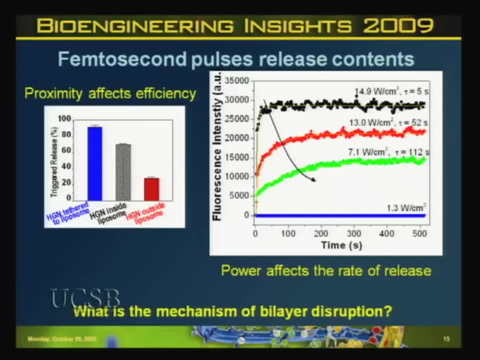 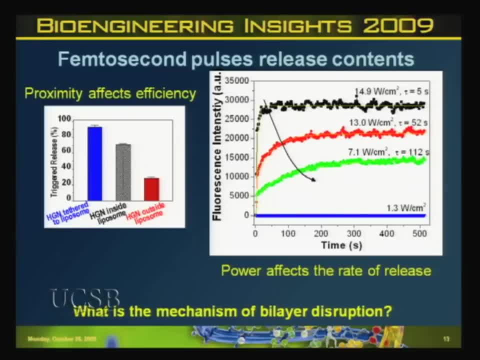 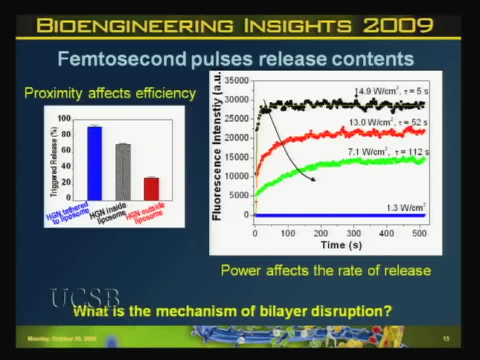 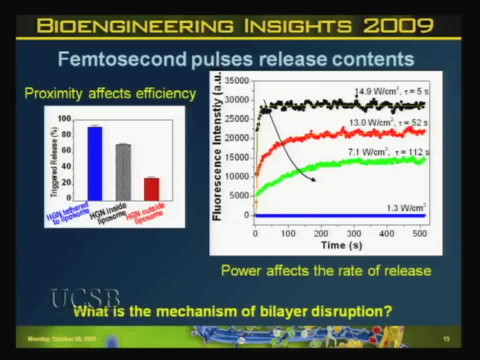 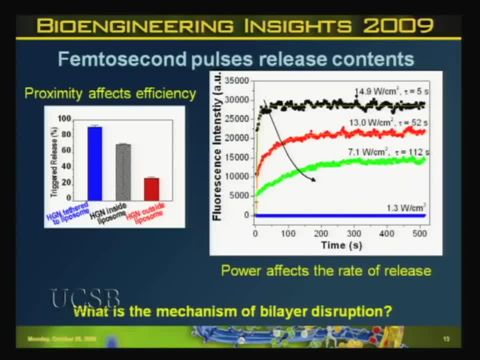 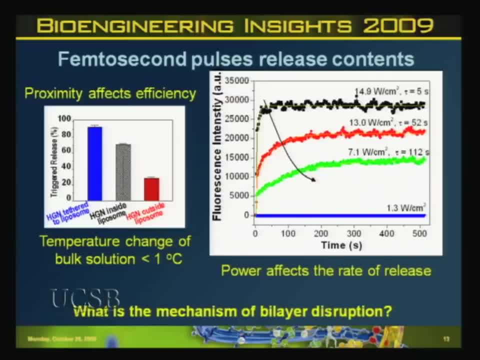 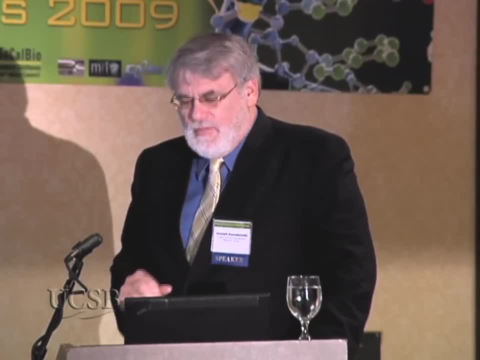 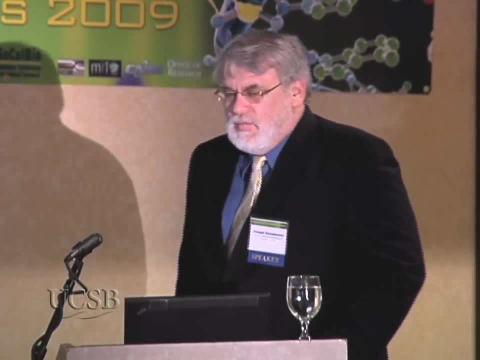 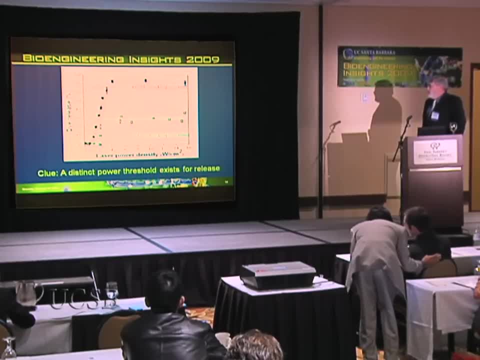 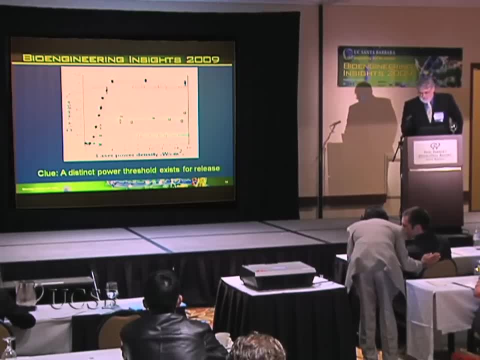 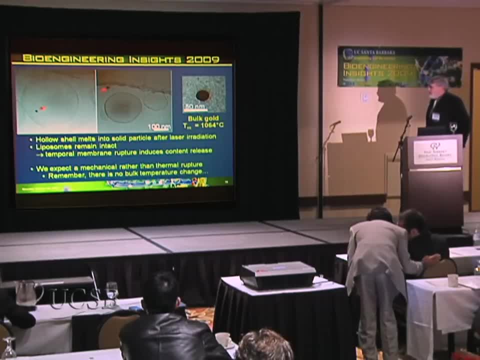 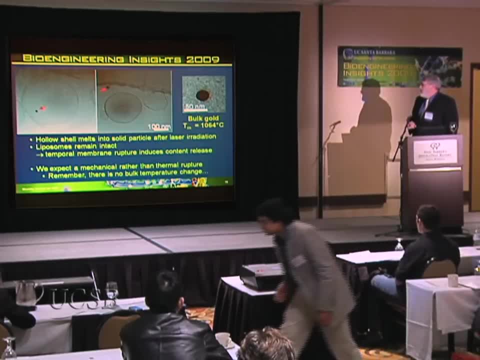 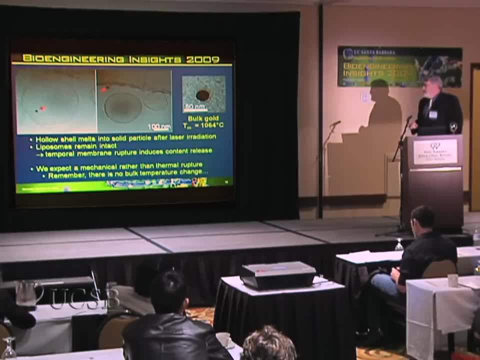 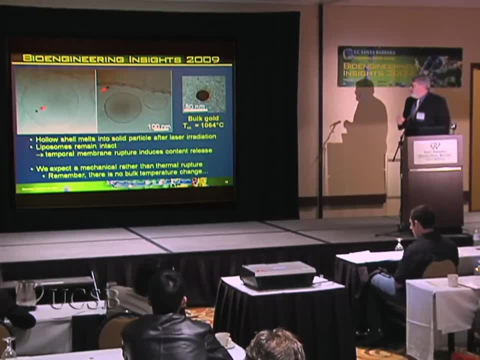 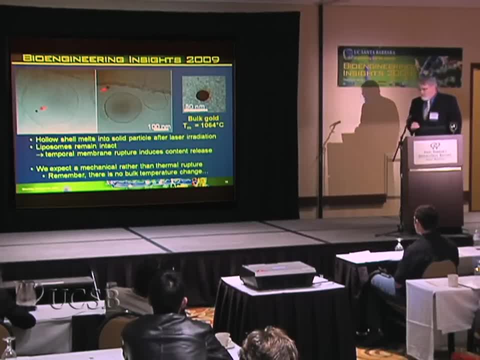 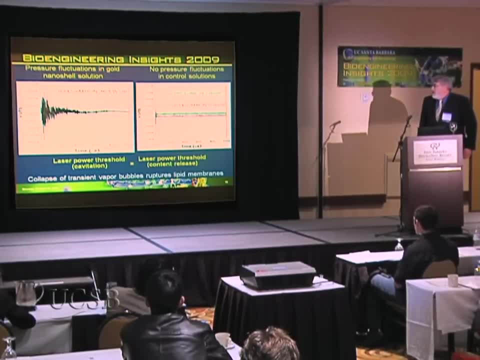 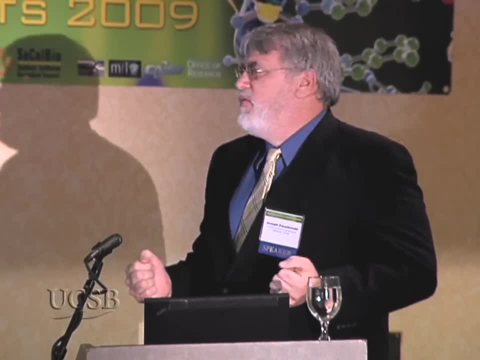 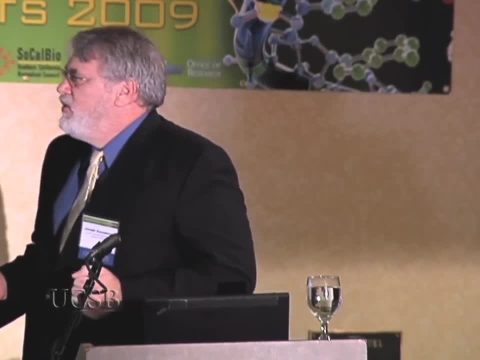 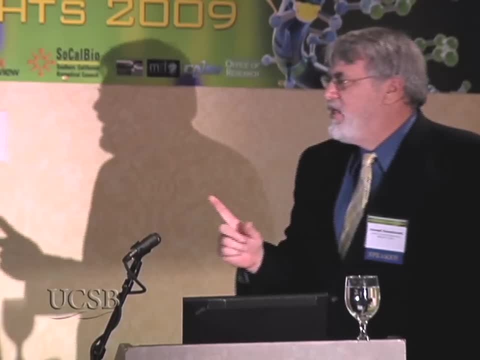 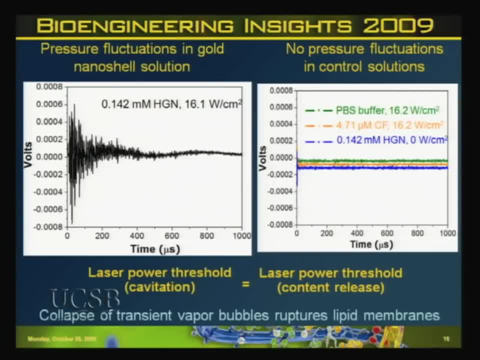 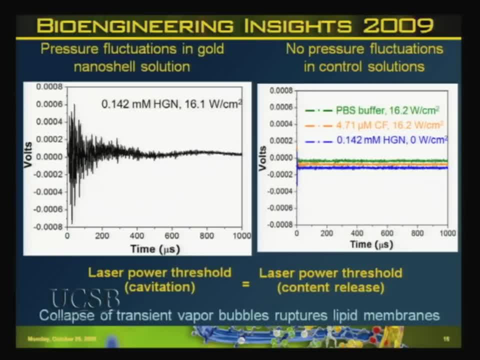 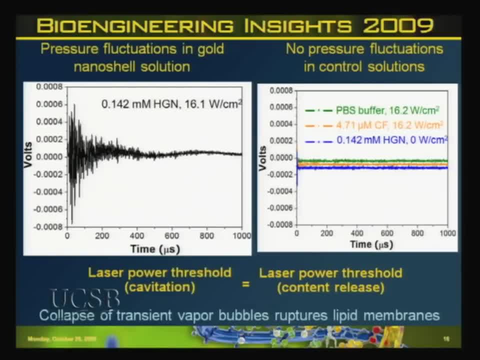 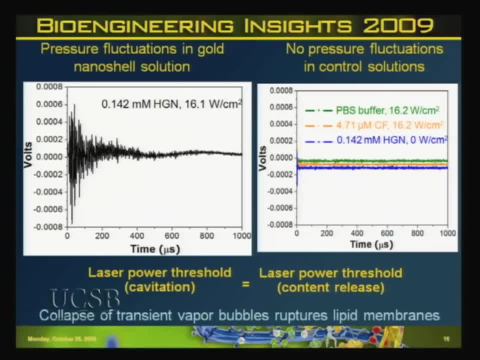 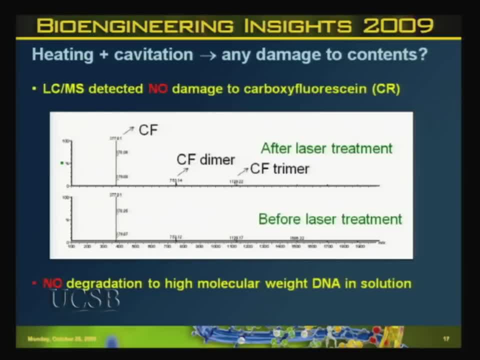 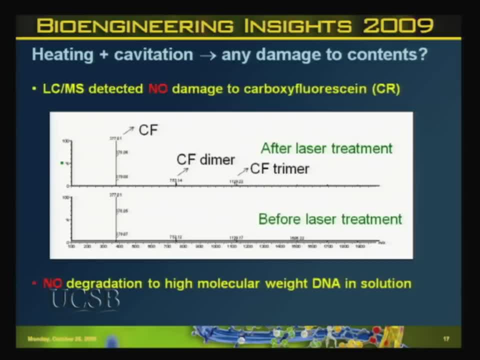 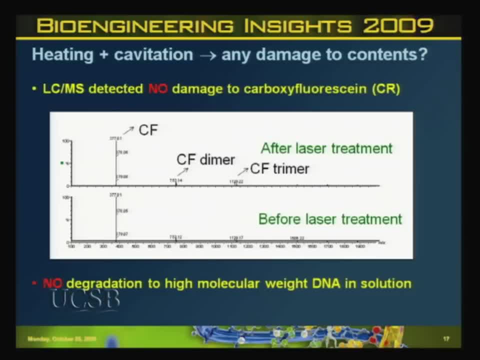 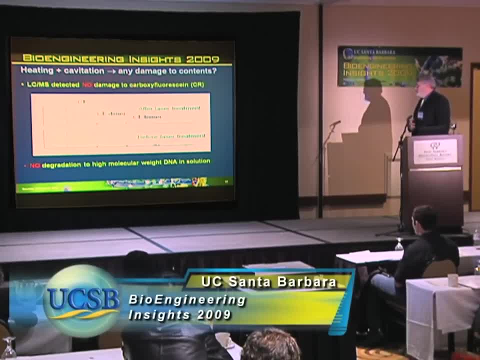 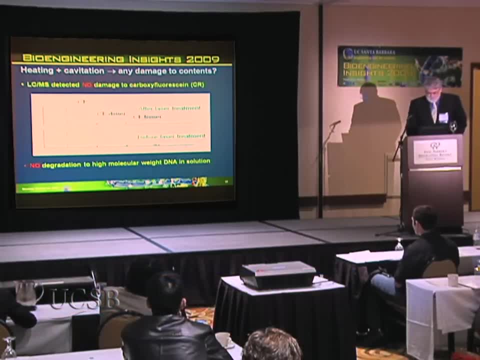 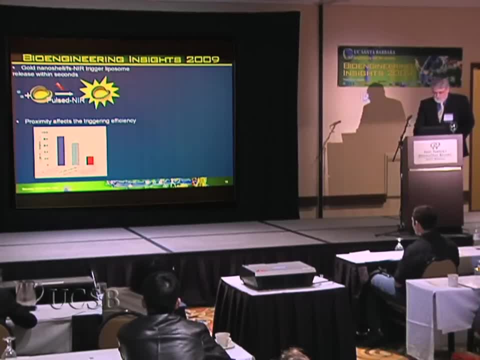 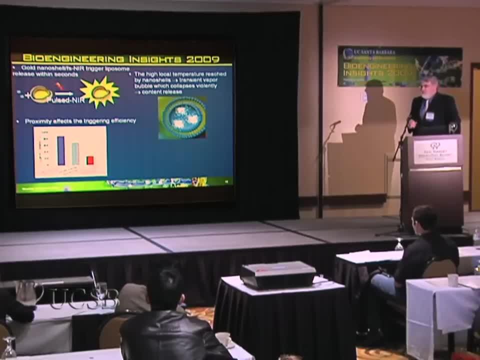 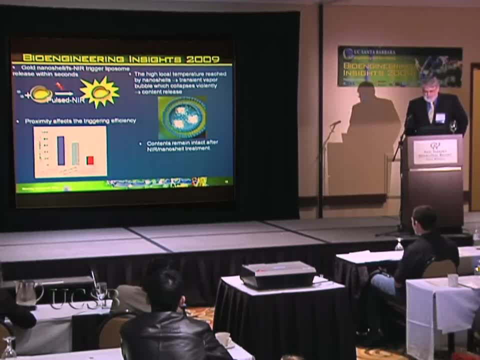 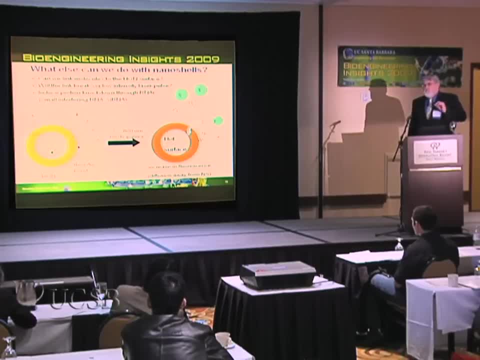 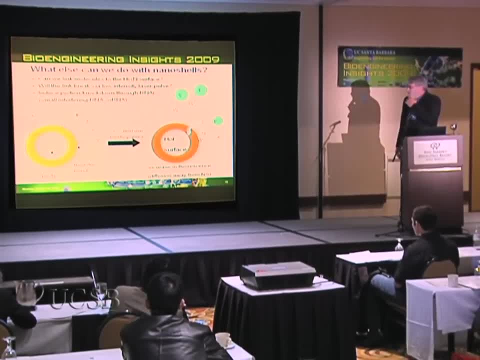 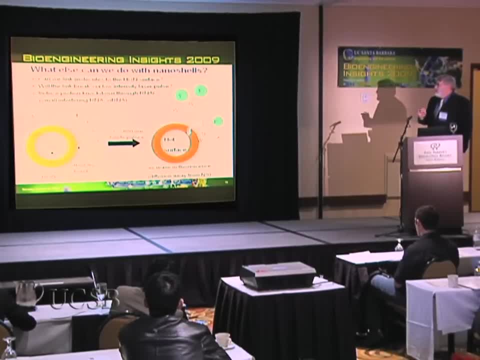 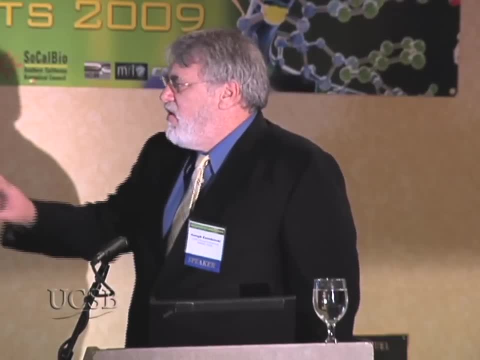 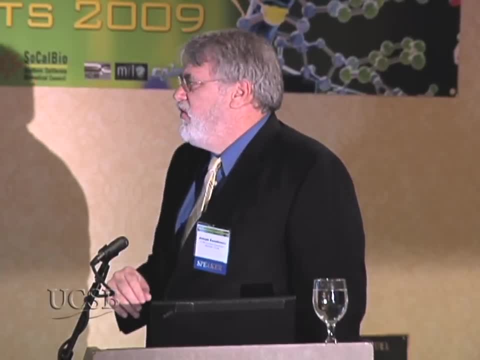 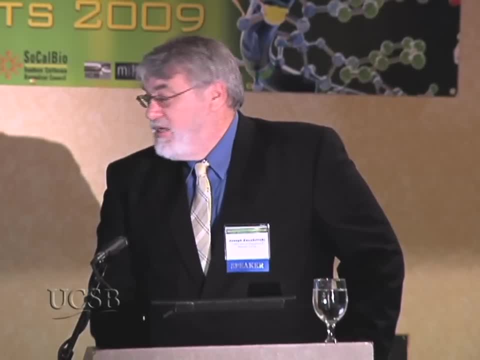 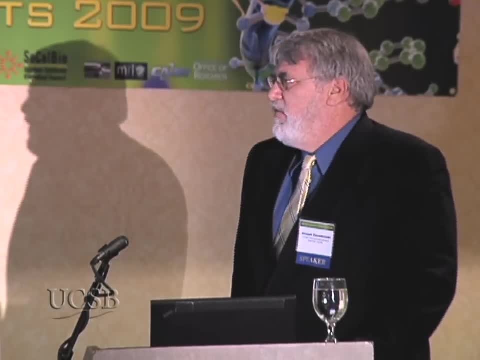 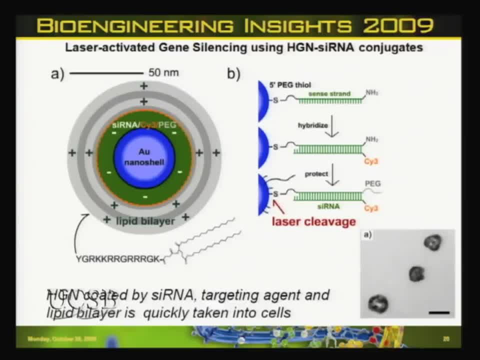 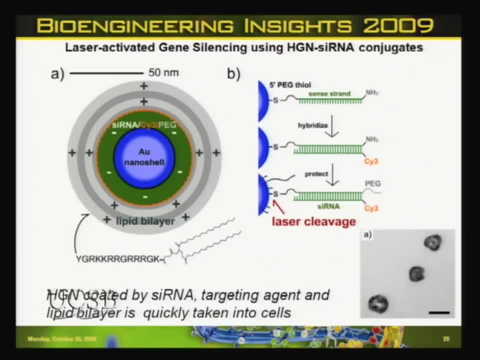 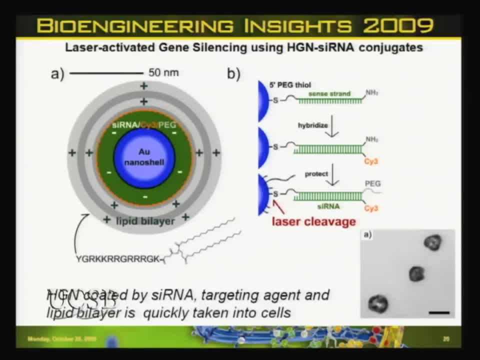 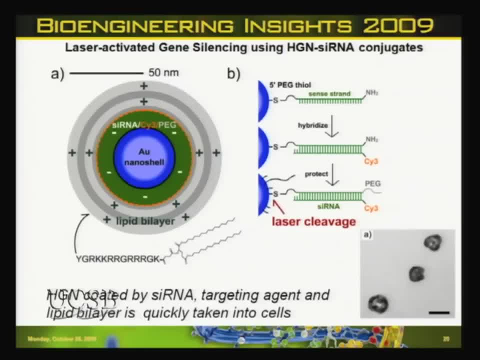 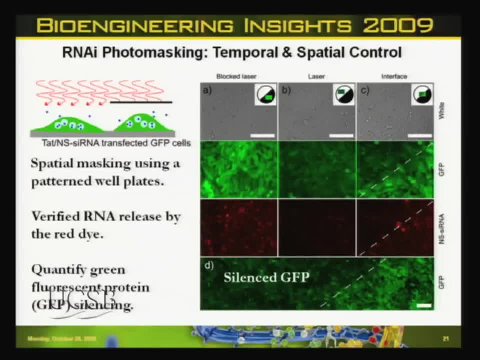 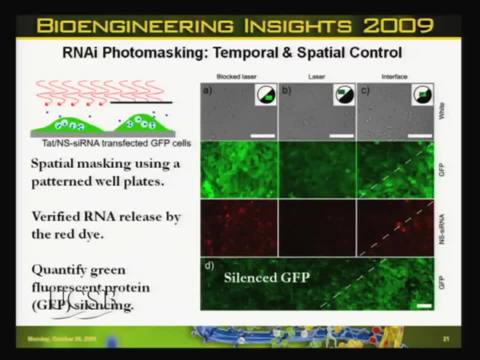 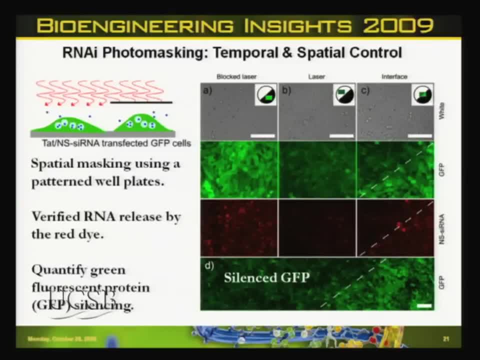 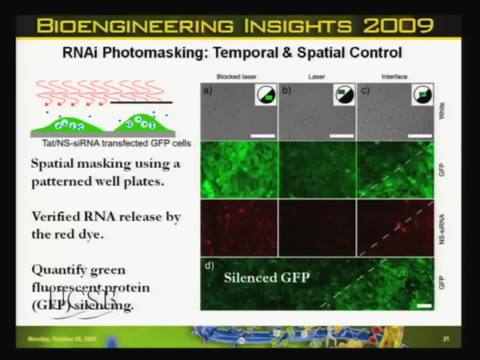 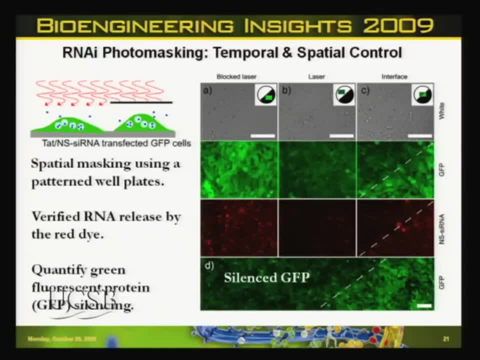 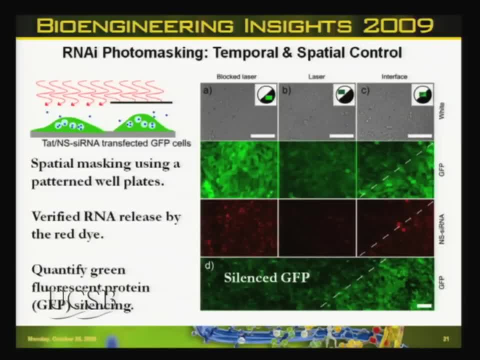 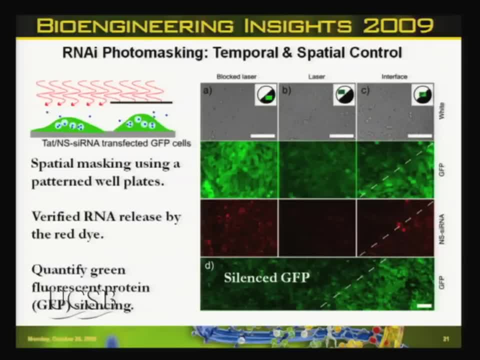 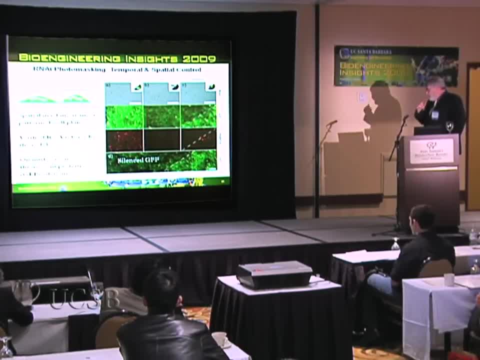 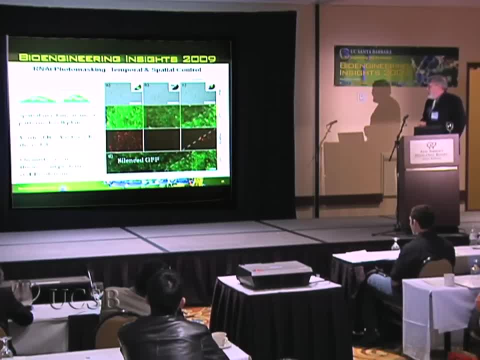 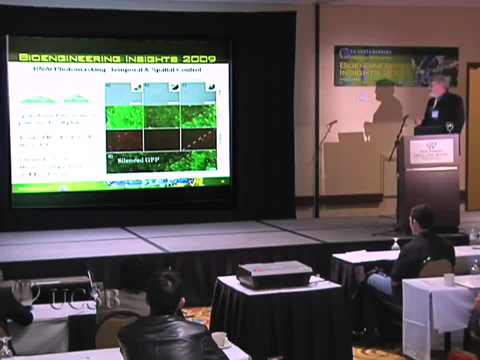 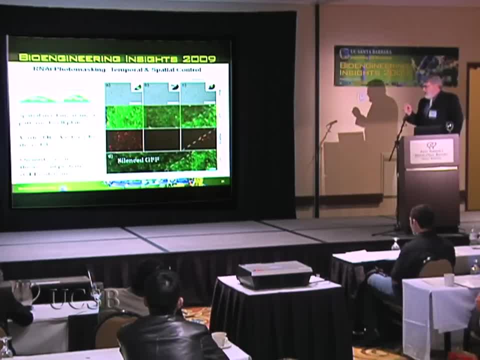 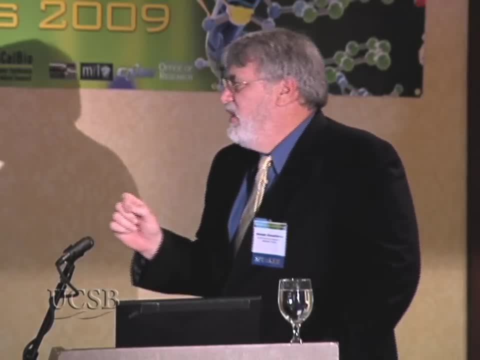 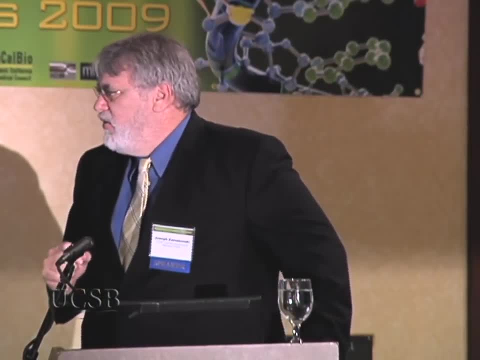 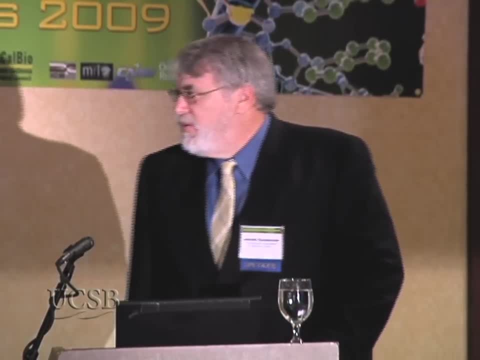 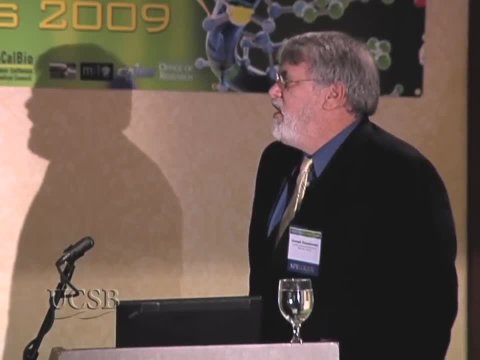 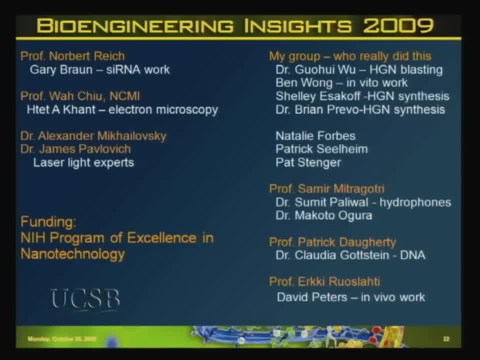 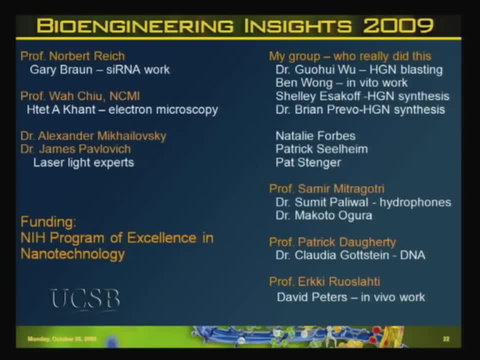 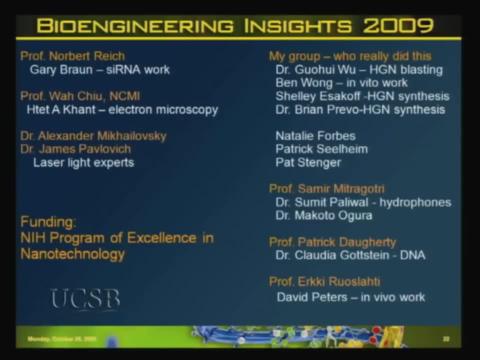 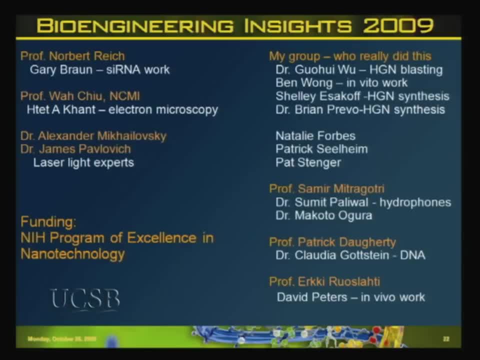 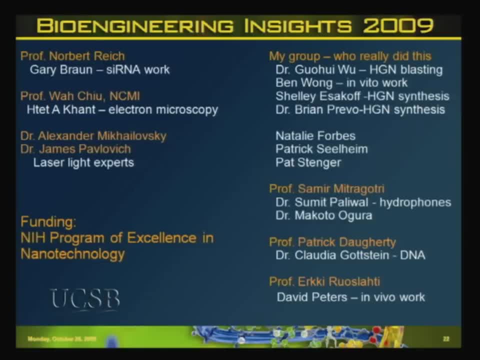 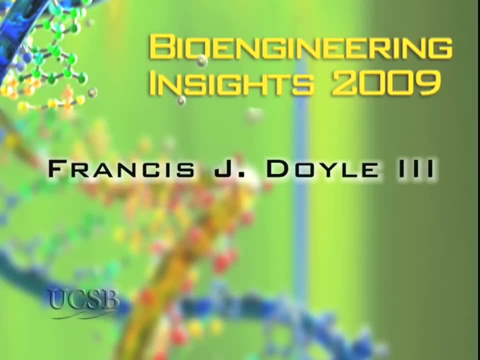 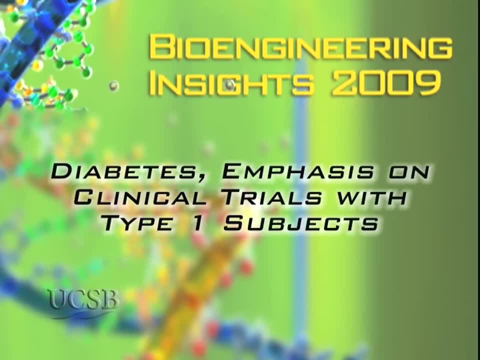 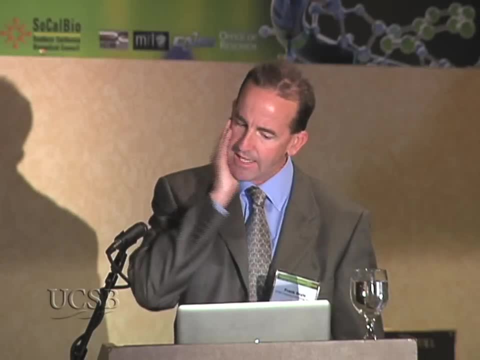 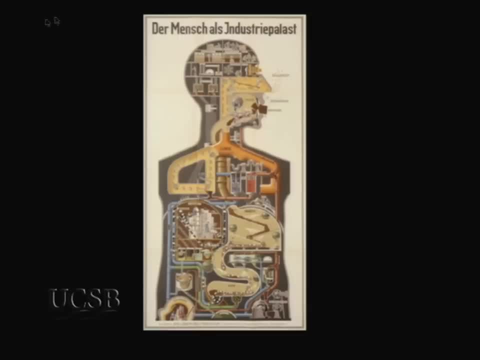 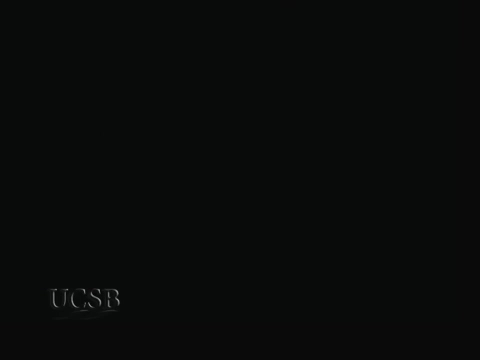 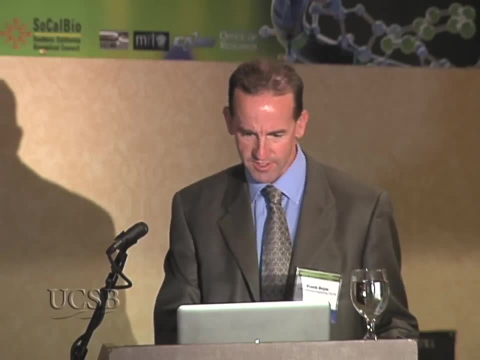 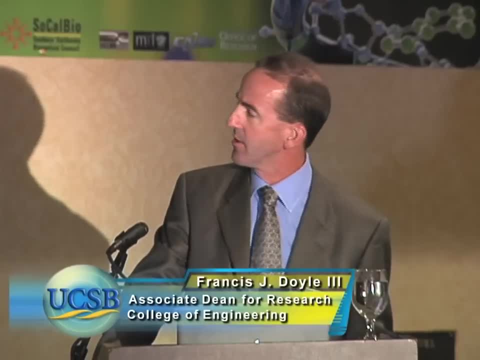 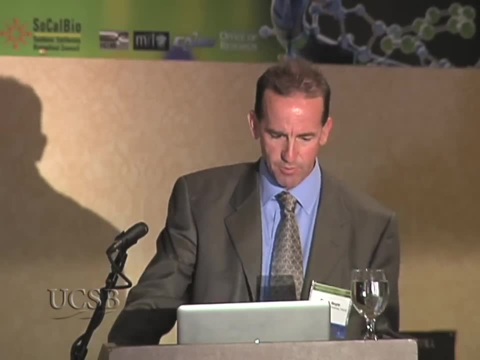 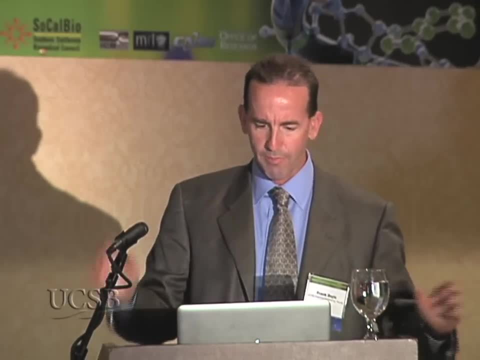 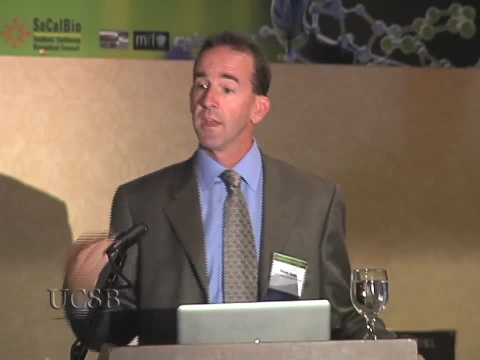 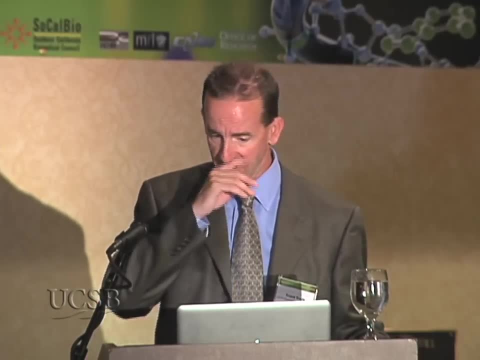 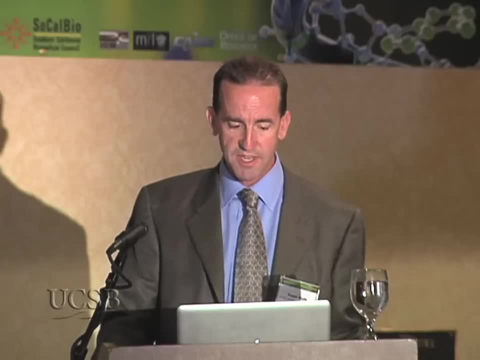 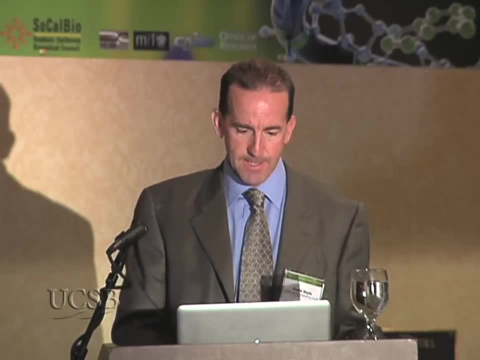 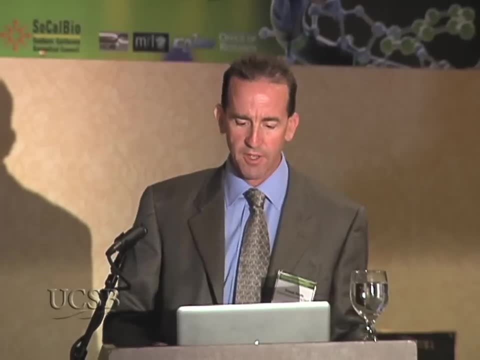 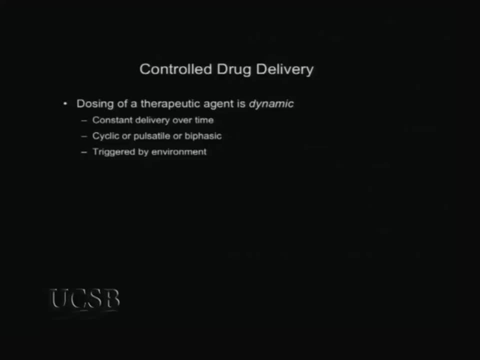 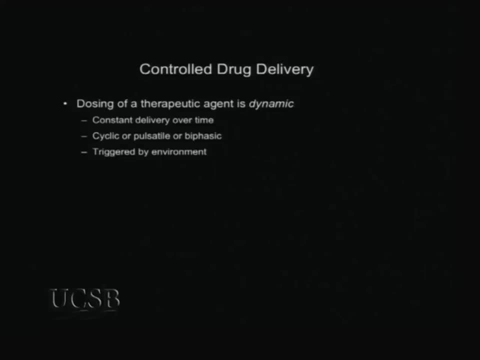 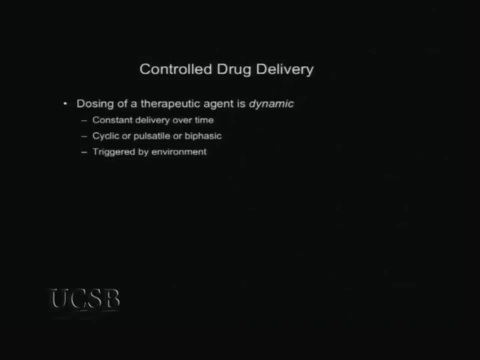 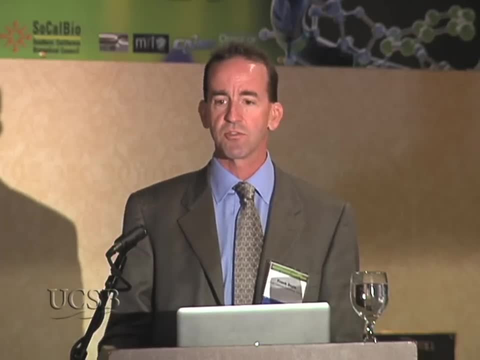 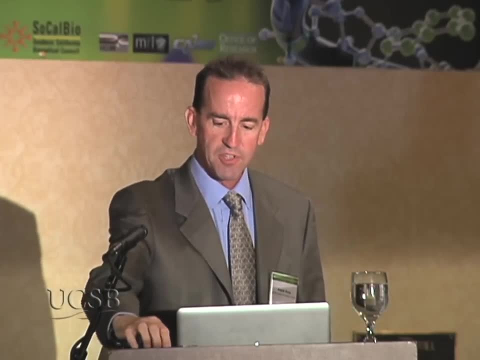 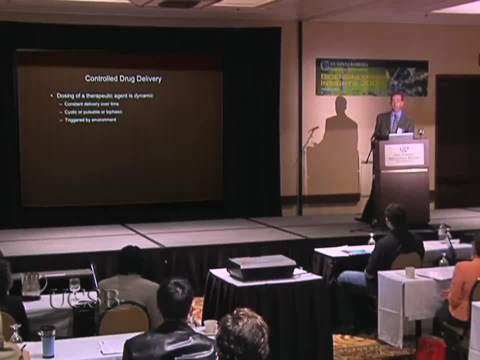 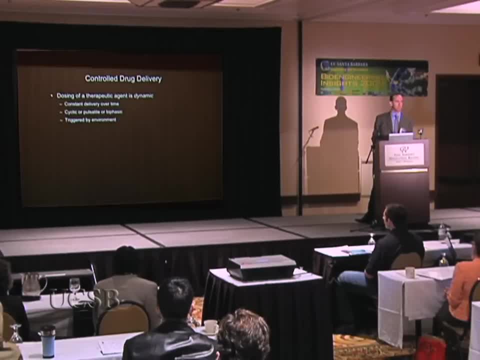 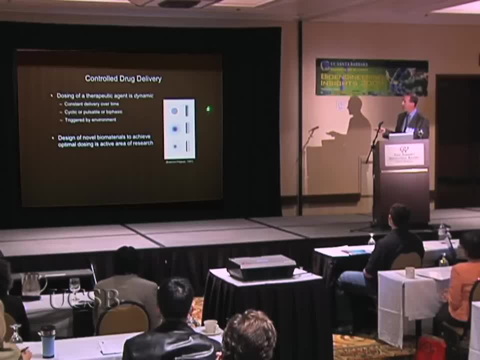 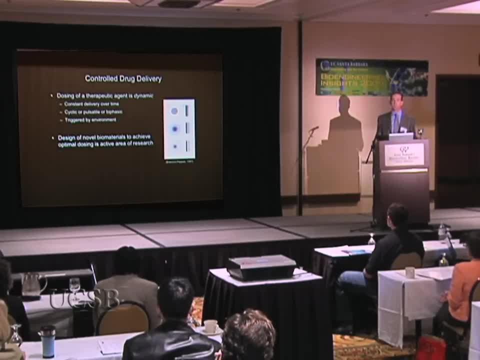 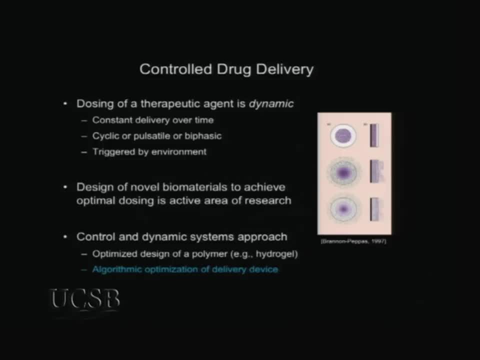 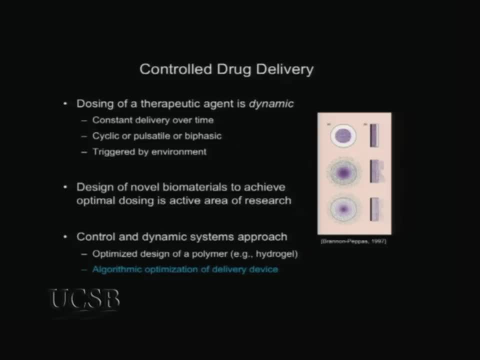 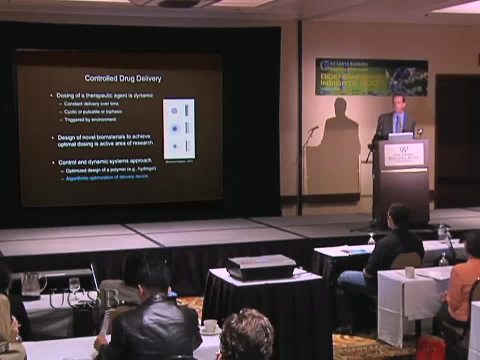 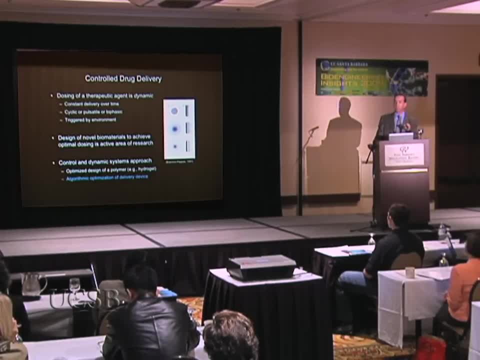 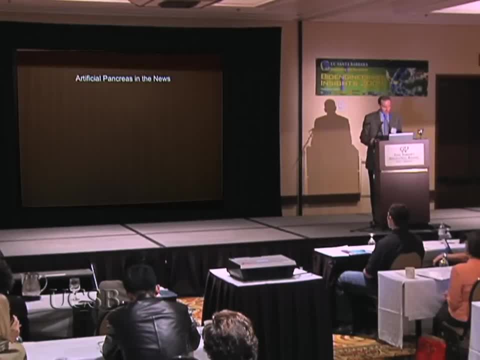 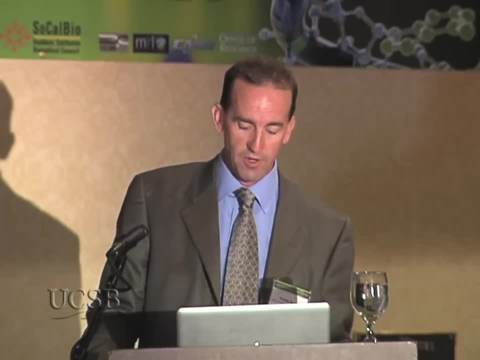 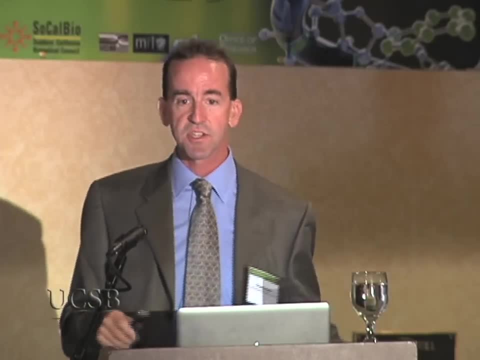 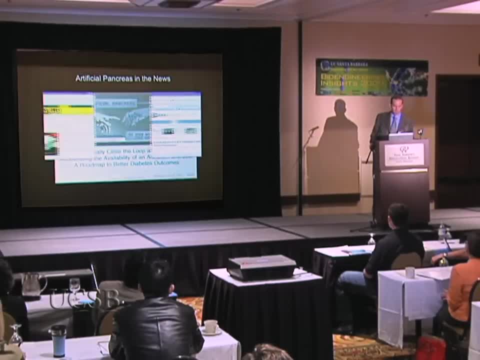 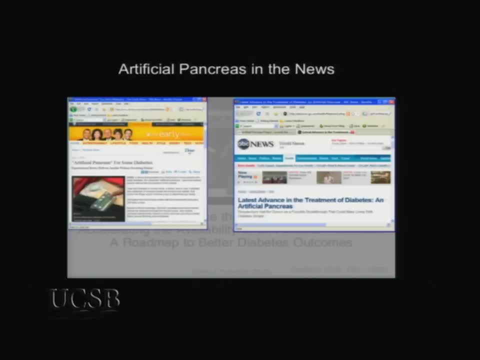 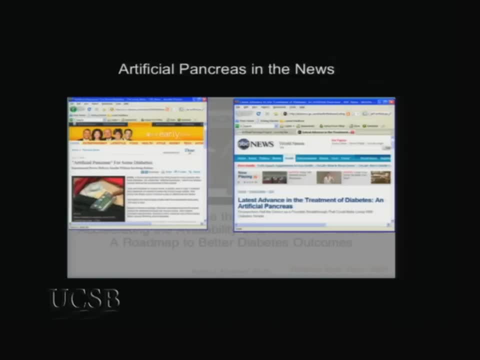 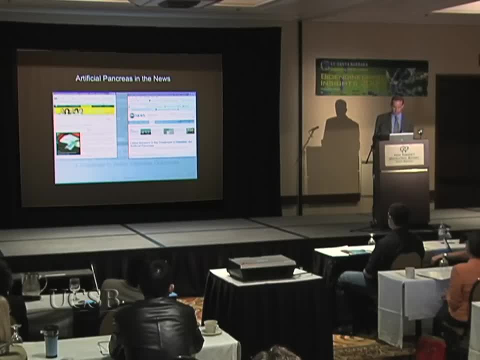 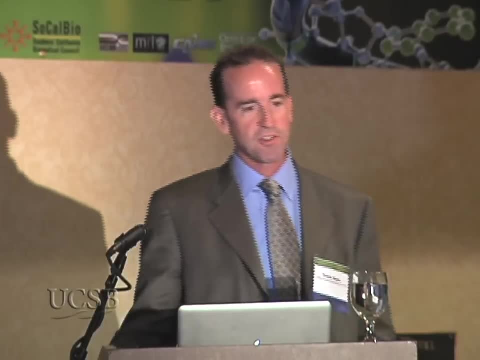 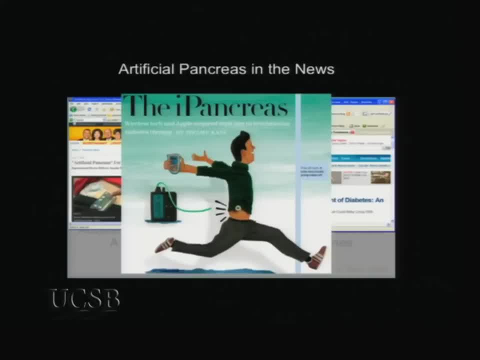 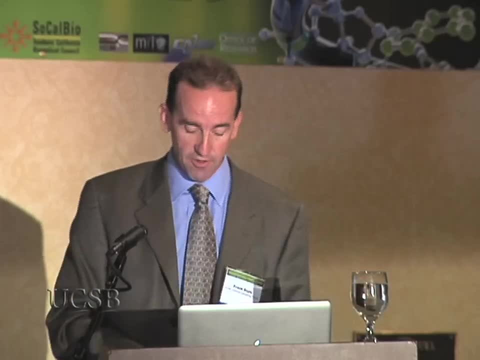 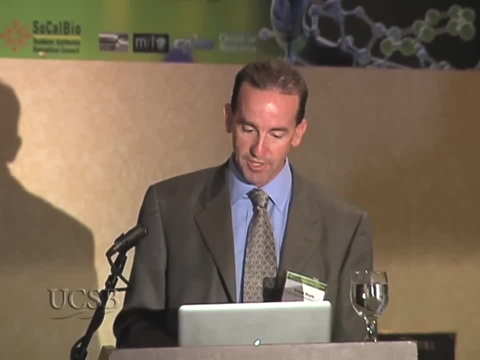 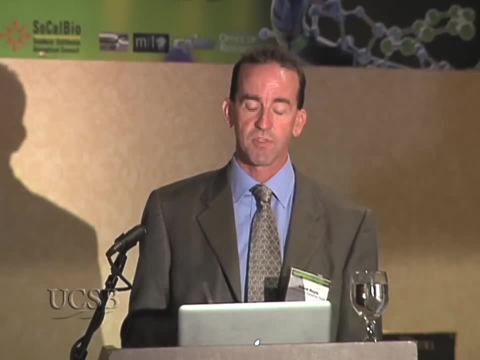 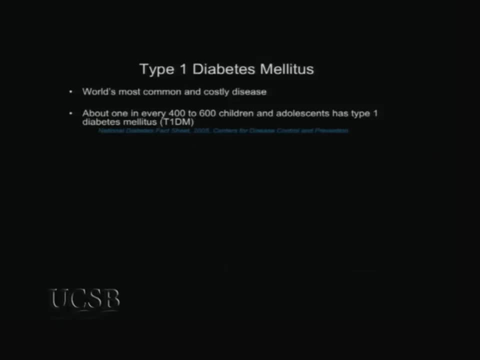 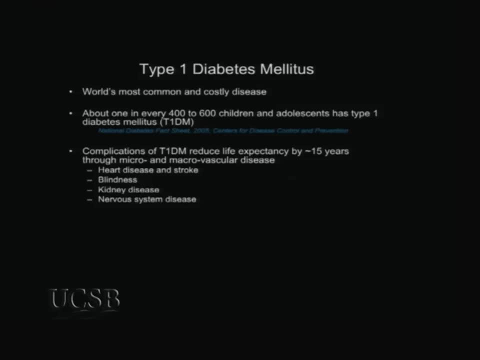 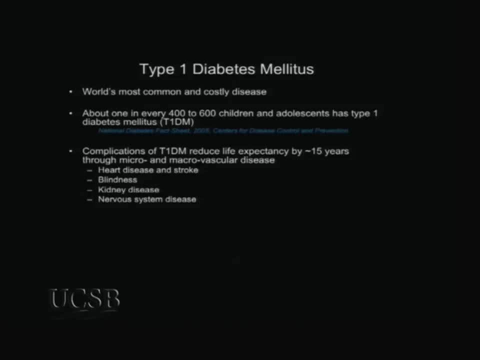 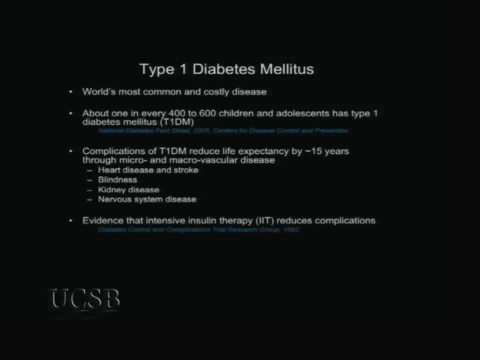 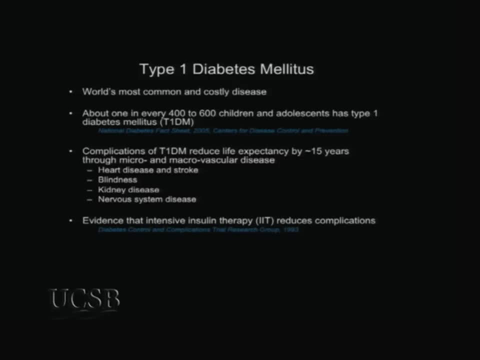 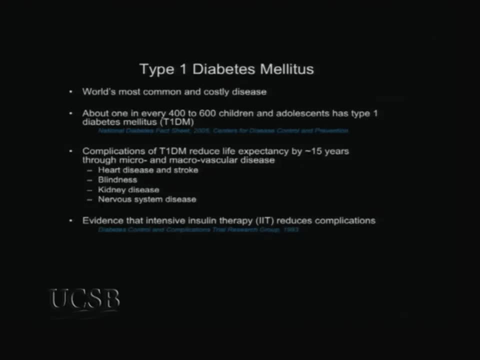 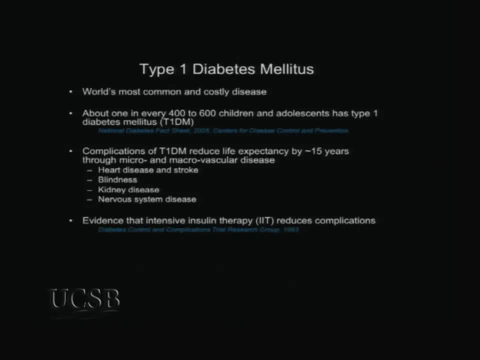 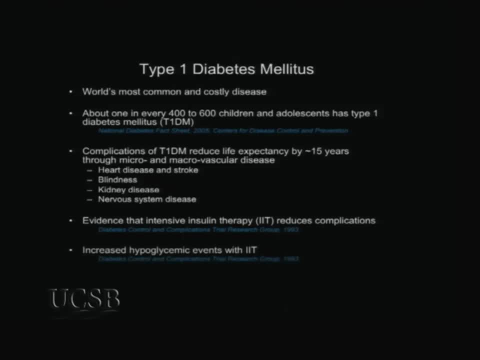 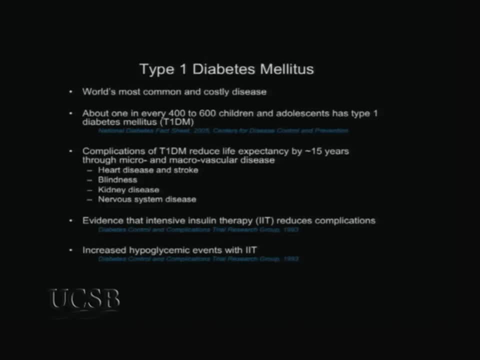 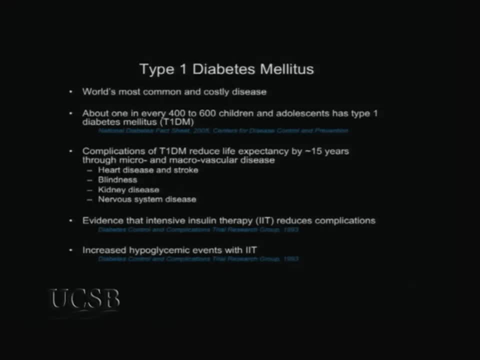 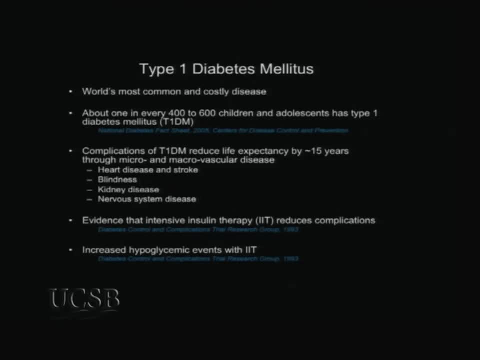 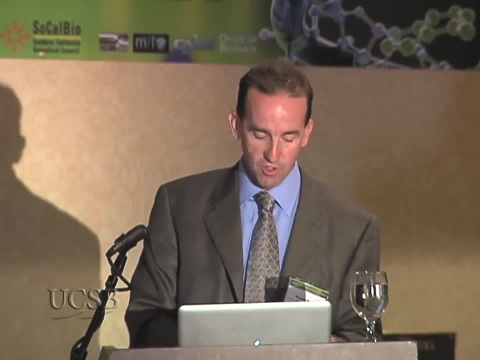 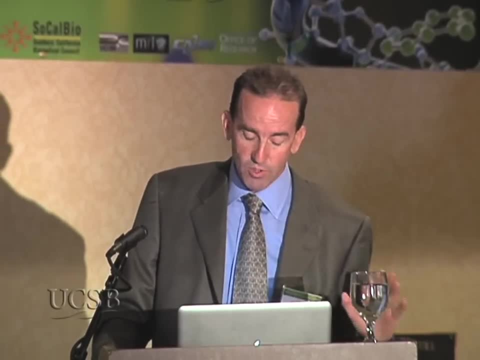 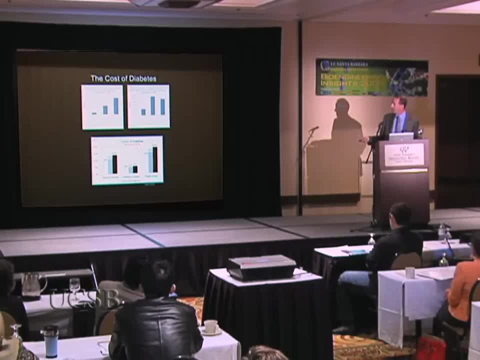 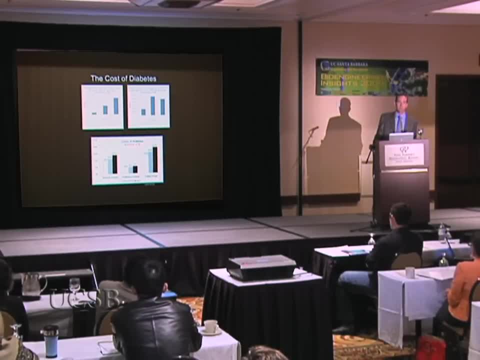 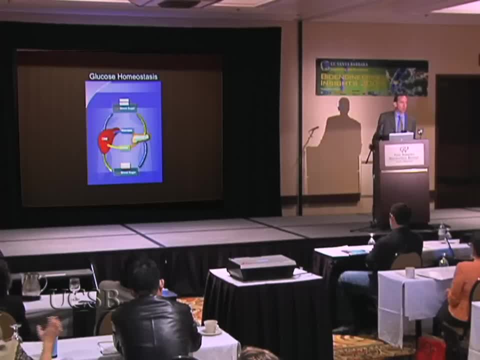 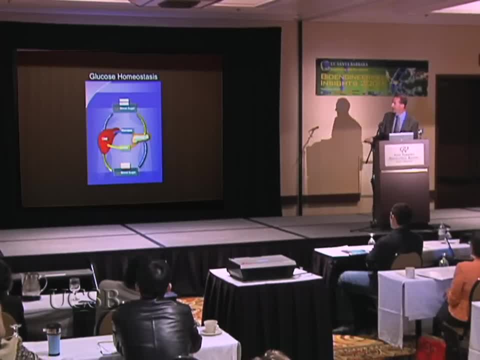 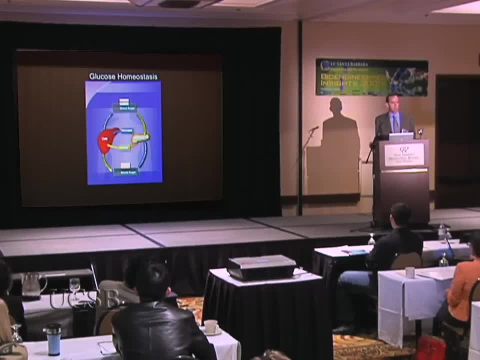 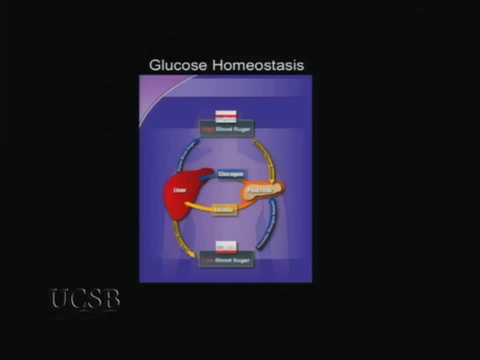 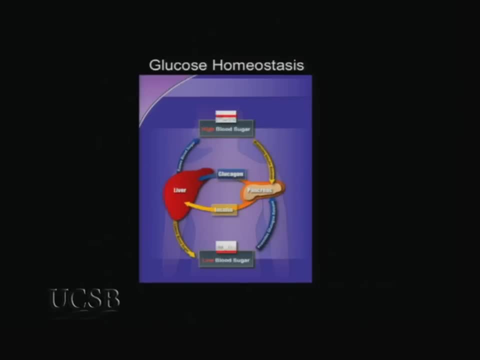 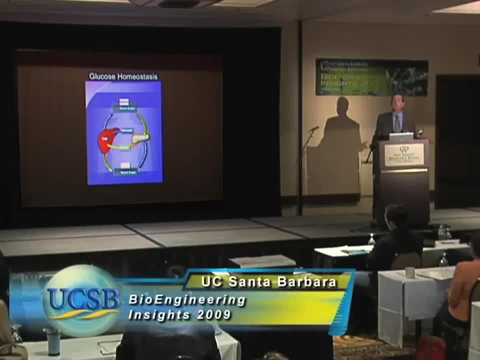 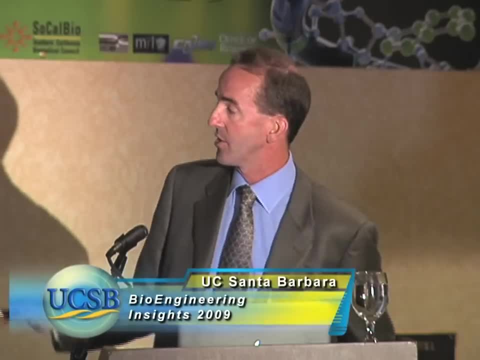 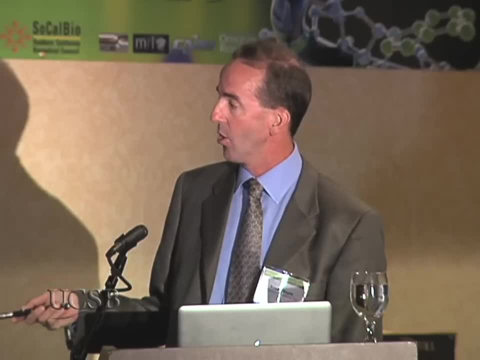 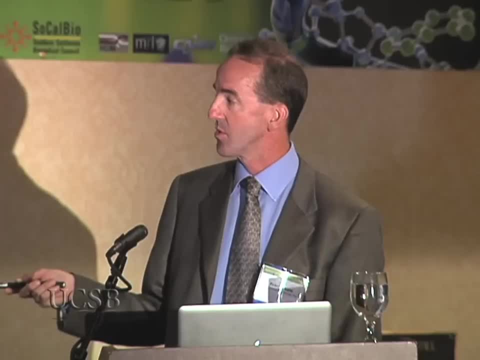 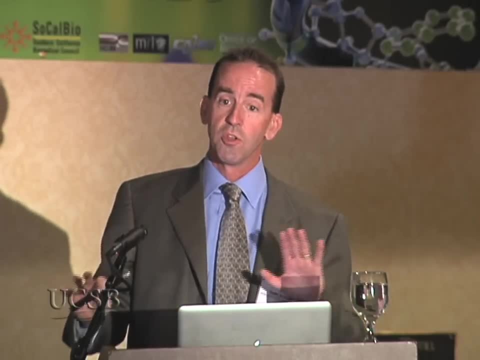 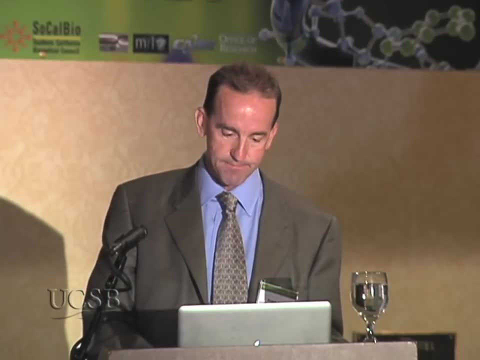 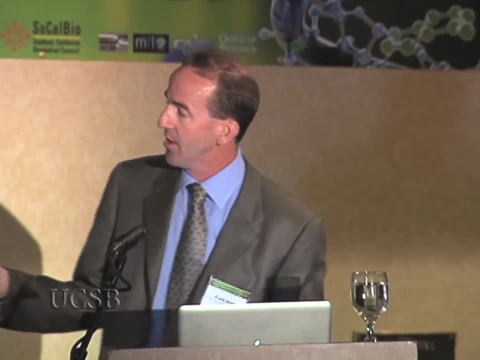 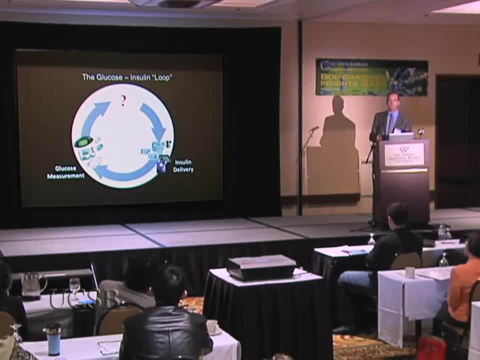 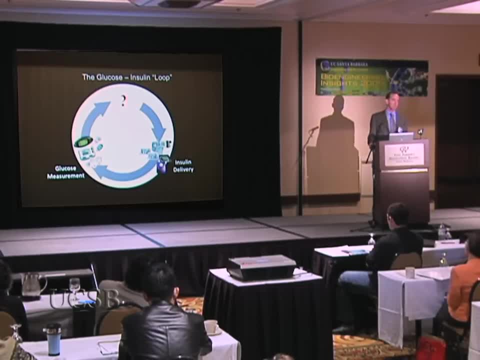 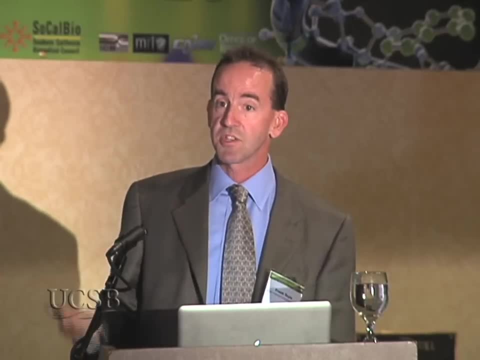 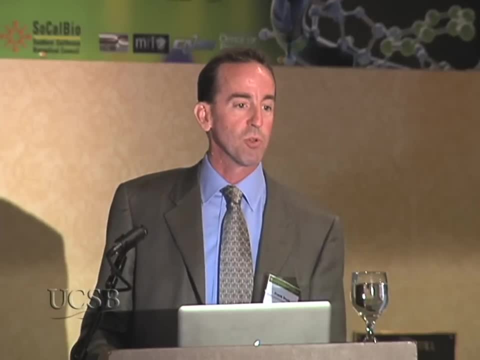 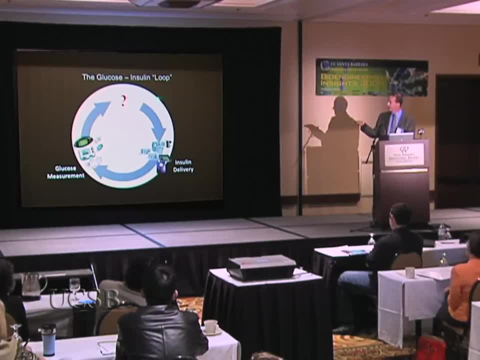 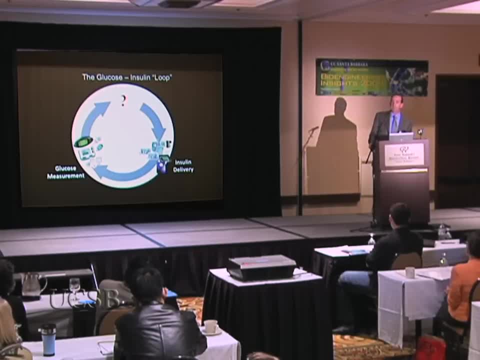 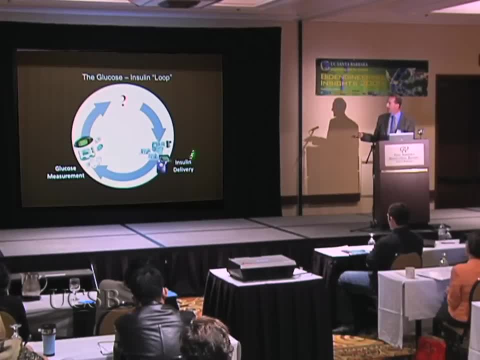 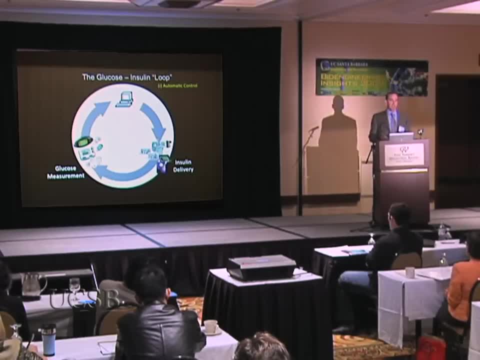 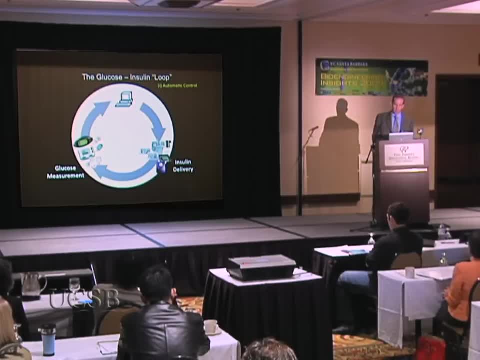 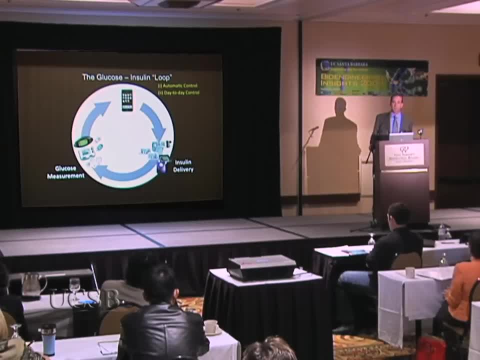 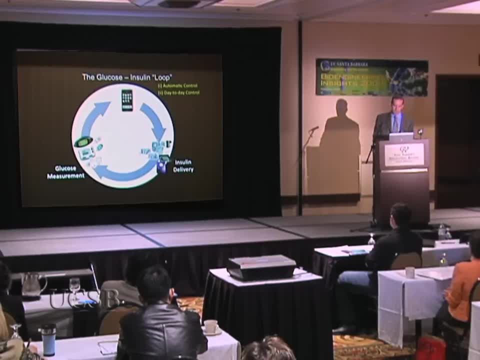 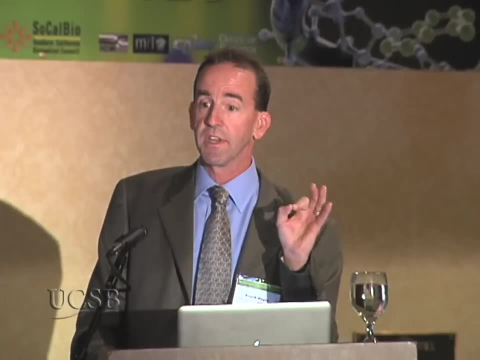 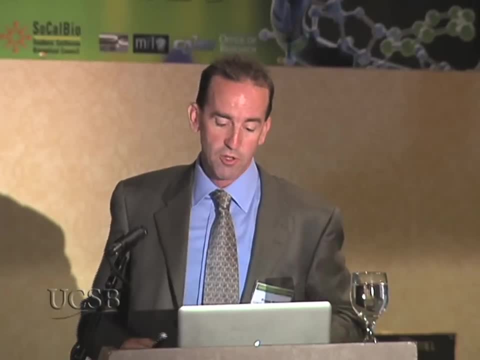 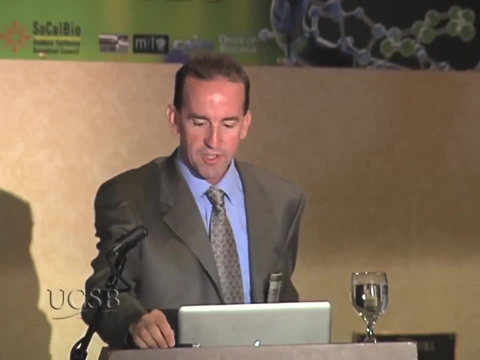 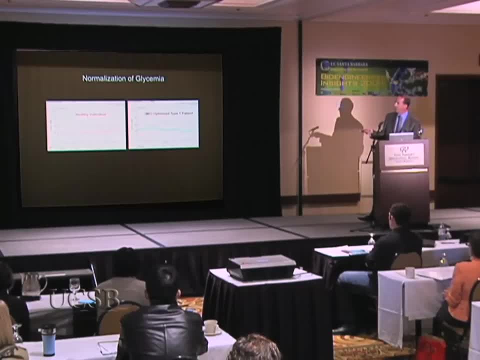 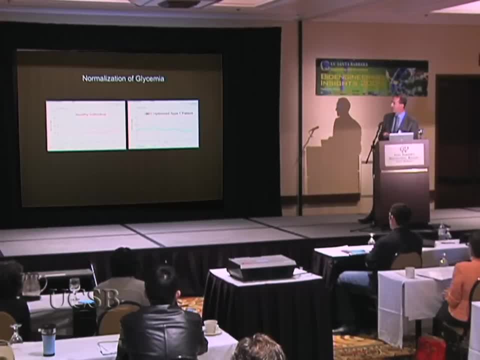 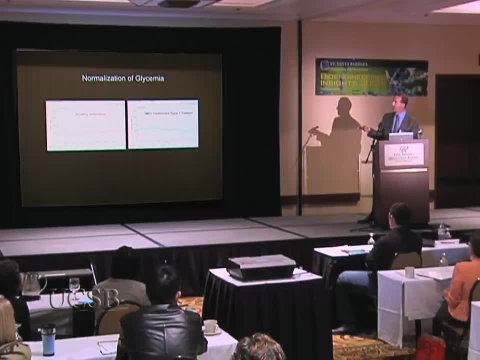 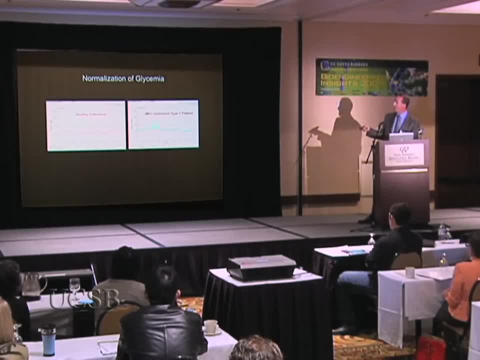 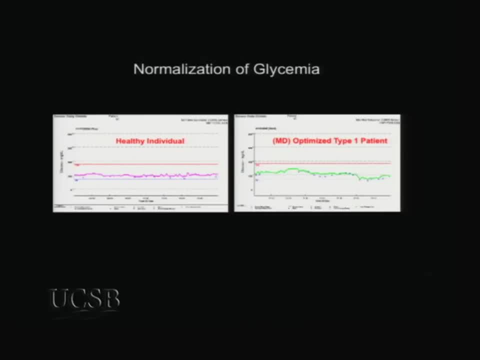 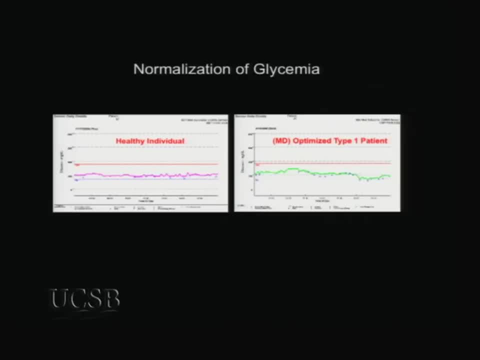 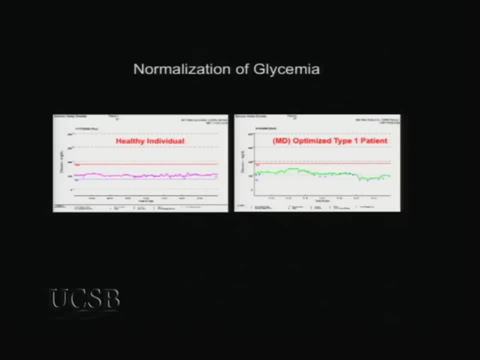 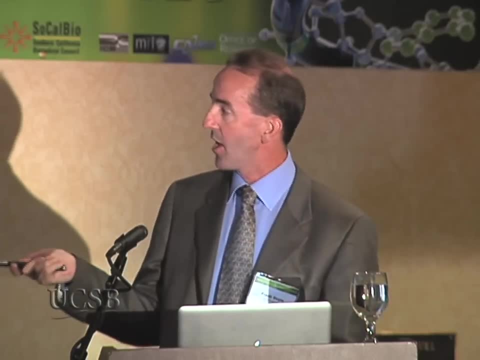 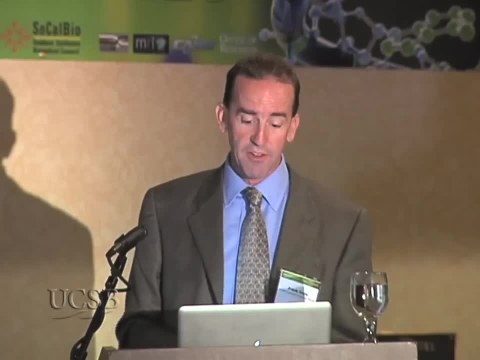 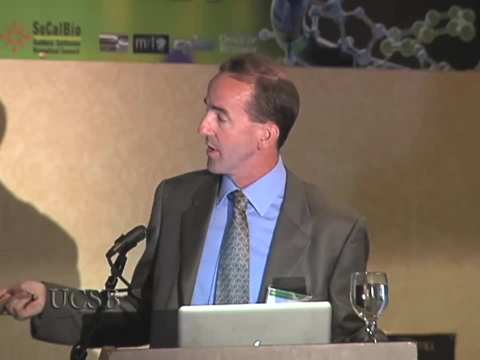 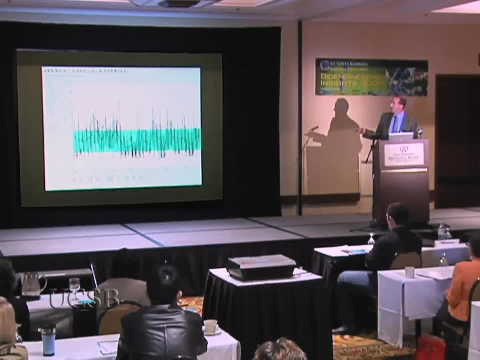 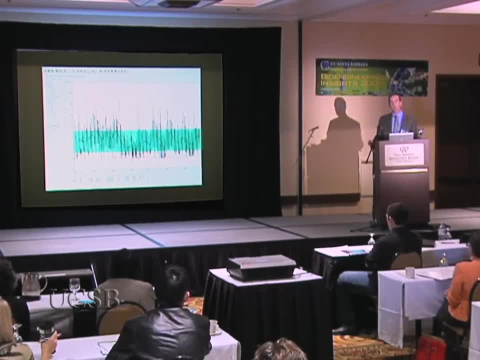 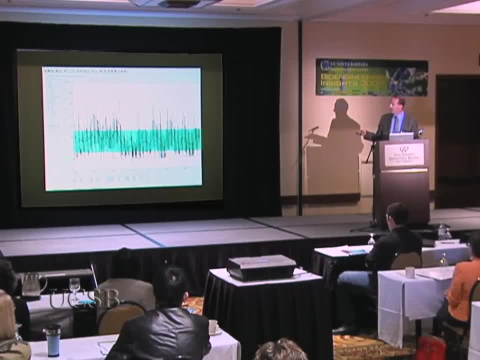 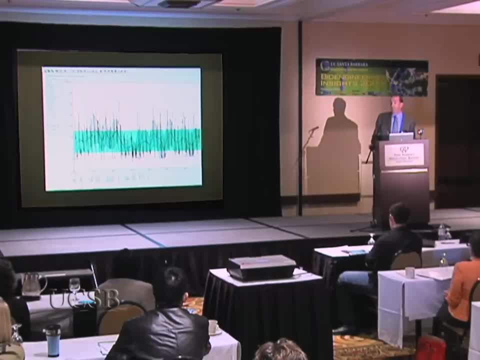 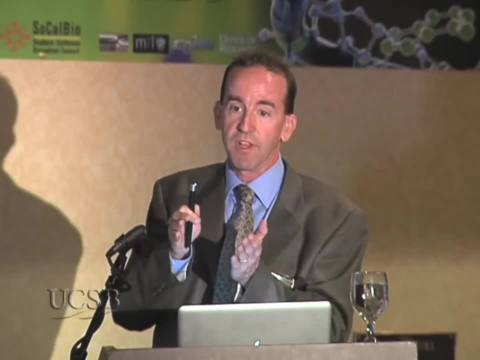 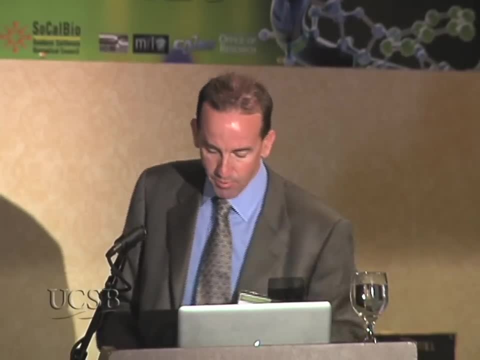 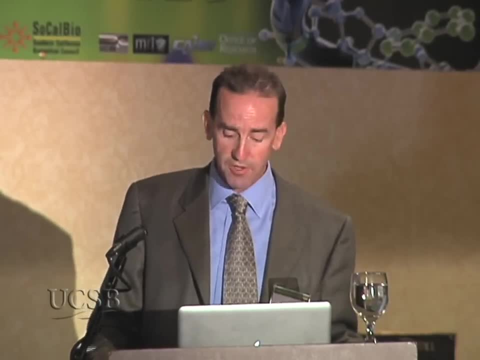 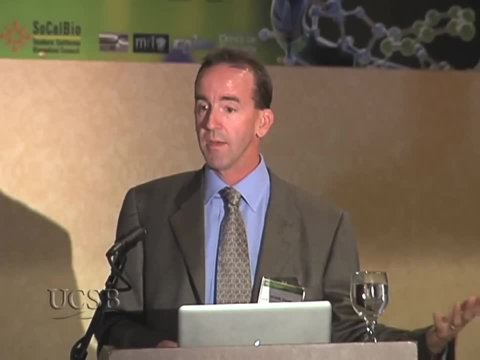 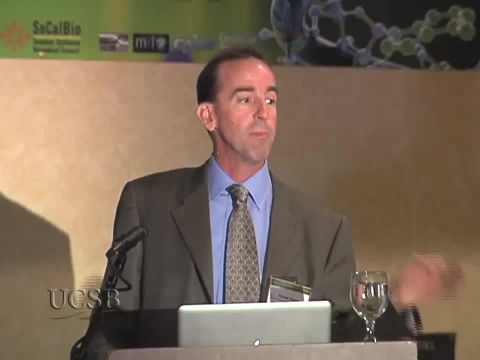 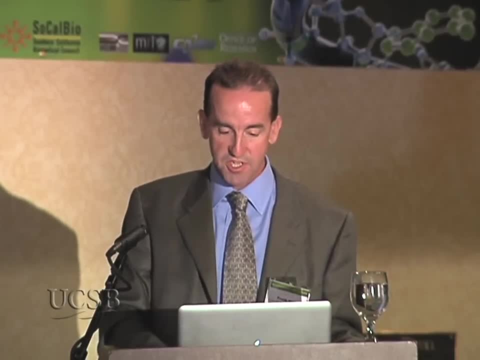 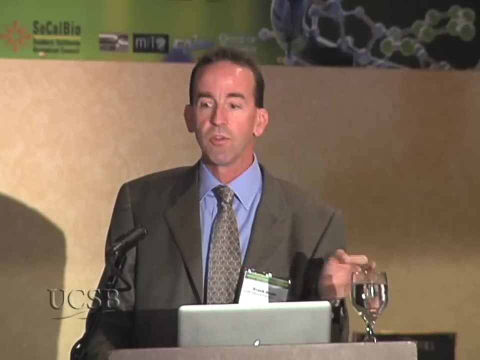 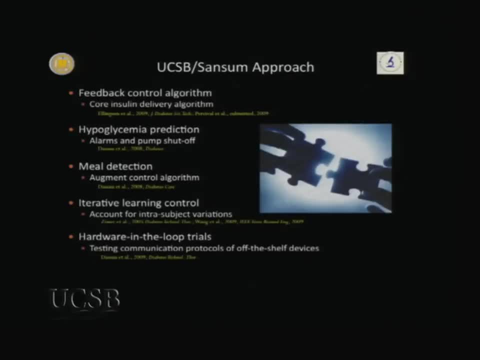 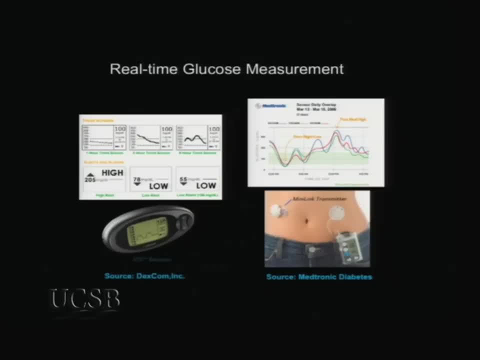 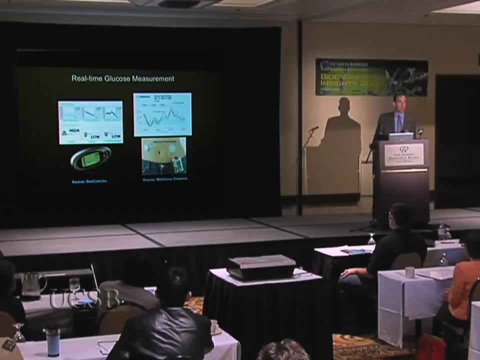 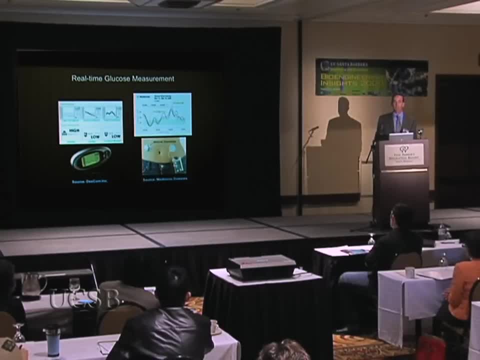 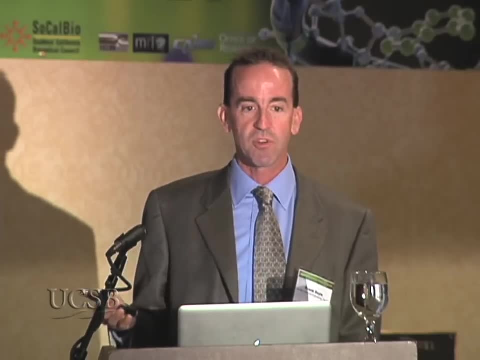 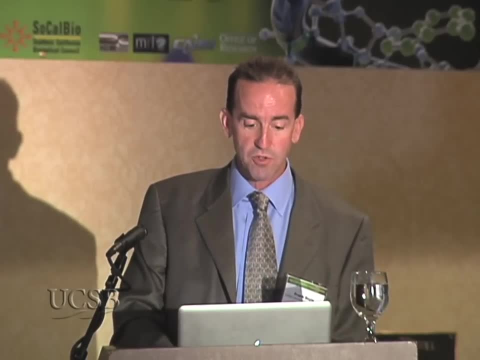 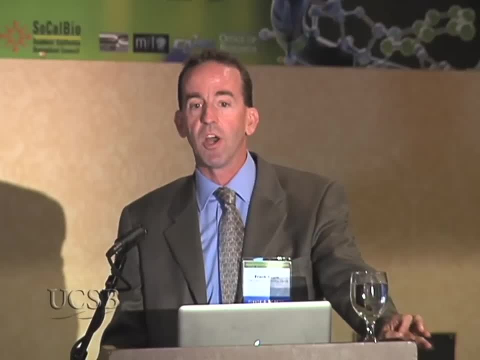 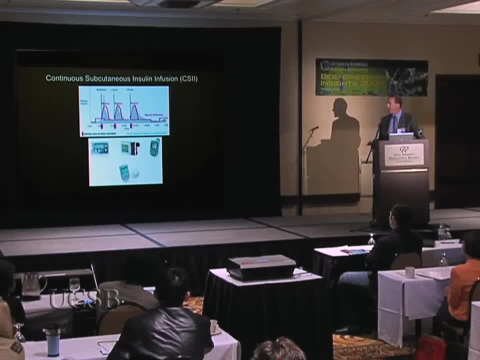 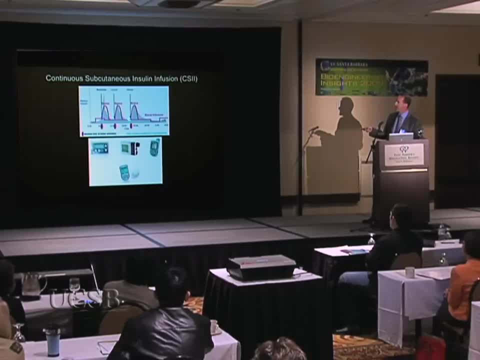 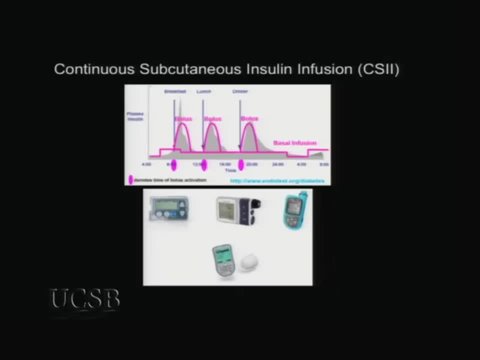 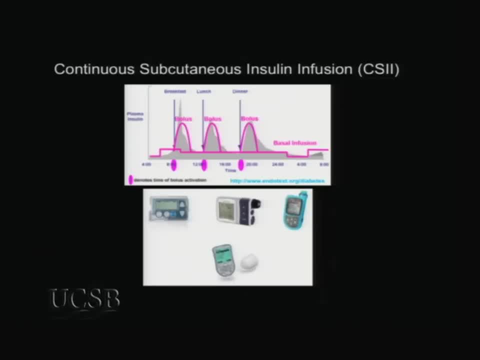 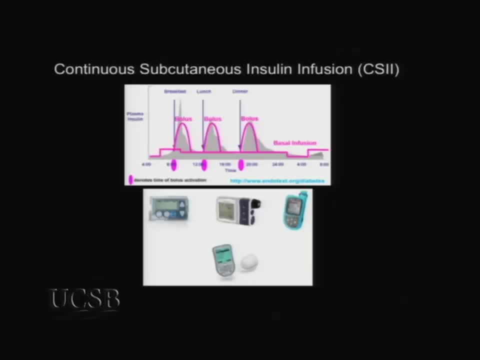 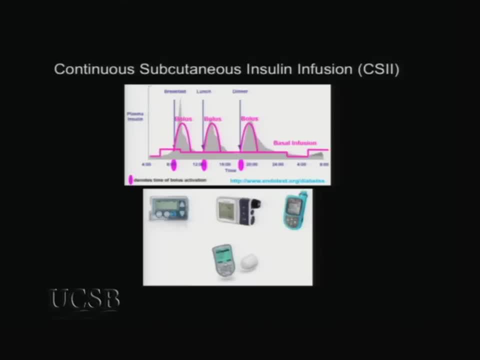 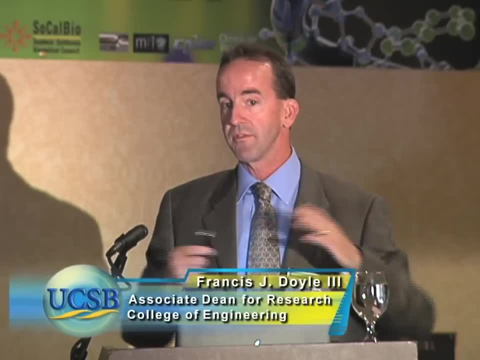 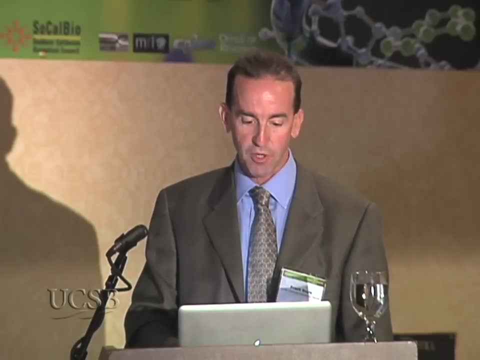 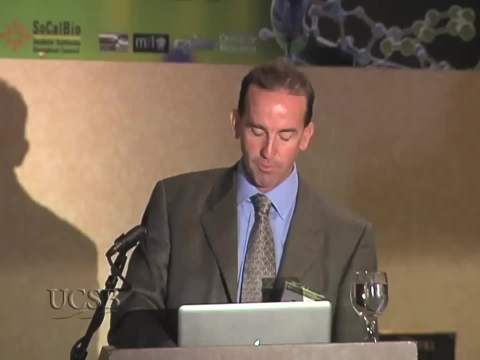 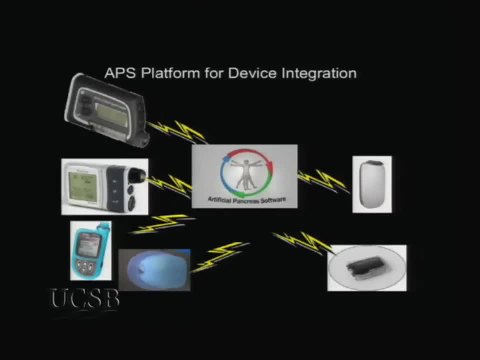 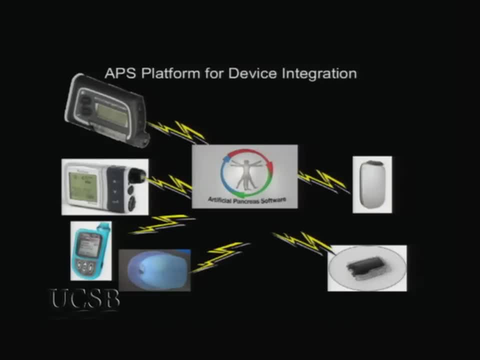 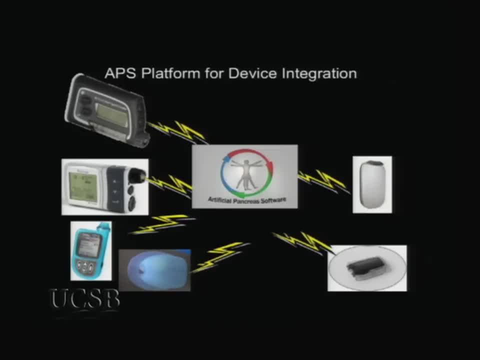 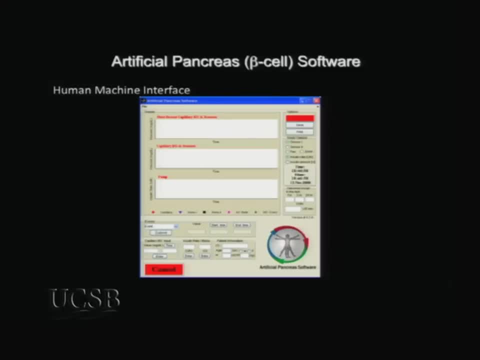 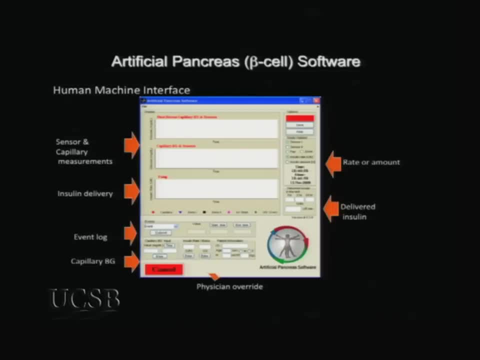 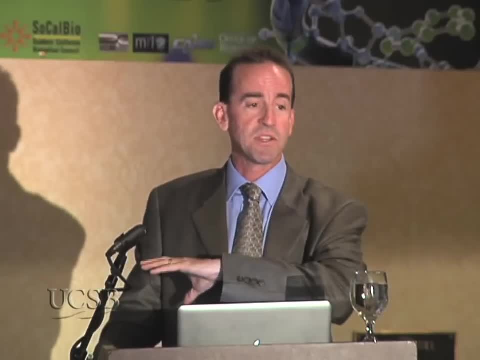 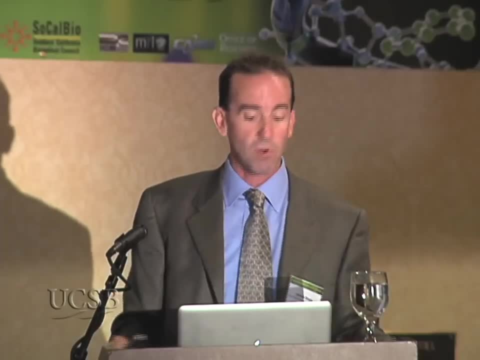 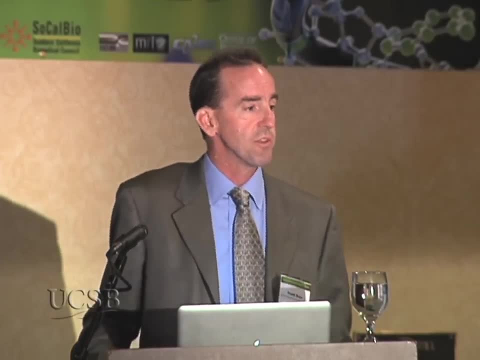 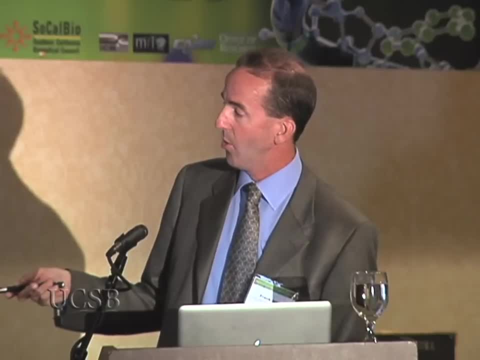 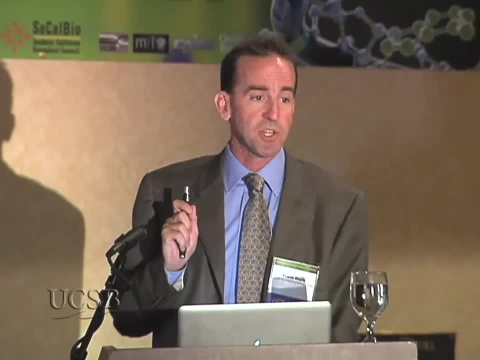 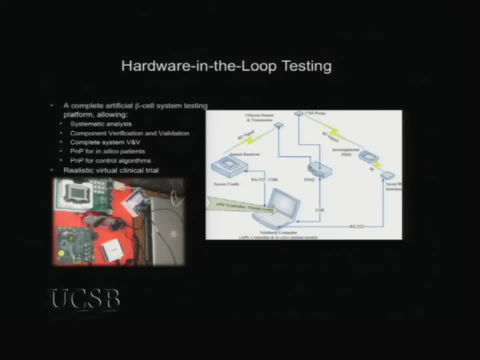 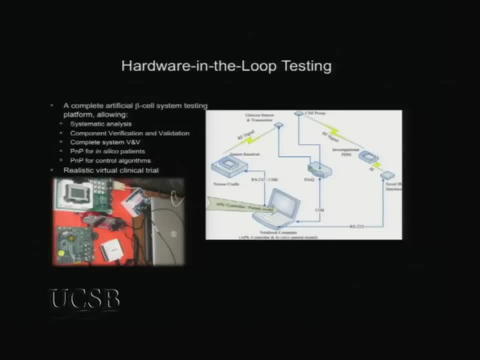 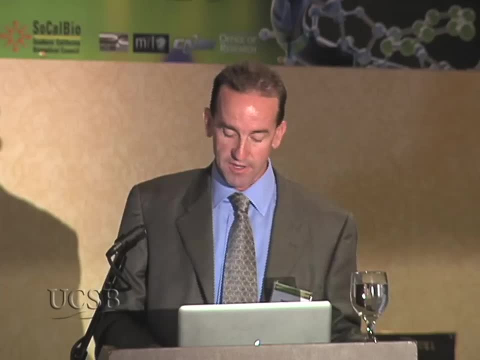 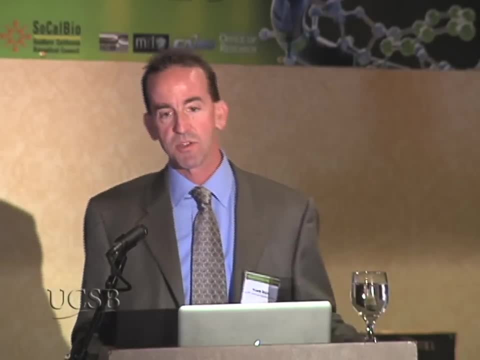 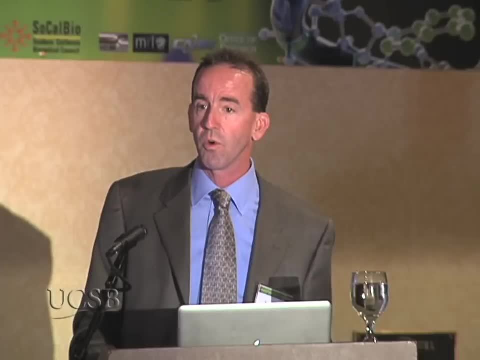 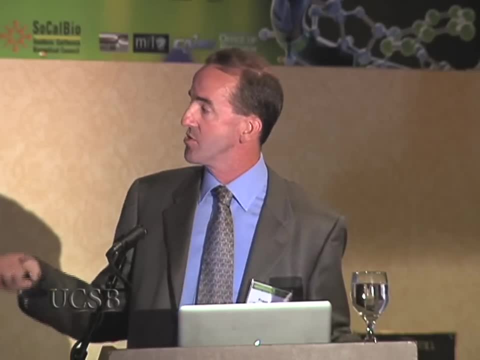 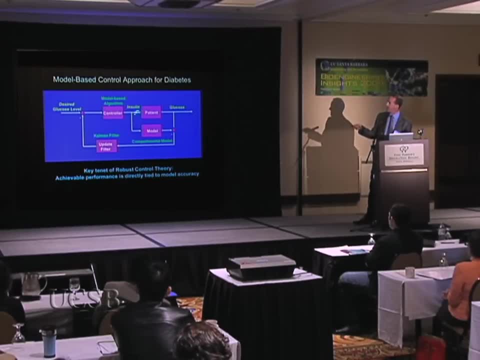 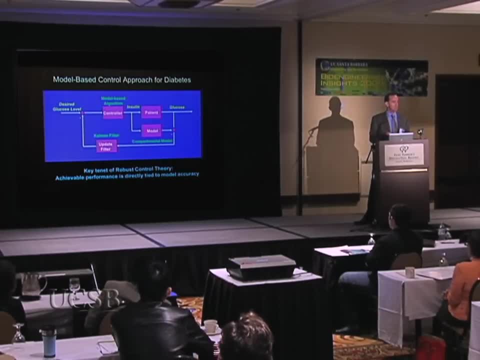 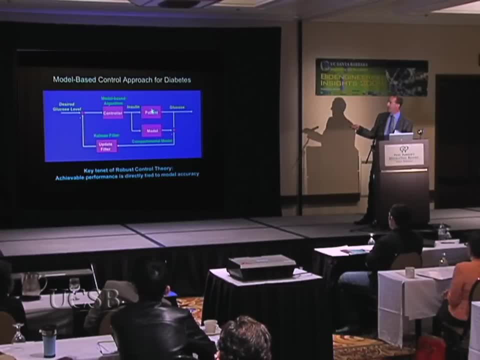 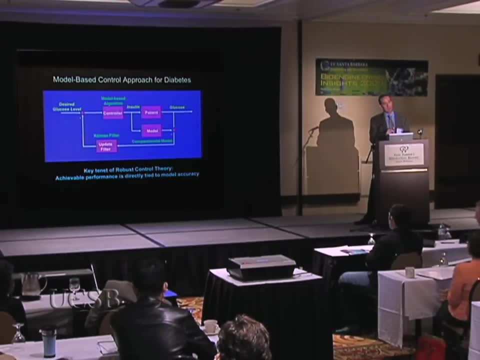 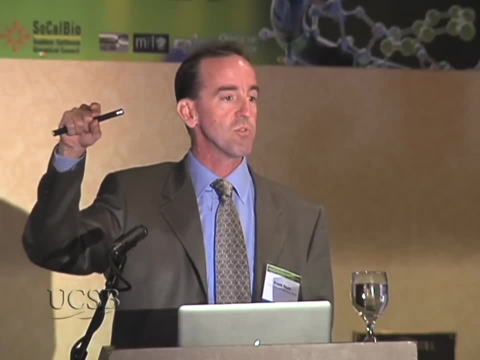 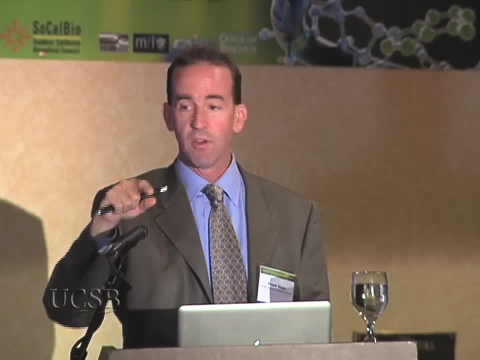 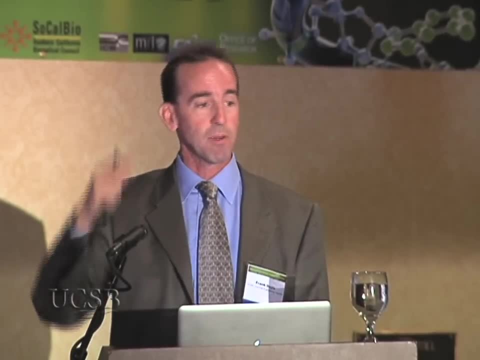 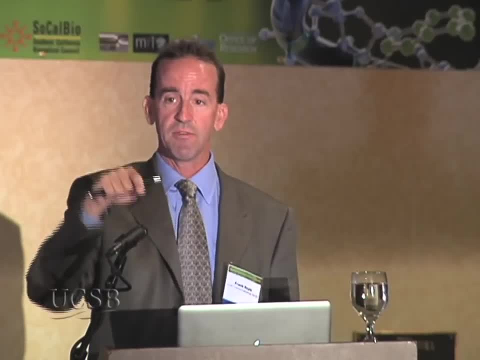 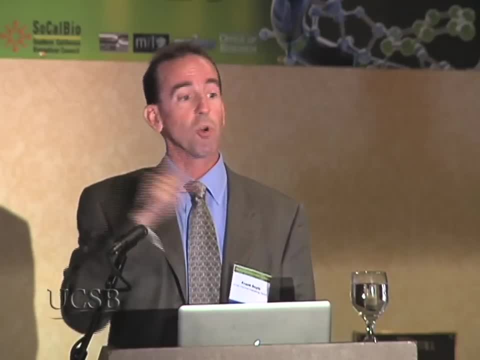 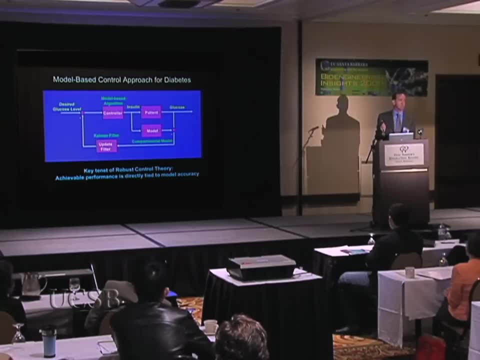 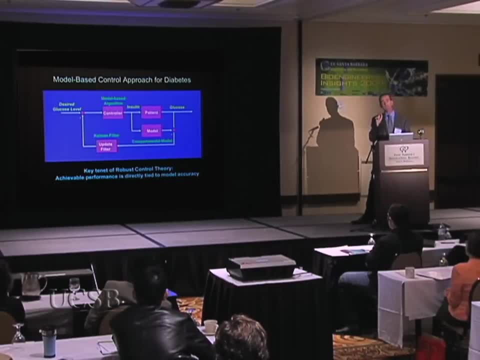 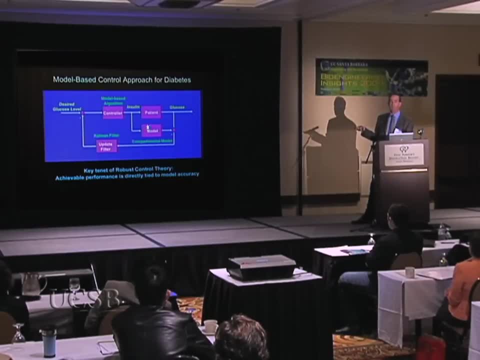 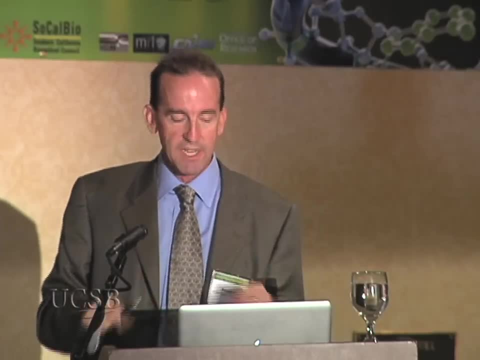 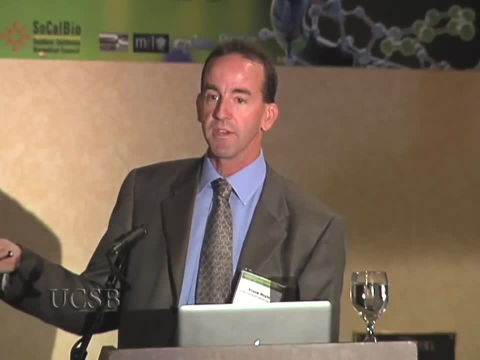 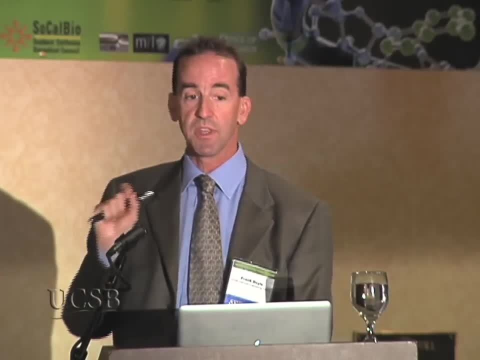 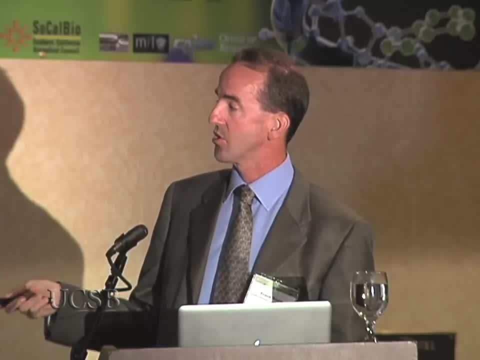 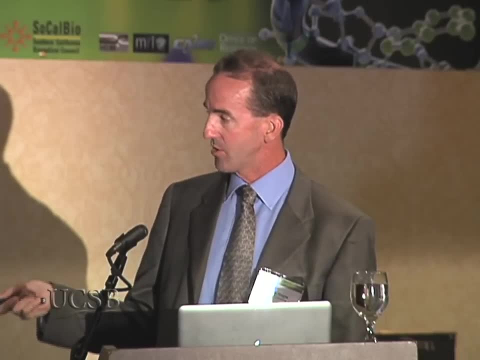 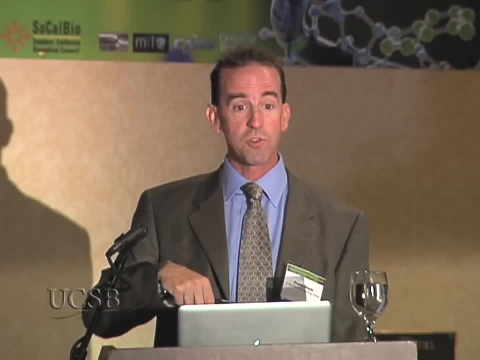 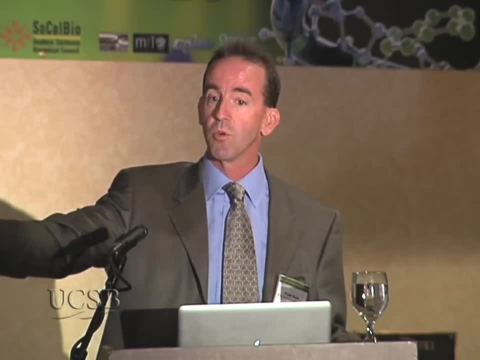 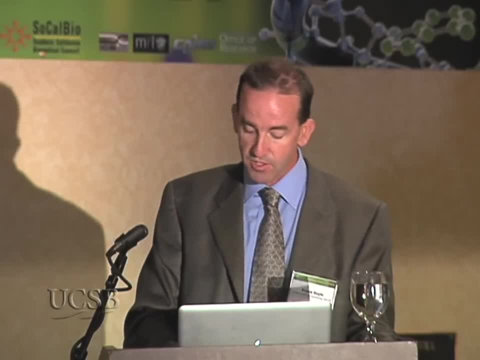 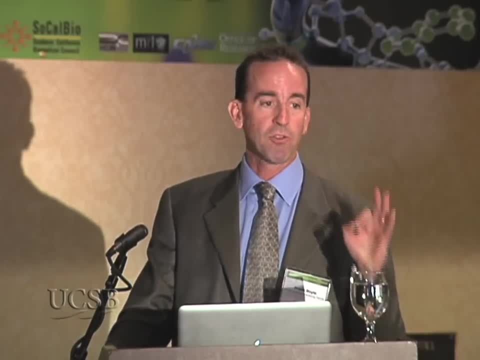 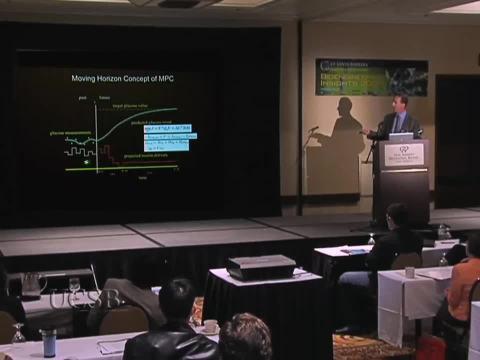 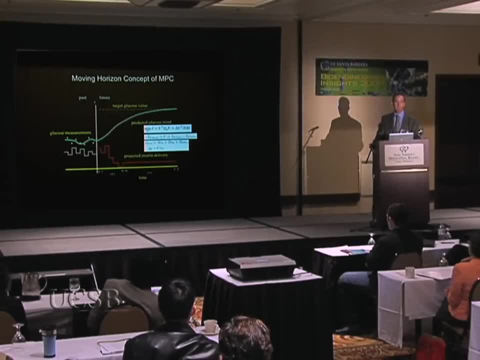 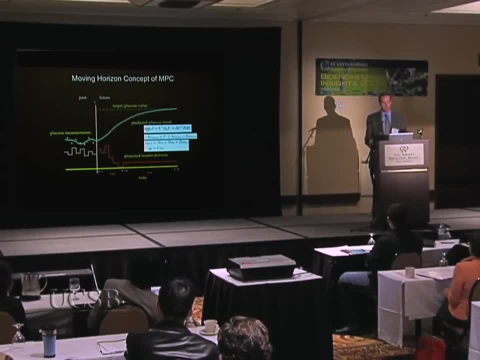 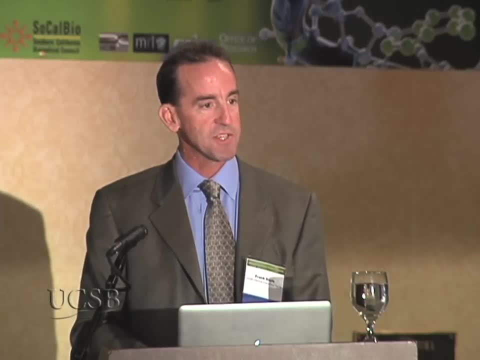 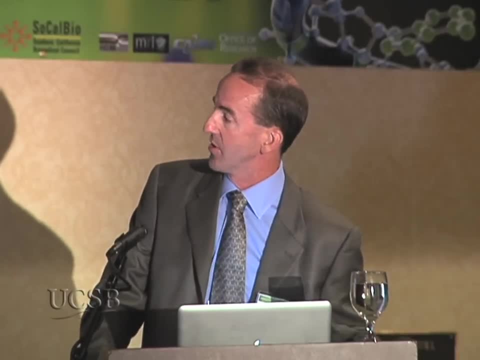 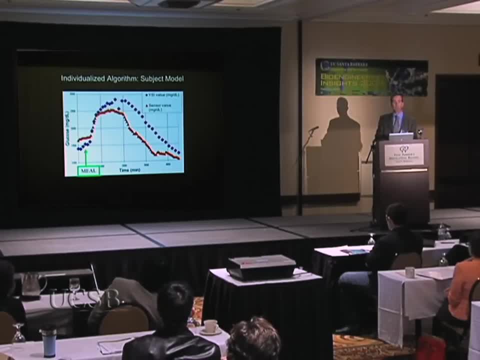 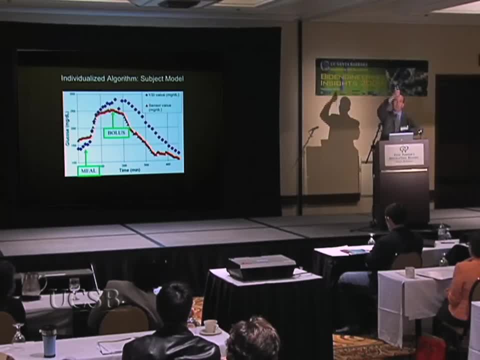 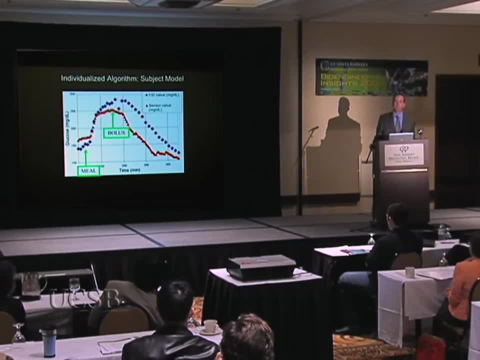 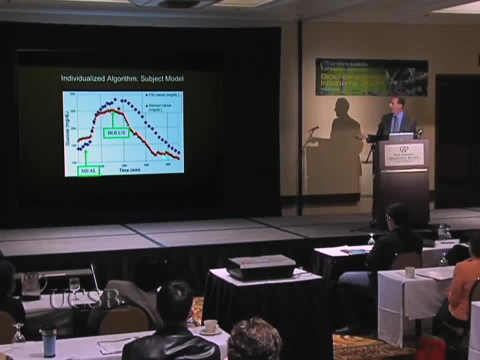 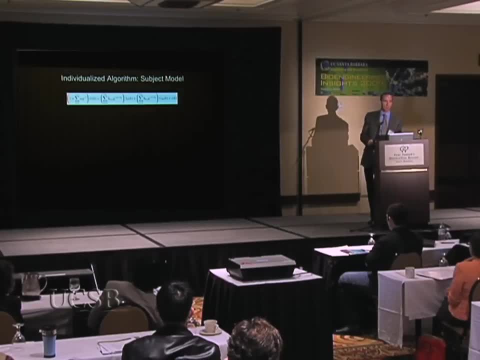 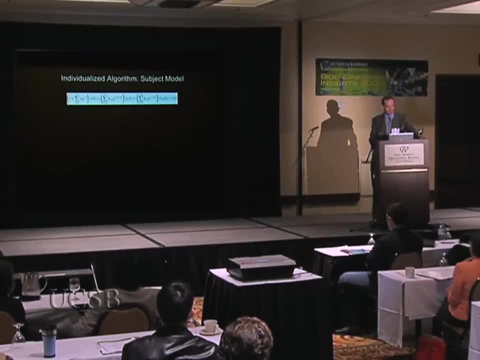 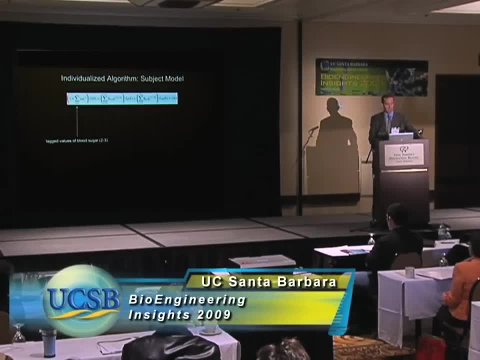 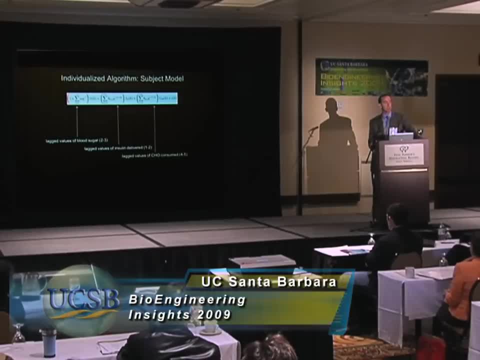 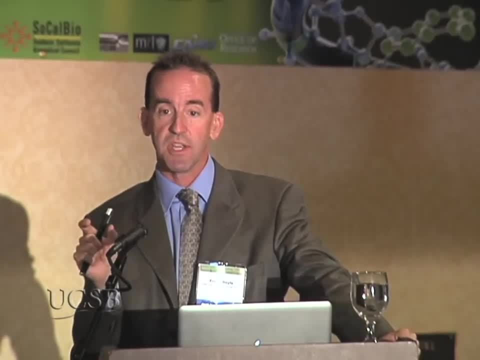 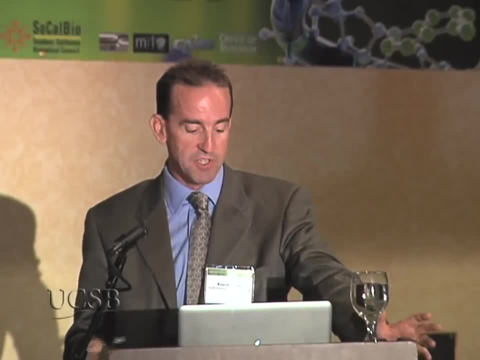 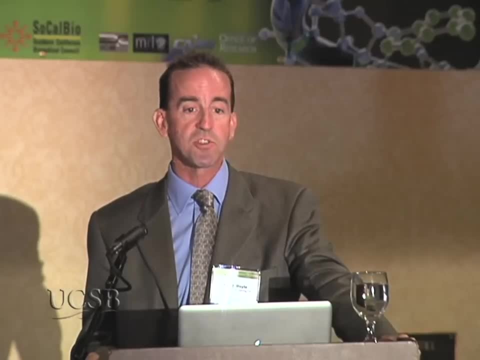 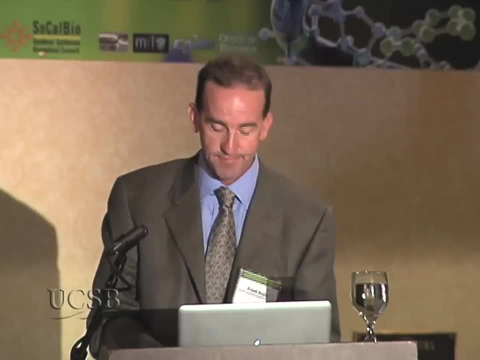 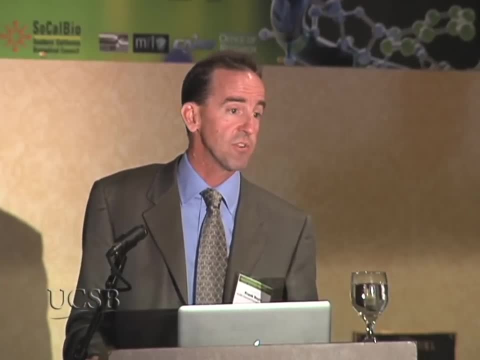 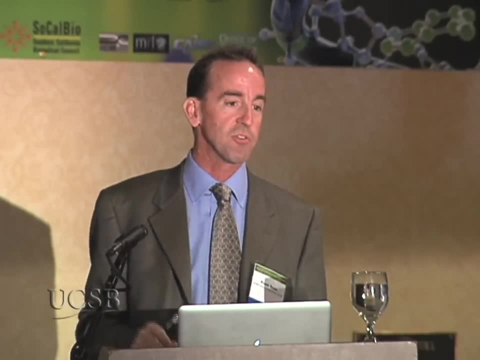 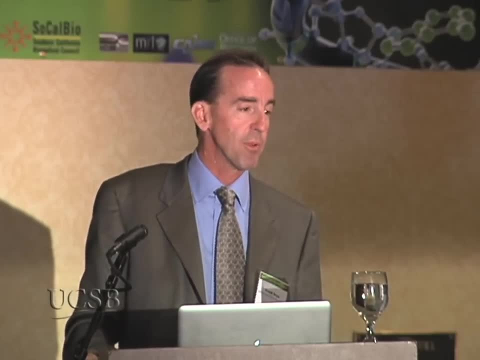 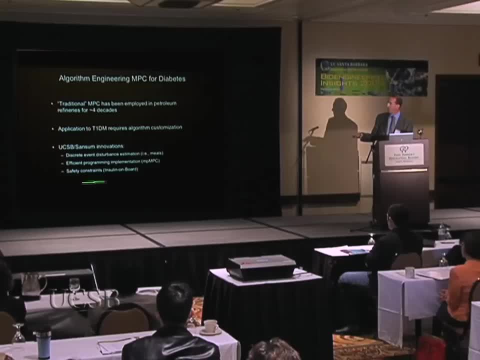 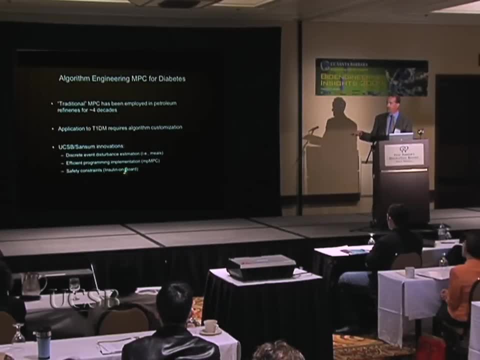 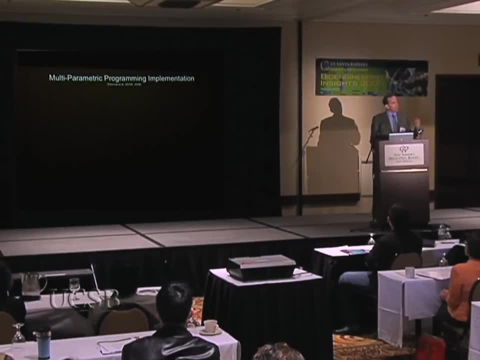 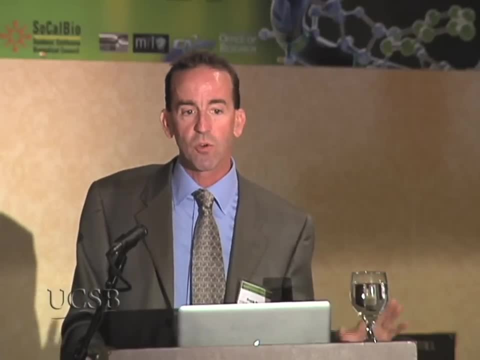 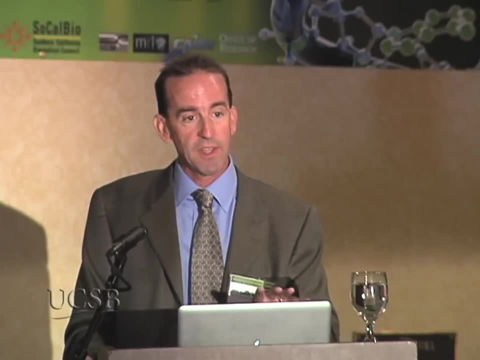 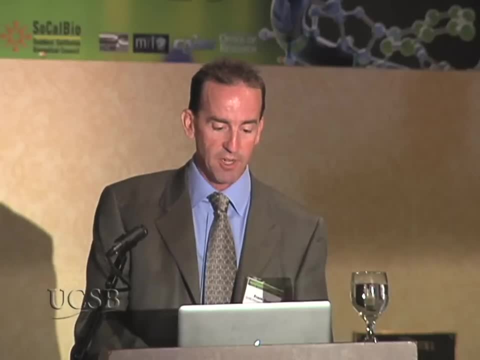 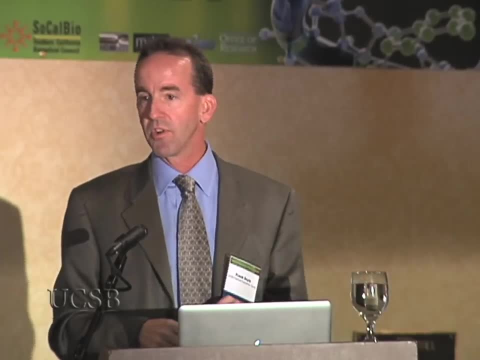 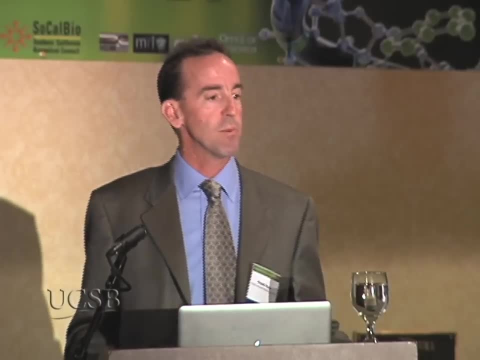 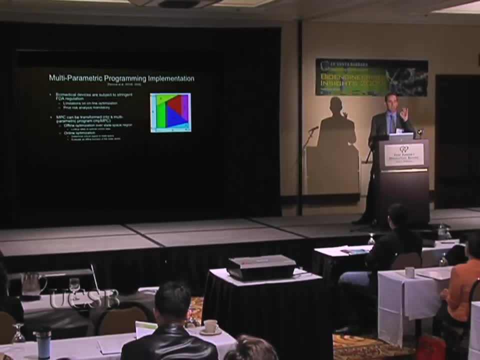 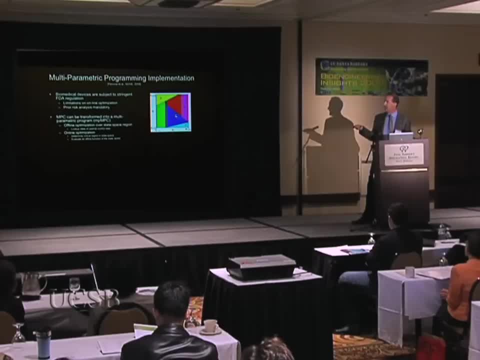 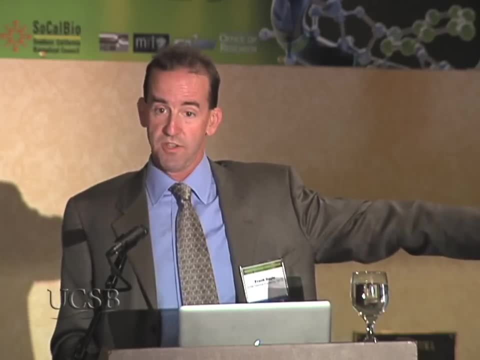 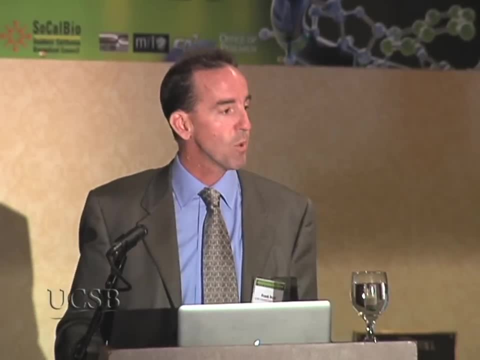 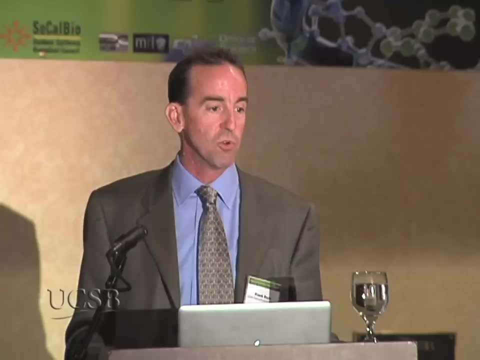 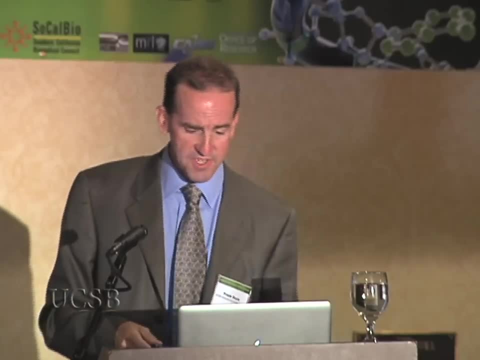 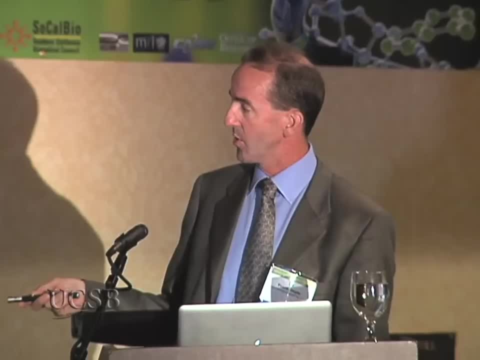 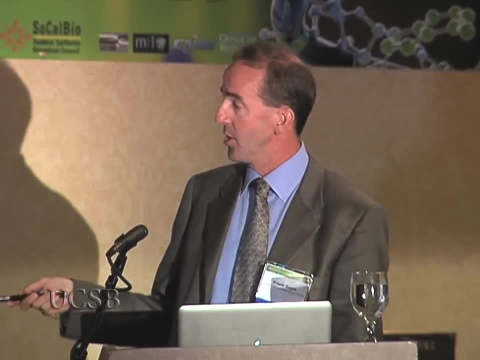 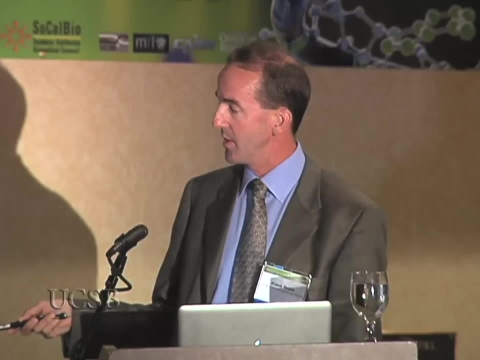 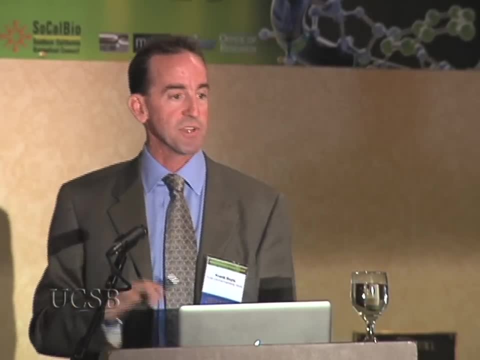 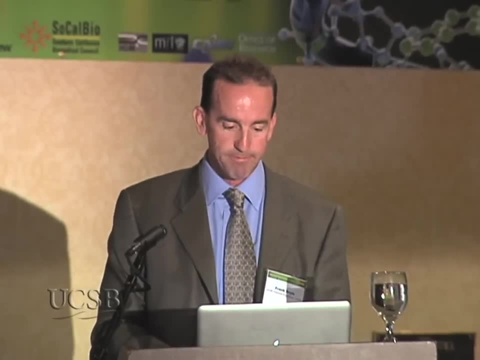 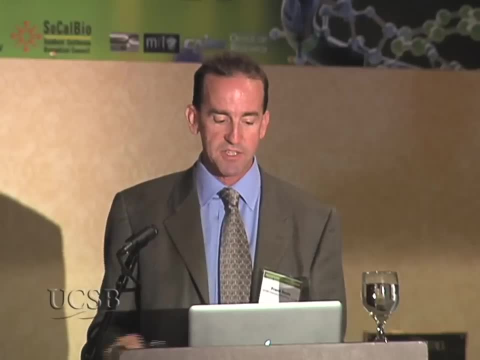 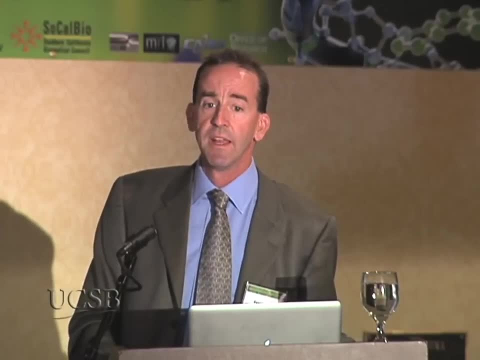 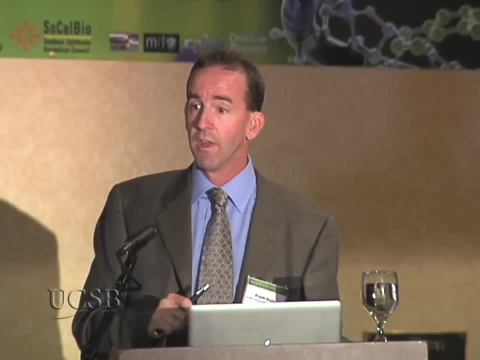 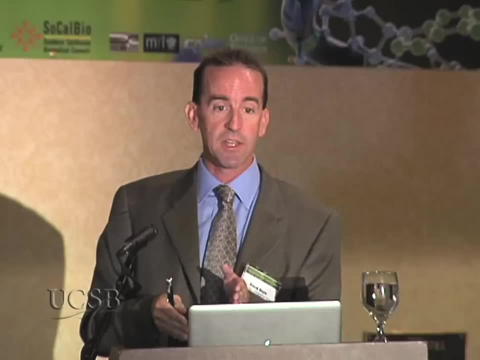 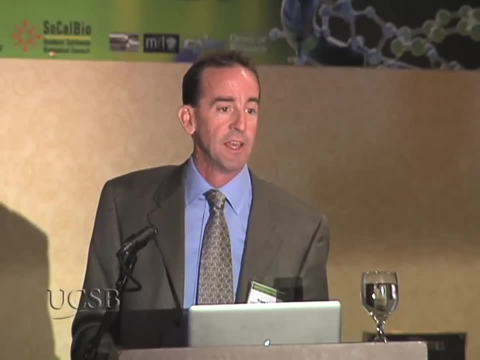 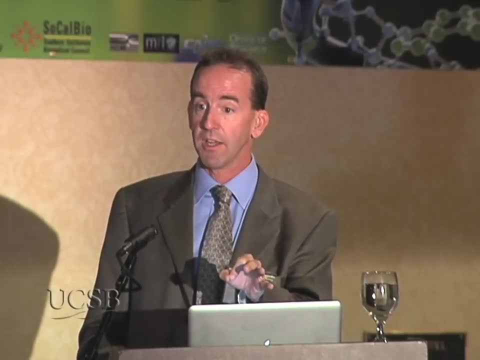 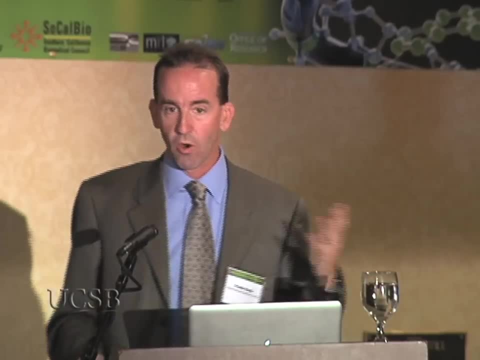 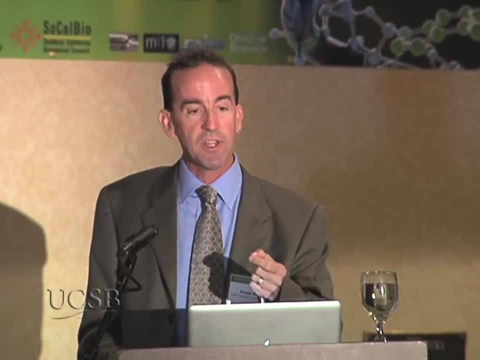 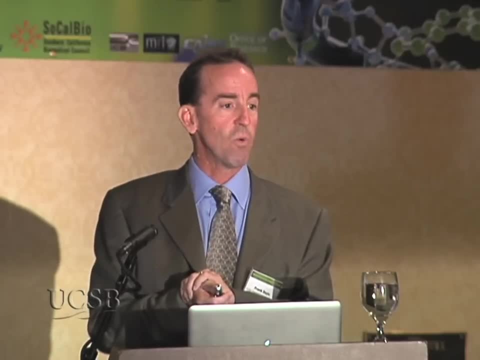 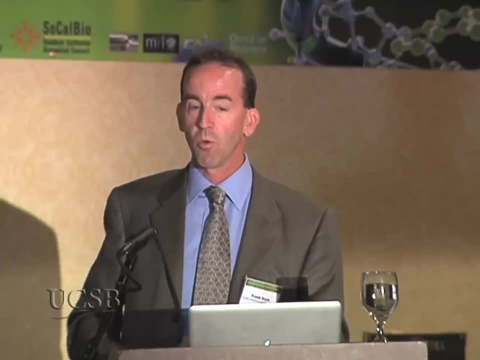 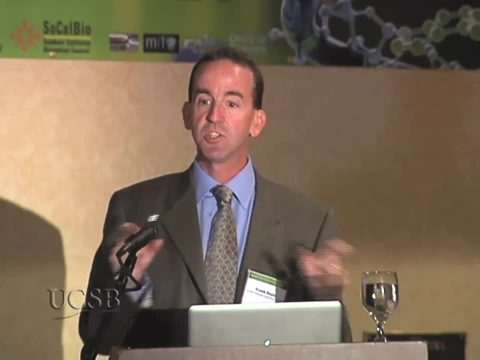 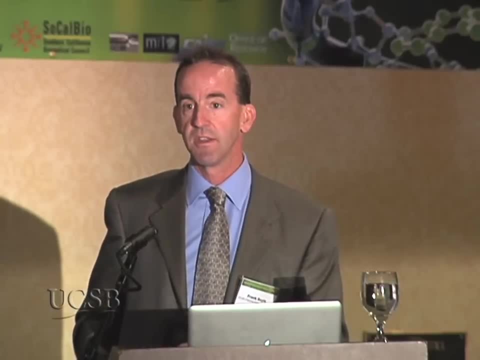 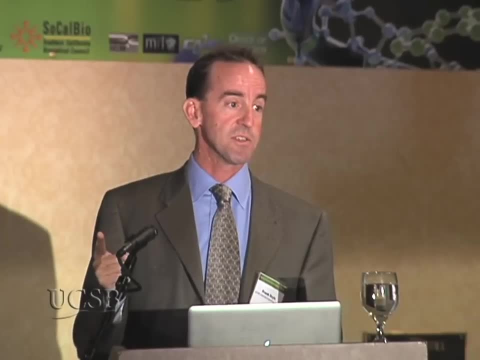 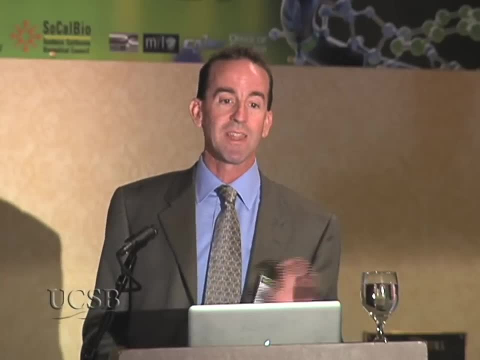 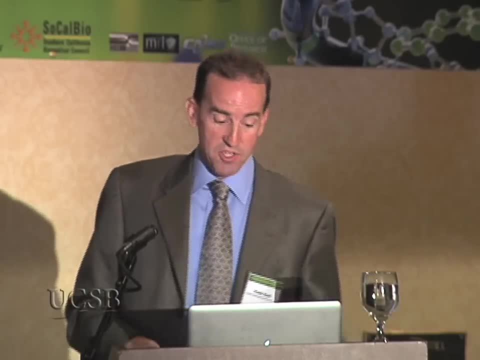 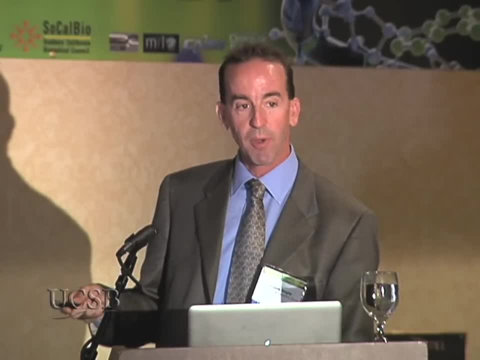 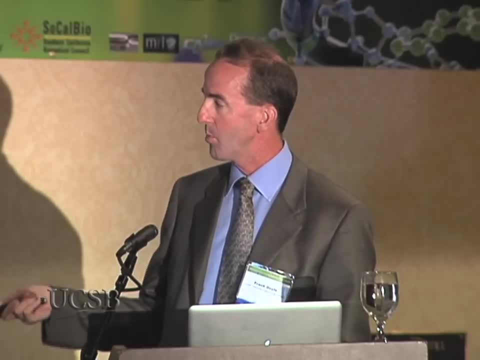 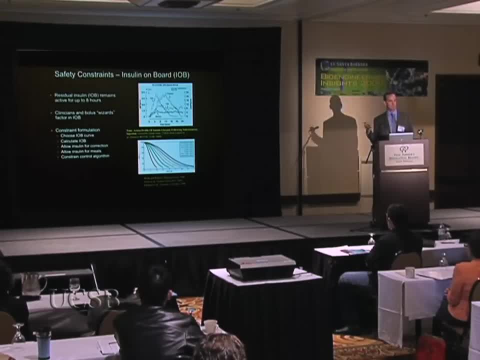 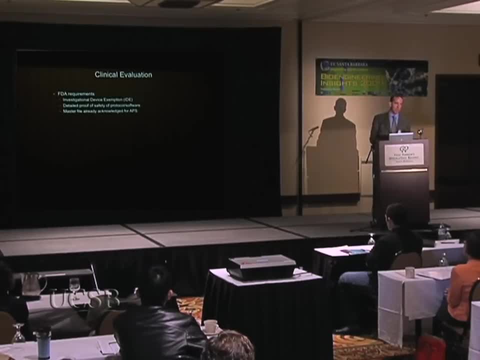 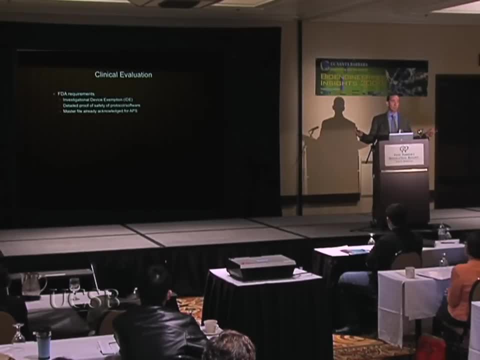 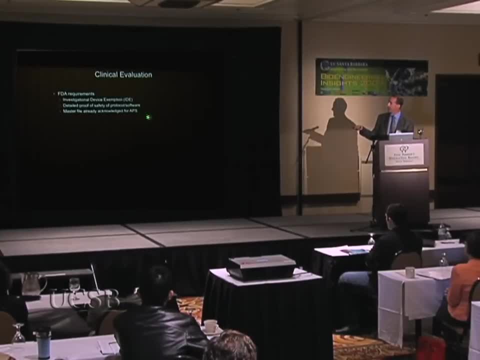 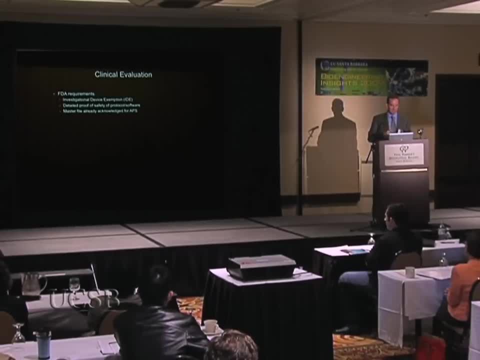 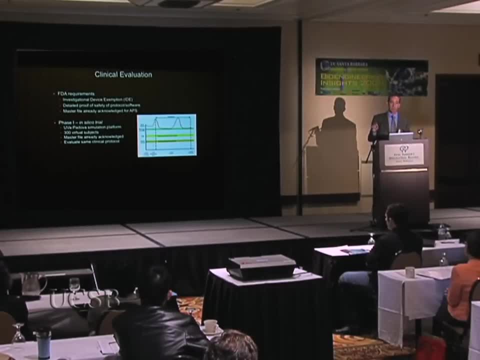 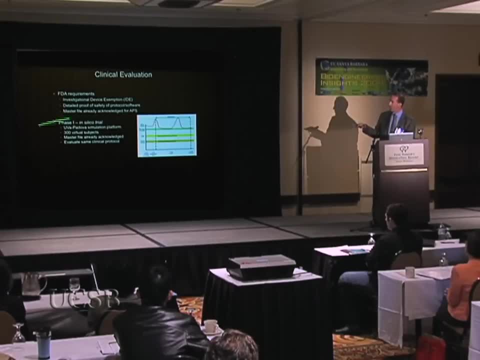 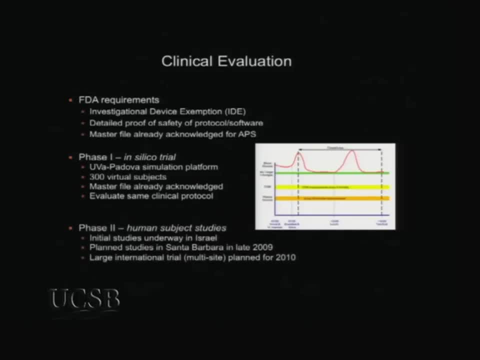 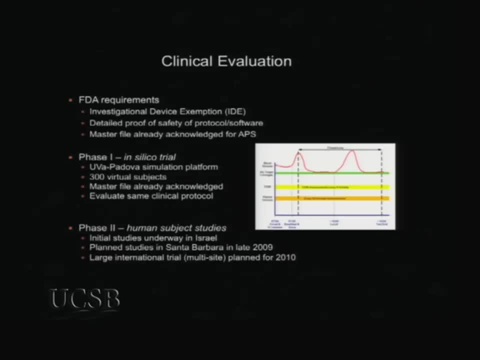 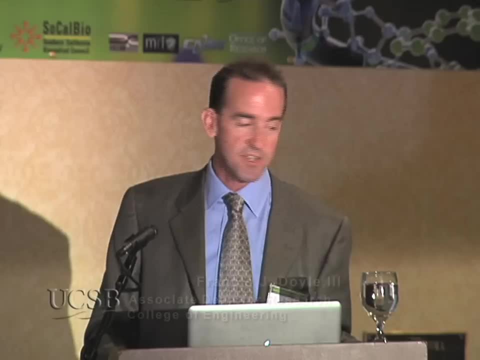 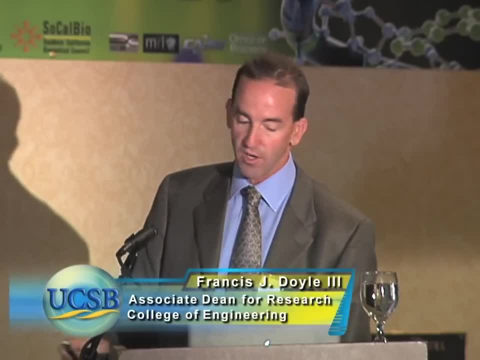 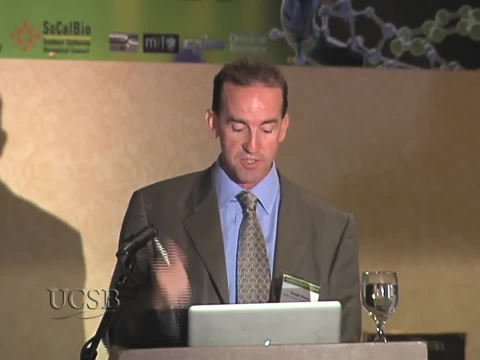 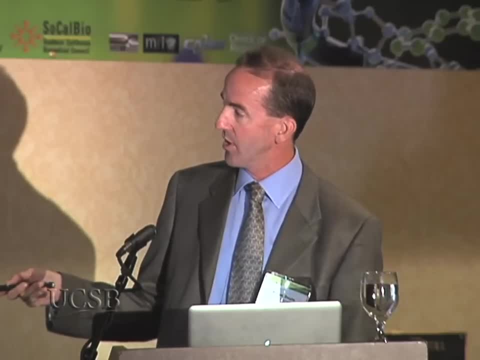 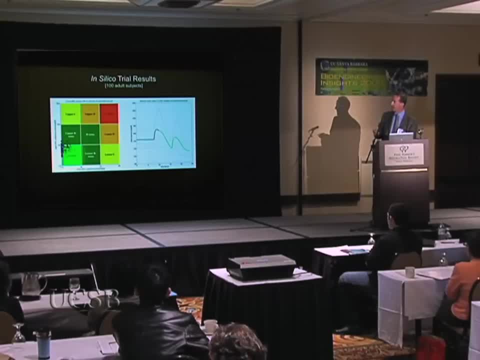 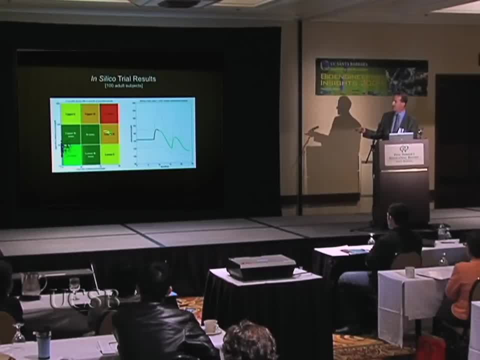 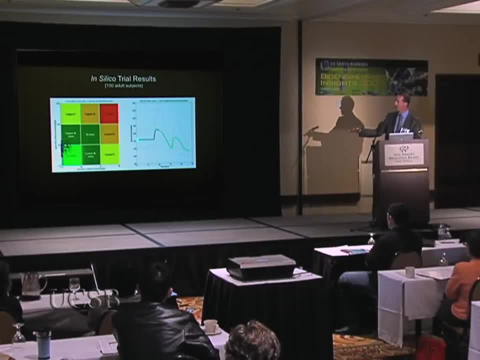 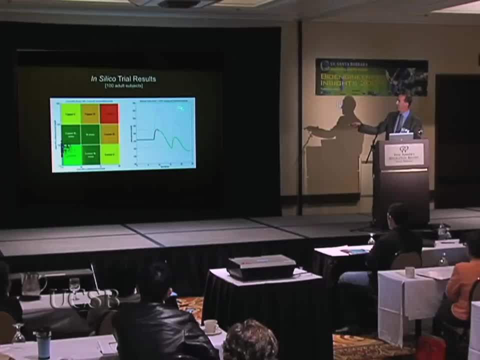 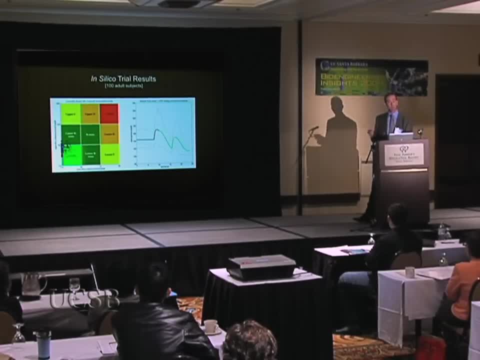 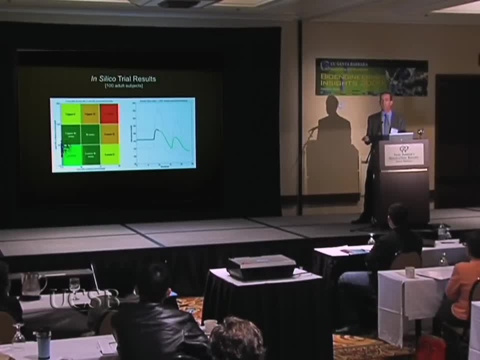 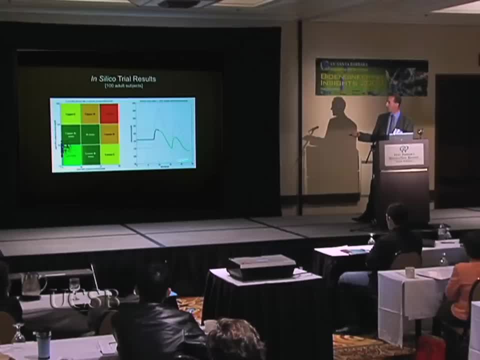 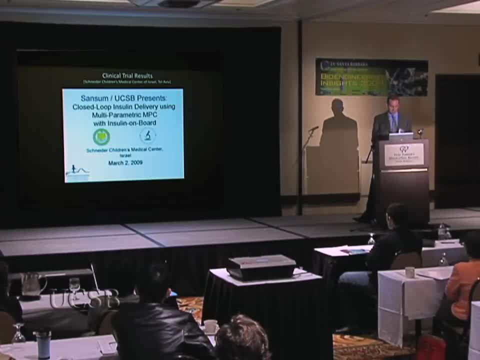 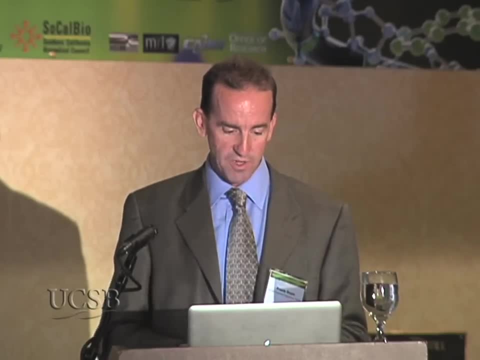 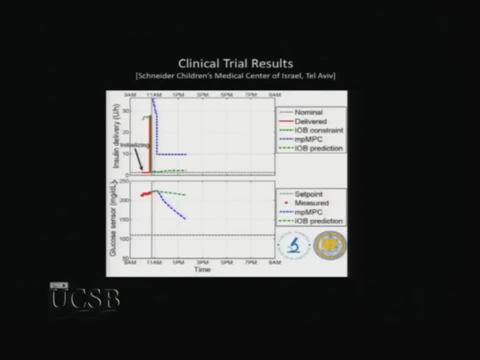 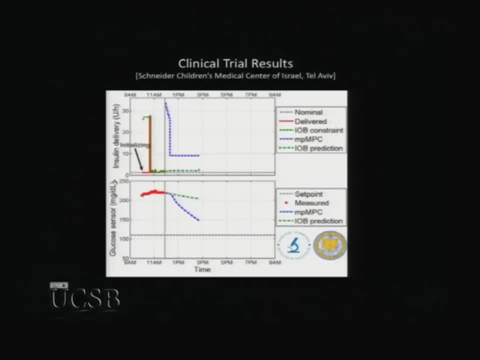 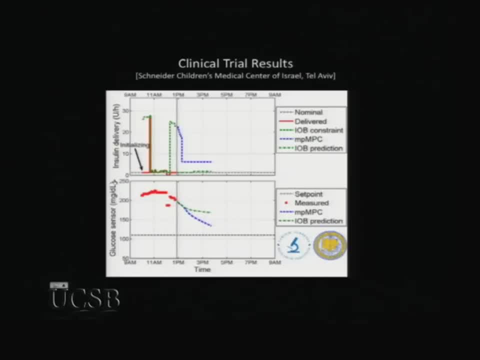 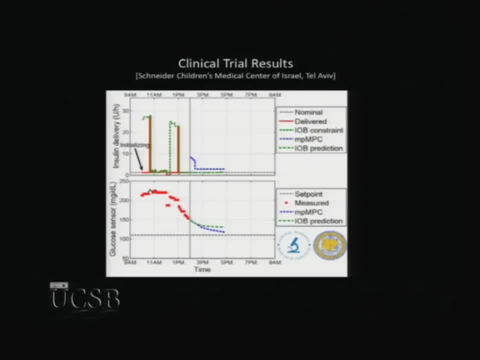 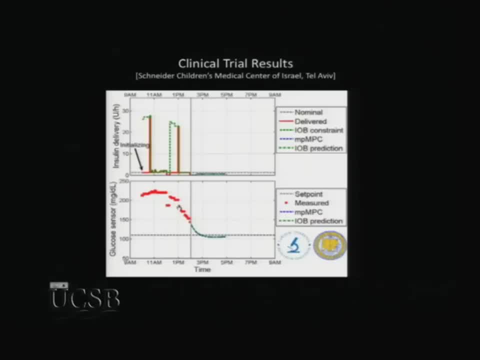 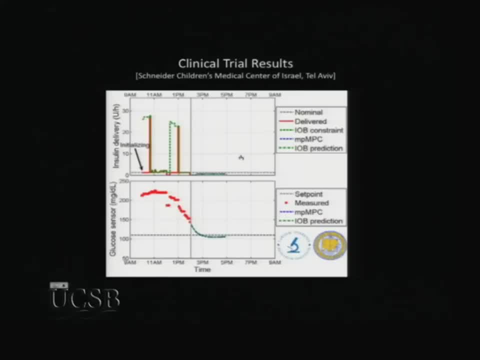 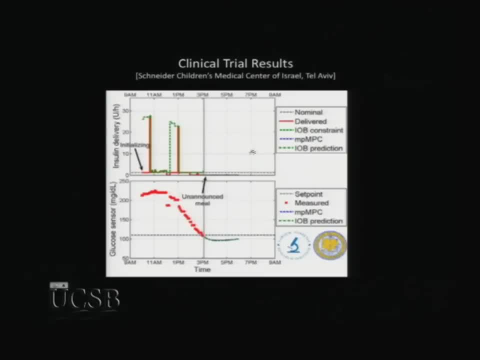 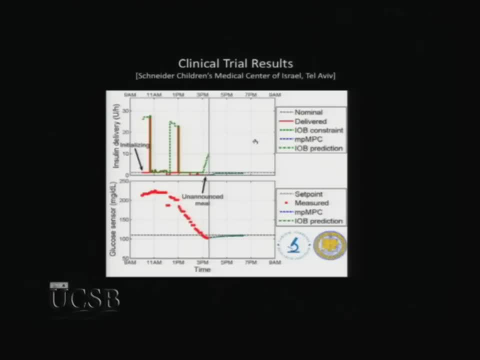 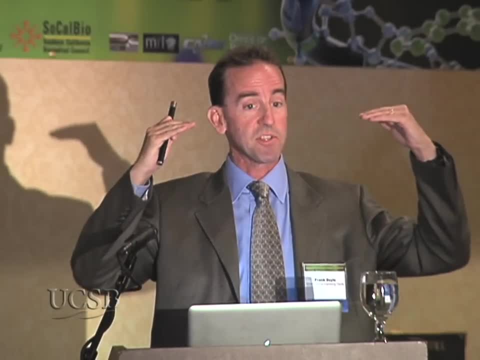 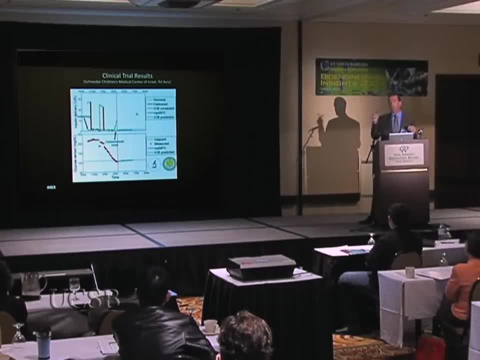 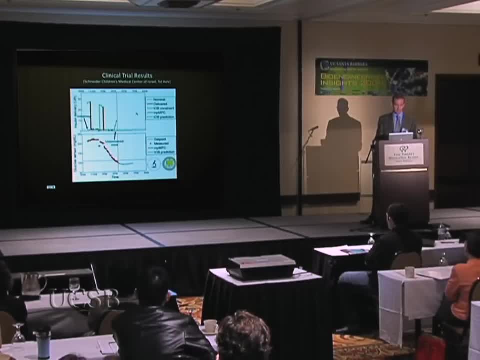 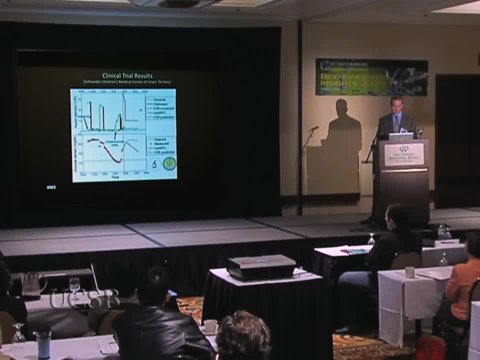 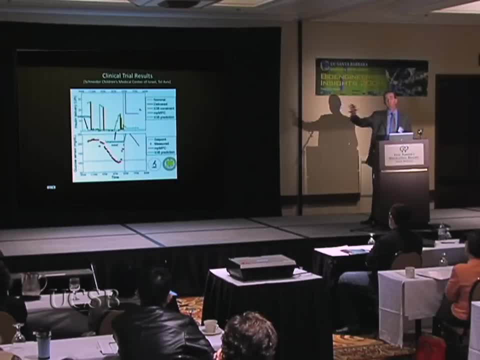 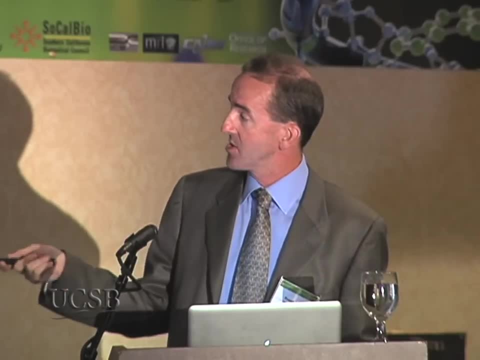 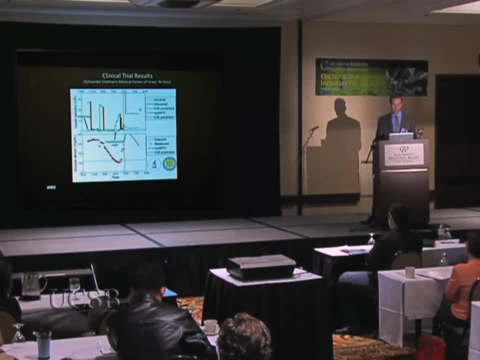 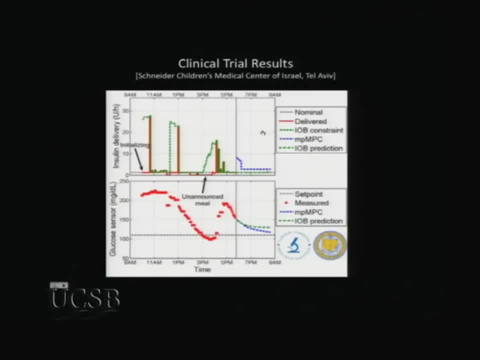 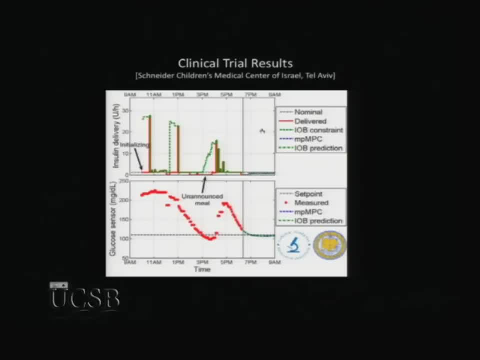 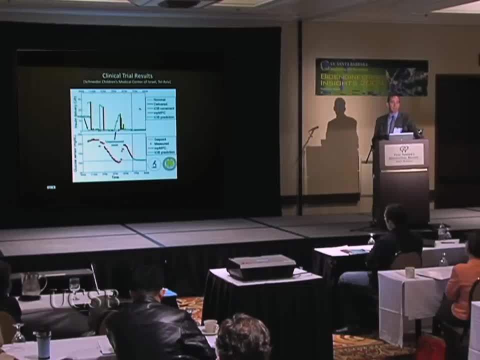 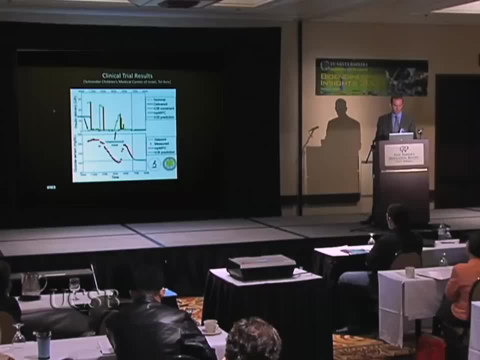 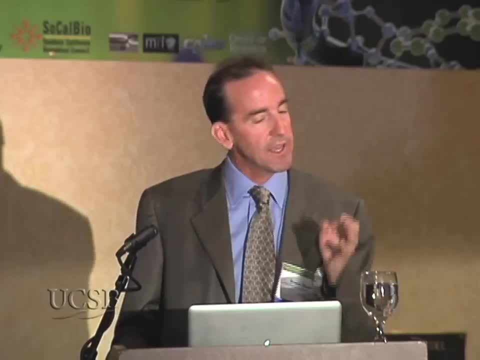 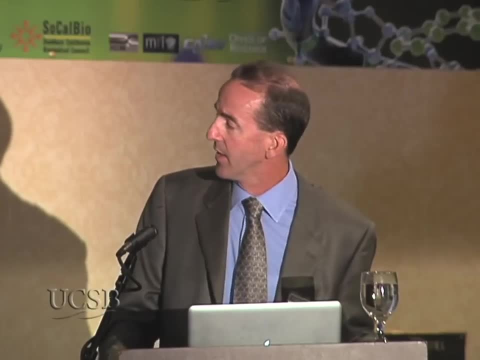 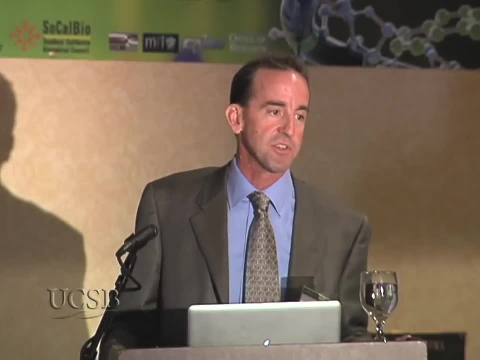 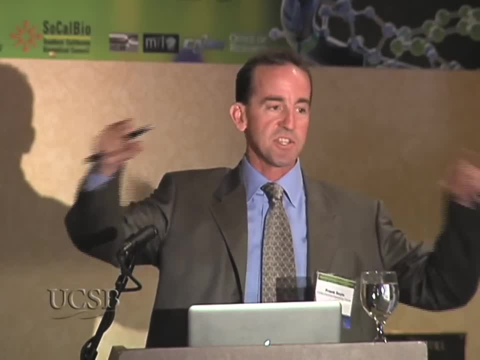 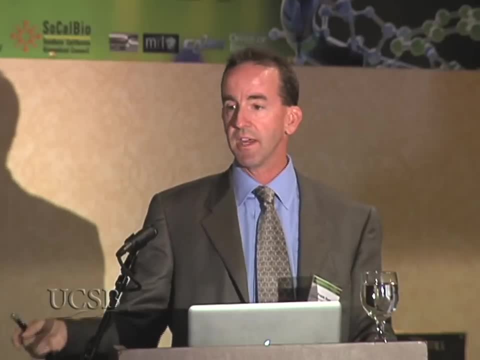 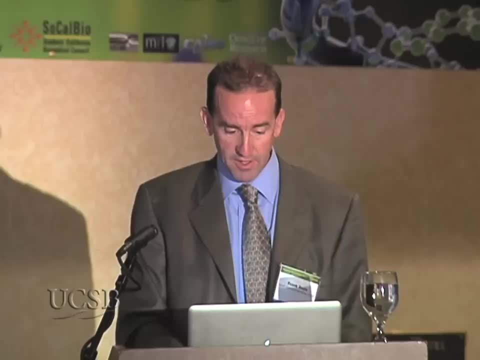 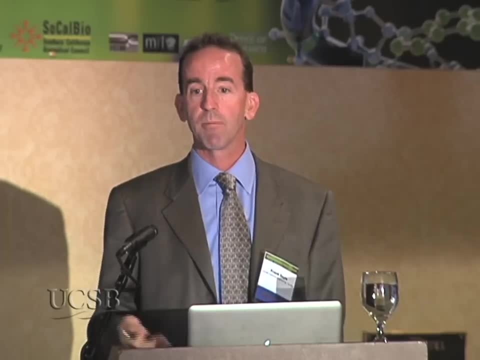 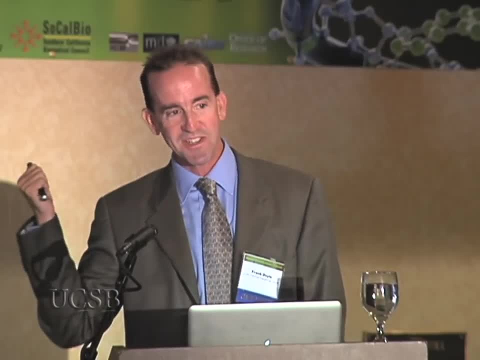 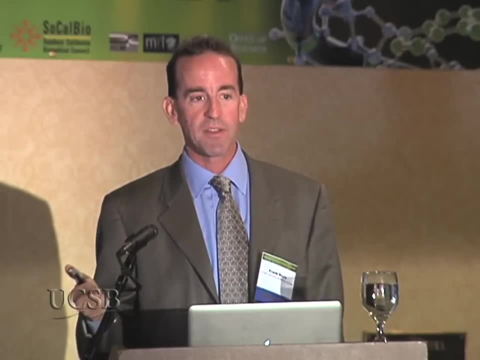 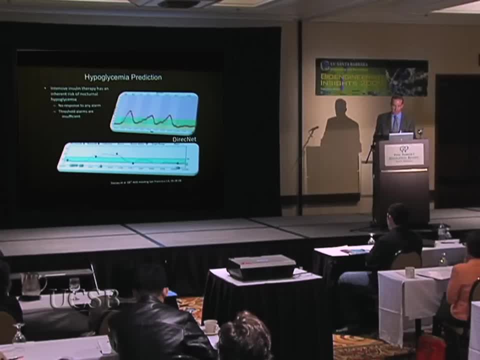 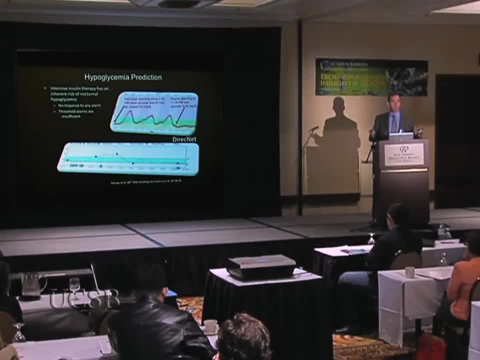 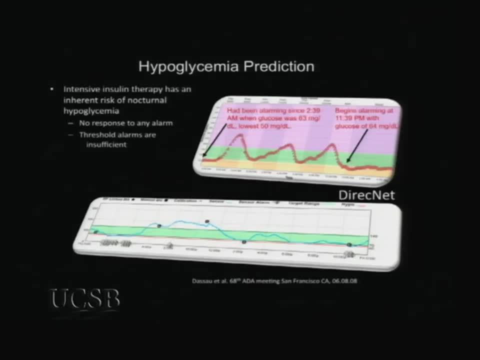 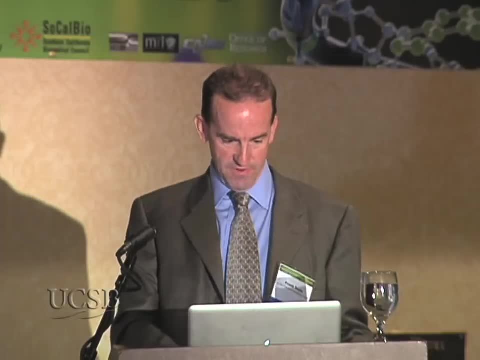 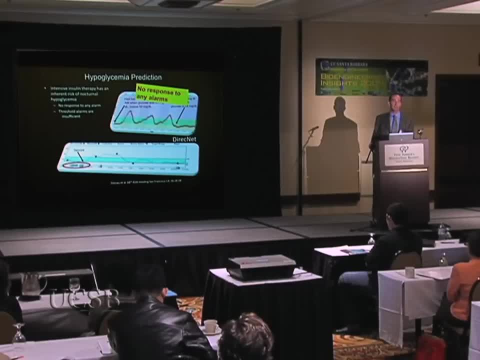 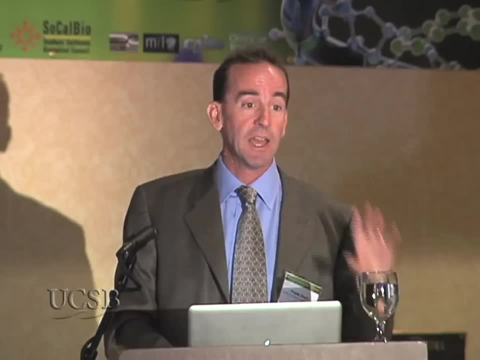 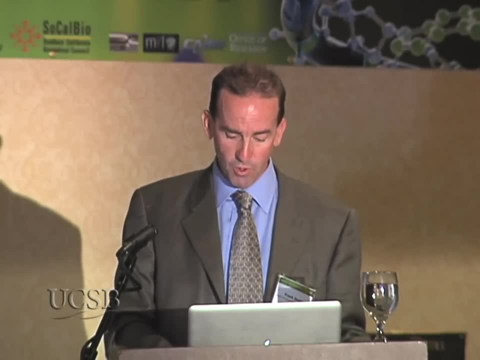 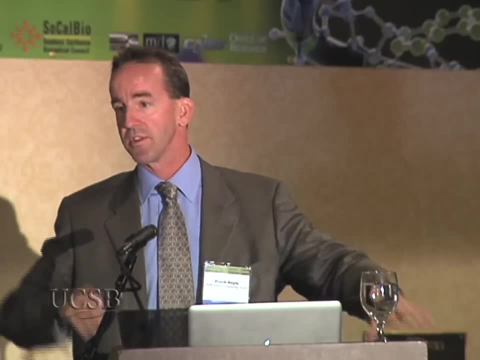 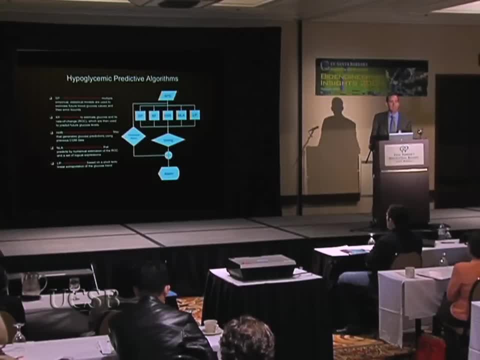 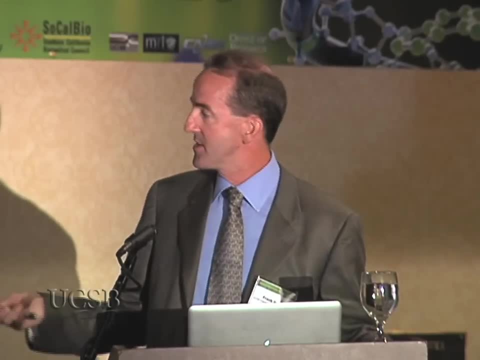 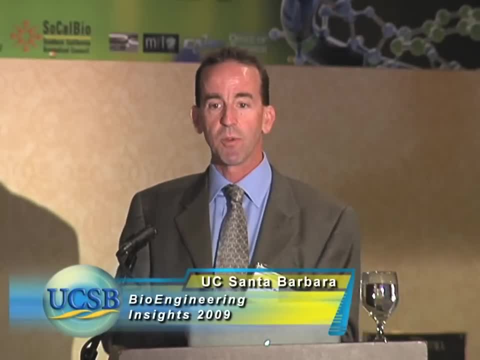 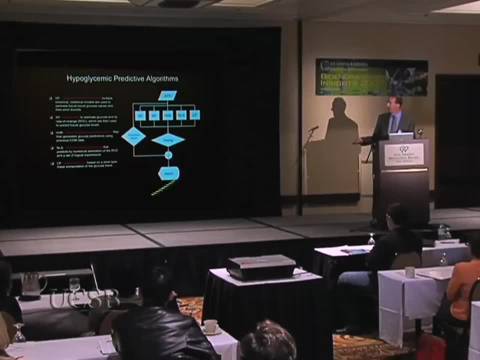 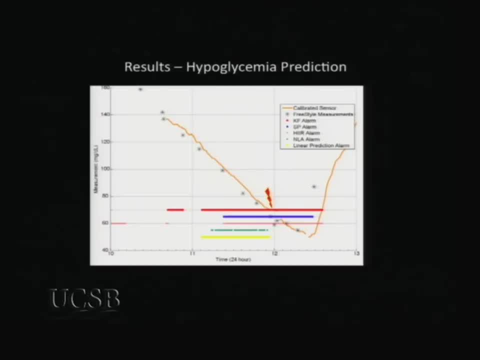 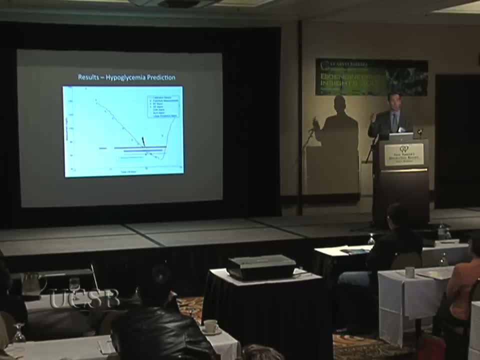 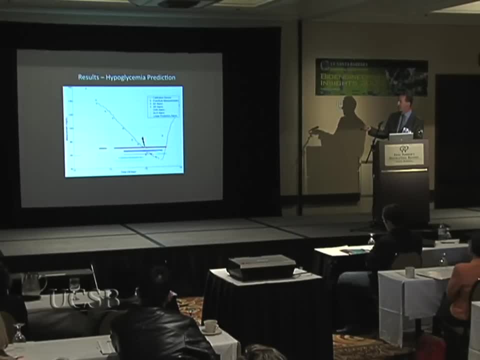 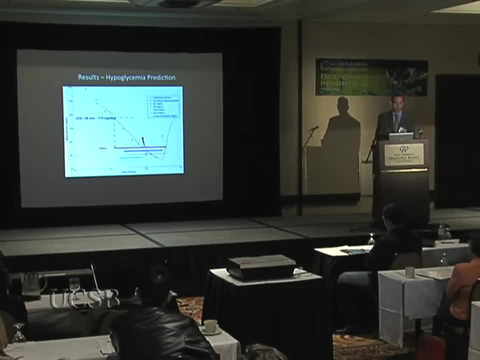 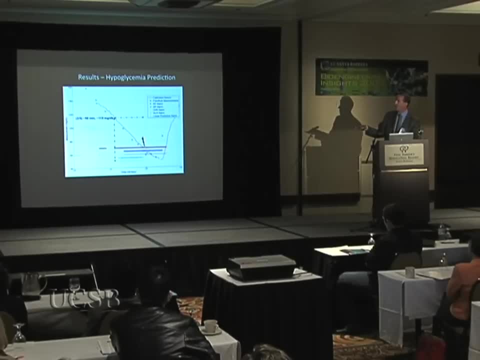 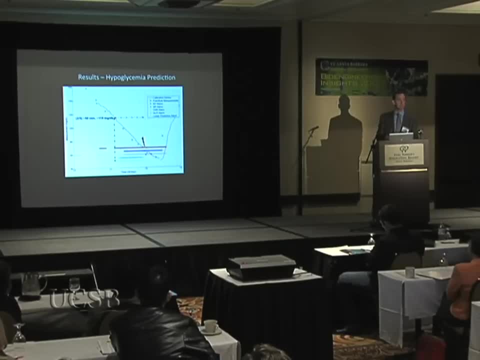 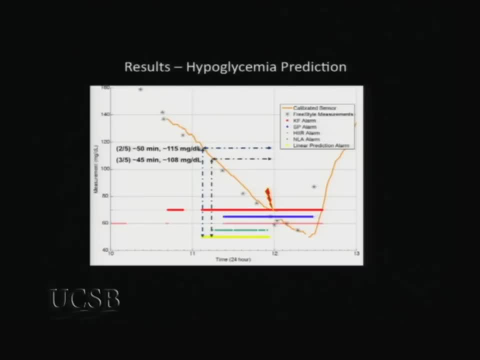 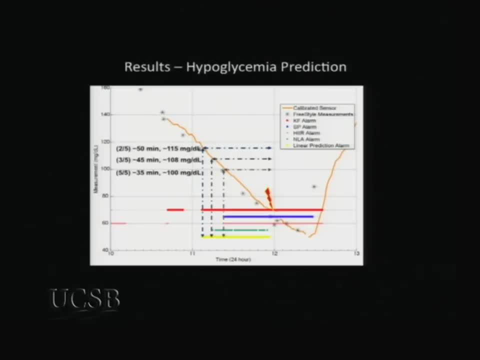 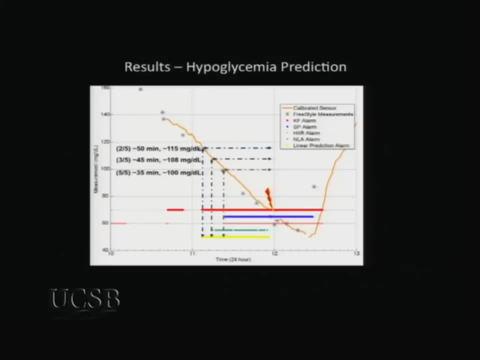 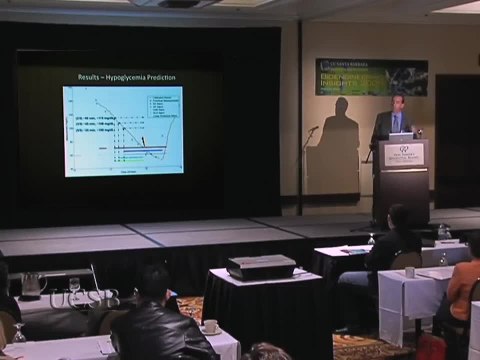 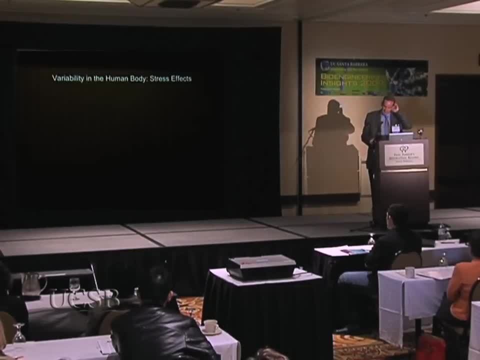 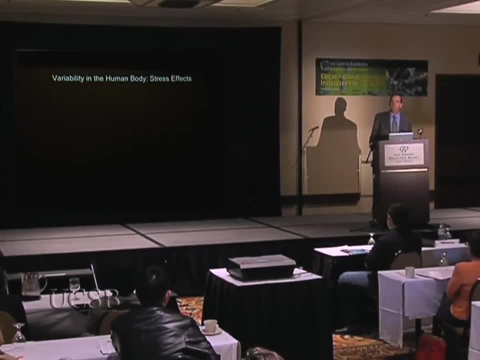 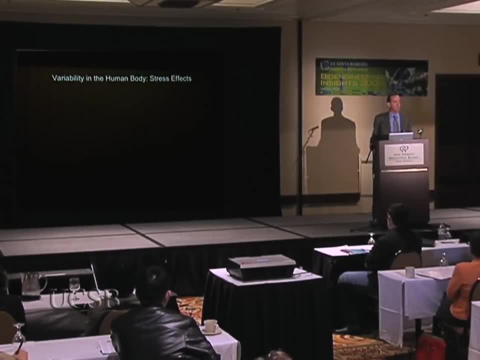 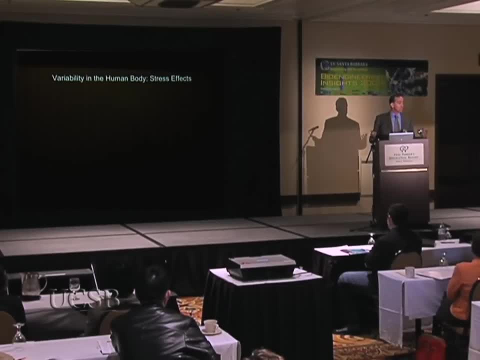 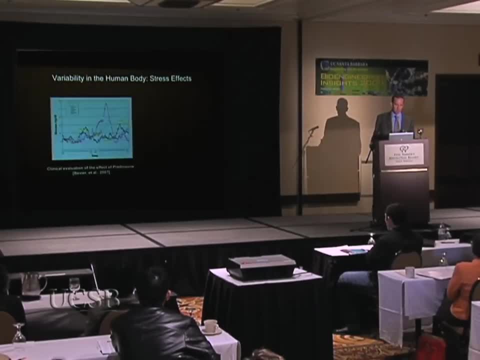 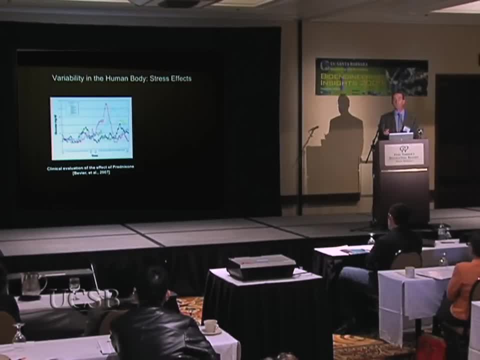 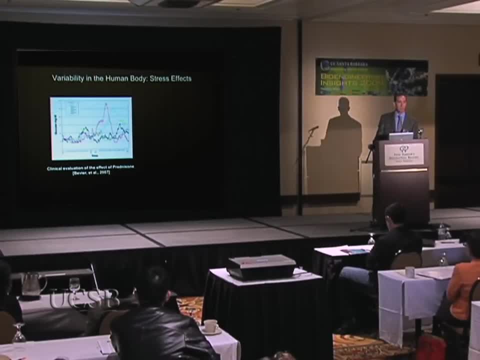 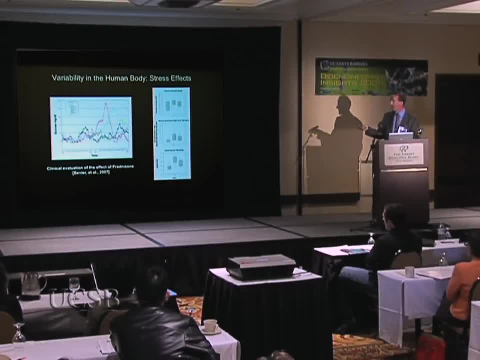 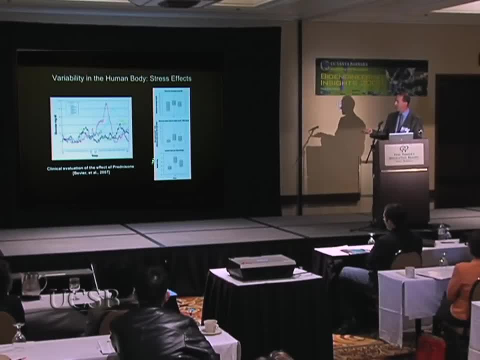 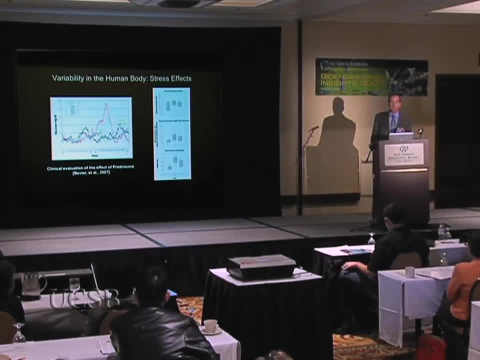 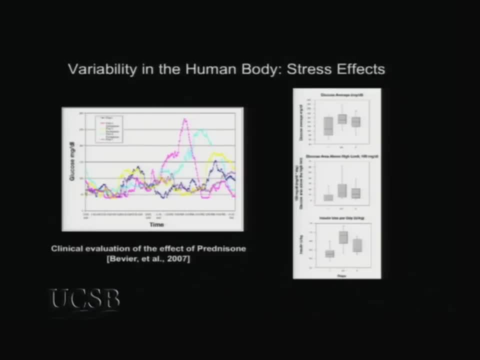 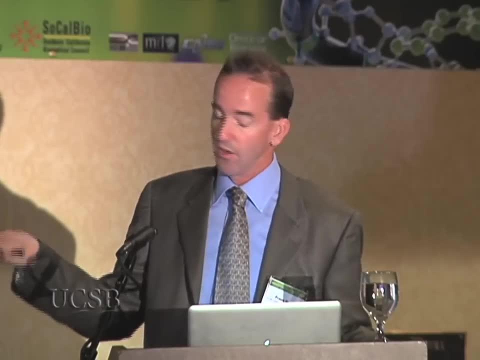 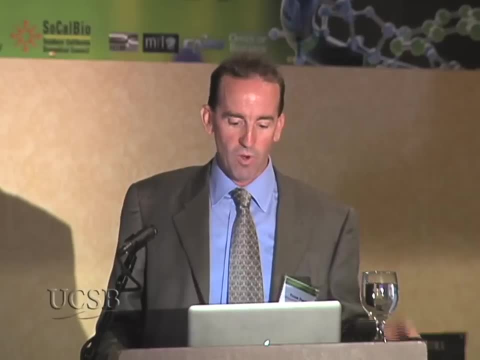 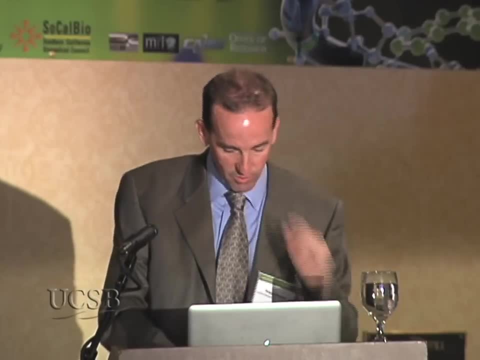 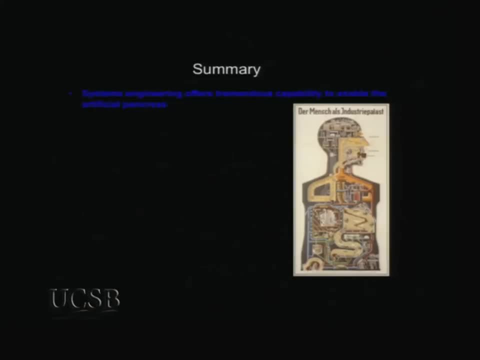 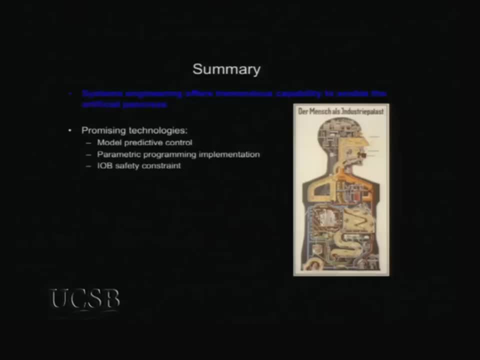 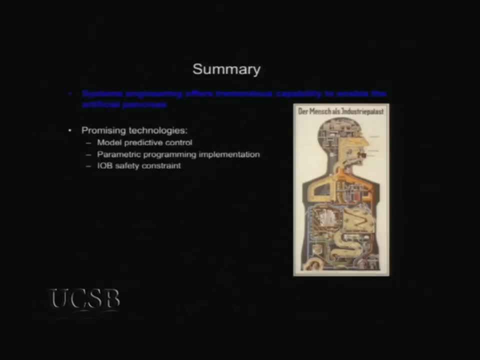 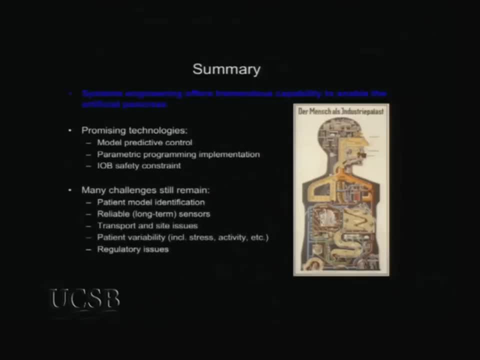 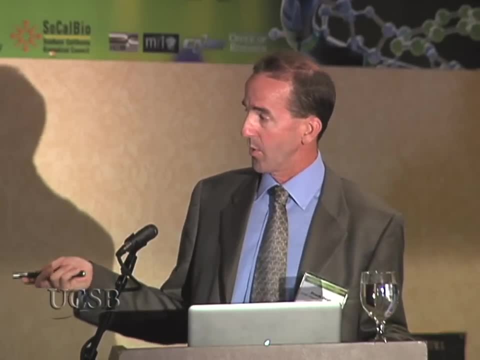 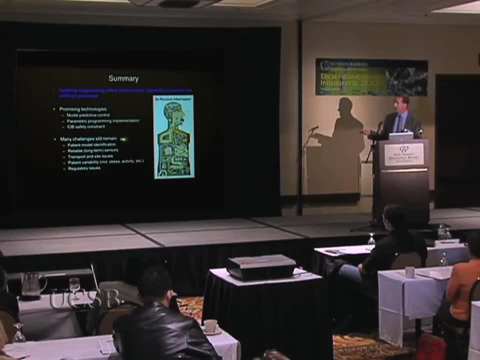 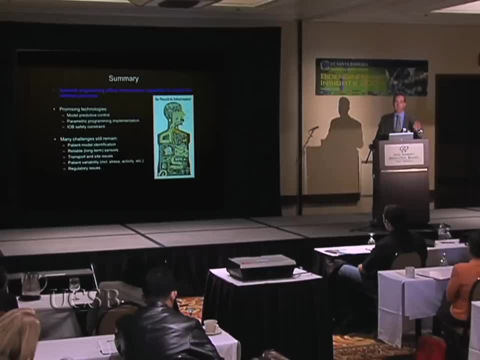 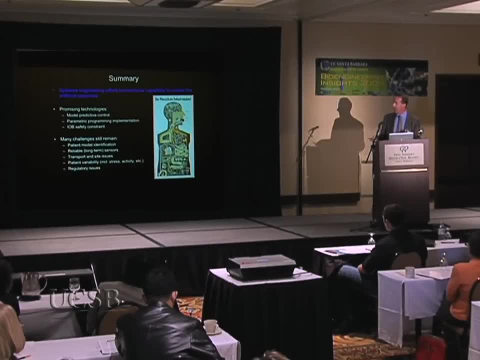 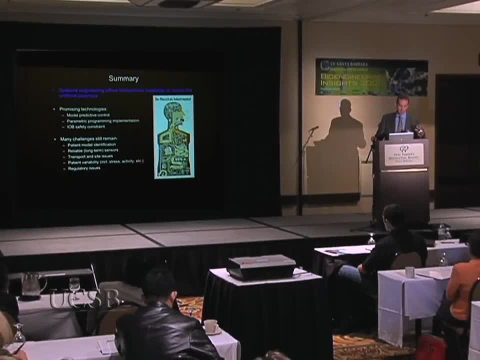 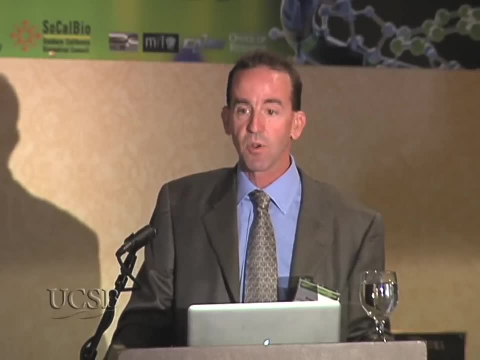